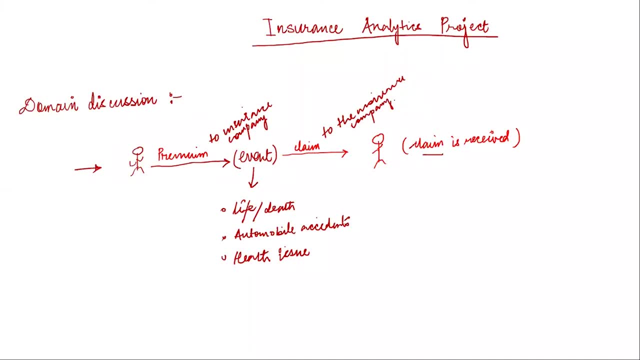 I'm going to first talk about insurance as a domain: insurance analytics. What happens, What do people do? What do data scientists normally do? What are the different kinds of project you can expect, And then try to contextualize this project so that whenever you want to think about it, 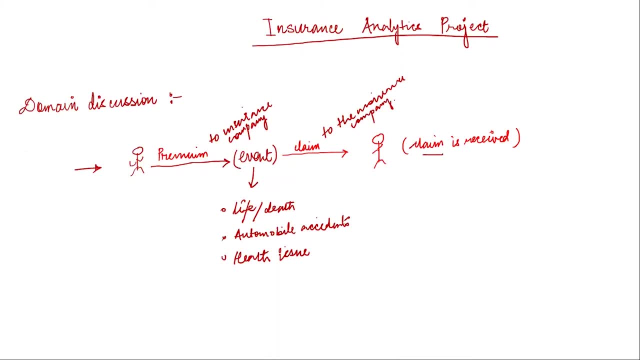 later on or you want to talk about it. you can put this entire project in the right perspective. So we'll start by doing a quick round of domain discussion. So what happens in insurance? I'm sure everybody knows what insurance actually is as a product, but let's have a look at 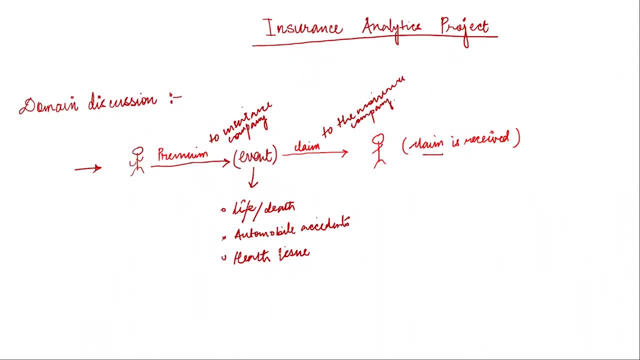 the basics first. So a customer comes along, customer decides to take an insurance product. What happens over here is that the customer is going to pay a premium to the insurance company and then this will continue whenever there is an event. So this event can be whatever. 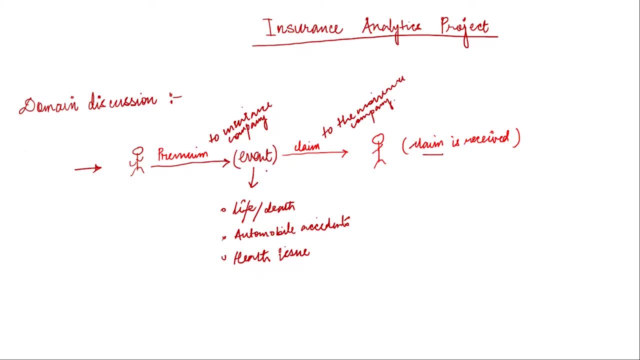 is the insurance insurance insurance is for, For example, if it's life insurance, if the individual dies, unfortunately, then the insurance company is supposed to pay back the promised sum of money to the nominee- No Okay- of the in insured individual. it could be for any other event, for example automobile. 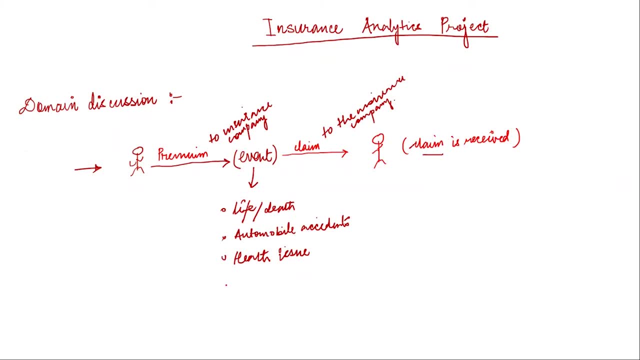 health issue: automobile accident, car accident. it can be even your uh. nowadays i've heard footballers are ensuring their various, you know, i think you know their legs. the specific um specific tools is for specific um different um you know uh profession that it can be. in short, 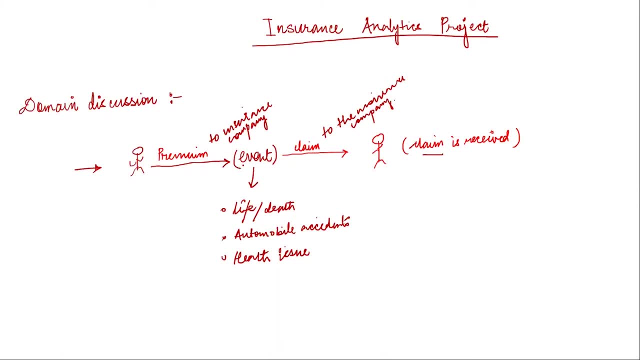 in the us, people typically insure their homes as well um their tv sets. you know whatever. most of it comes with insurance. even nowadays, ola has introduced something like a travel insurance to charge you a rupee something for it. irctc has been doing it for quite some time. so insurance- 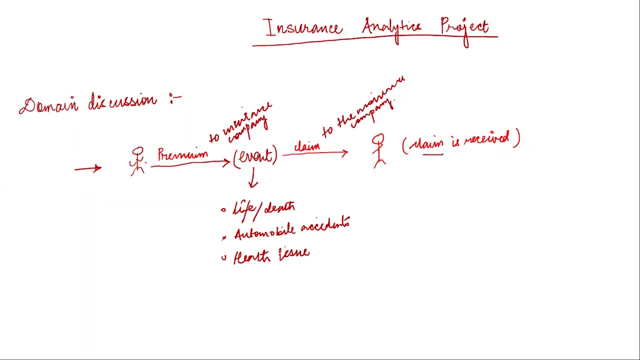 um is, the is basically the business of taking money from the insured individual or a group- in terms of, uh, in the form of premium, and then, when something goes- uh, the event actually happens, then a claim will be made and then, uh, the claim is going to go to the insurance company and the 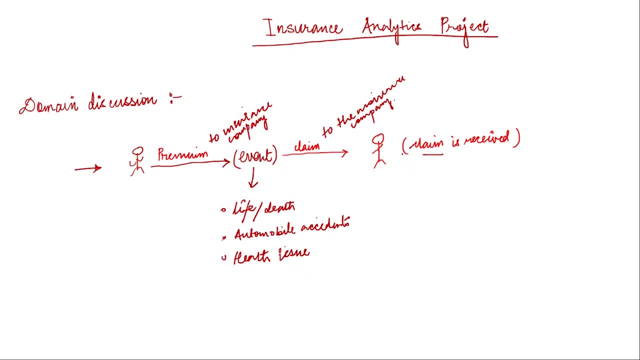 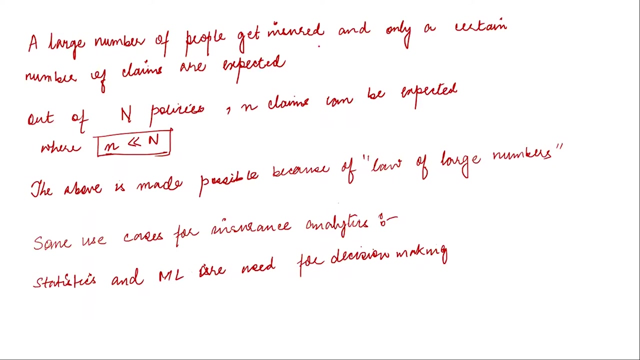 claim is, i mean received, of course, by the company, and then they will pay out, right? so insurance is the business of taking money from you and uh then paying out only when the event for which you're insured actually takes place. okay, so question is that? uh, we often find that you know. 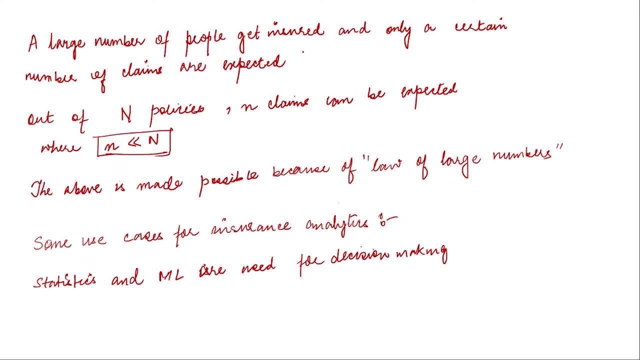 lot of people come and tell you, especially in policy bazaar- we find that ad from akshay kovar too many times that you know. just pay 500 rupees and get insured for one crore. um, do any of you, uh, have you ever given? 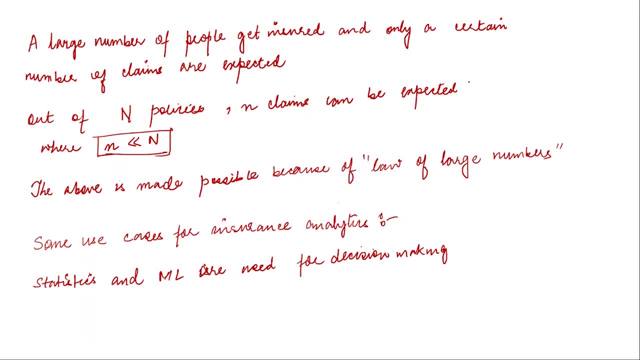 it a thought that how is it possible that i can? somebody takes a insurance policy of 500 bucks, pays for a few months and then, unfortunately, even if something happens, um, the individual can actually claim one crore rupees. so how does that work? so what happens is there's a mathematical 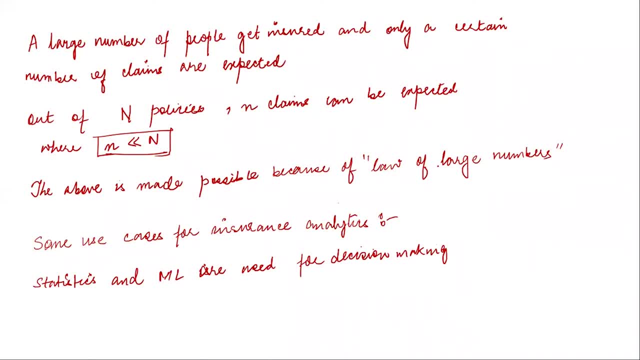 law that's in action in case of insurance domain. it's called the law of large numbers, this law. so what they do is they will ensure a large number of people and only a certain number of claims can be expected from them. okay, so out of capital n policies, small n claims can. 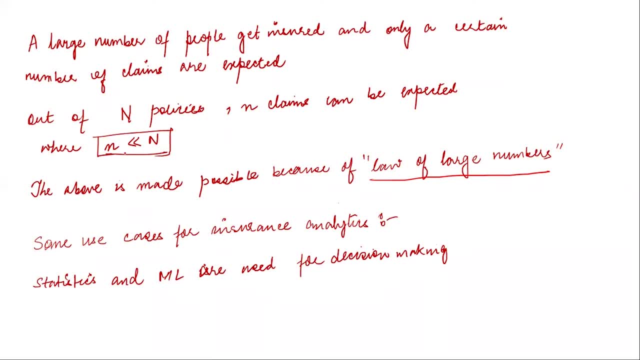 be expected, where small n is much, much smaller than capital n. so you're going to basically say that, although there is a- uh, this is a aspect of people that you know- people can actually claim and get their money, but insurance companies spend a lot of time doing analytics on how many people 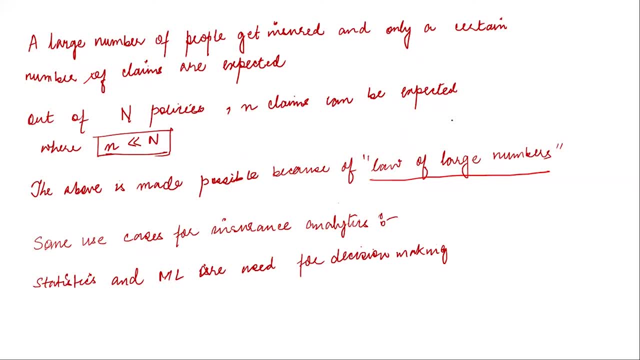 are going to claim, if somebody is going to claim at all, and those kind of things. so these are some of the questions that they will ask. okay, so some use cases, if you look at it, and they- this is one industry that heavily uses statistics and other very, very heavily. uh, you know, insurance in in. 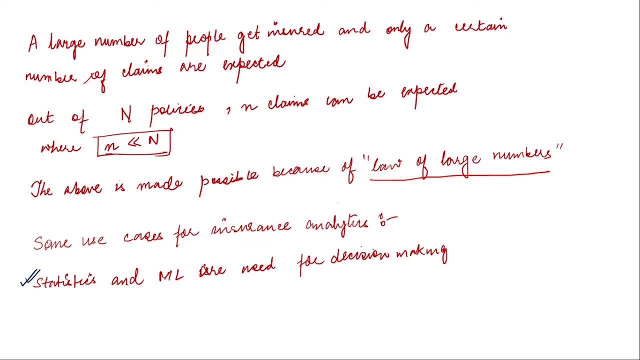 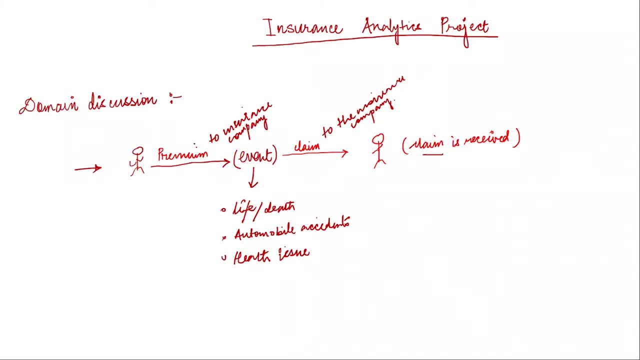 this will use it primarily because they're always trying to figure out that what is the right price to charge you. so if you look at what is happening here, if you're insuring something, there's a certain premium, uh, attached to it. right, you have to pay some money. the question is insurance. 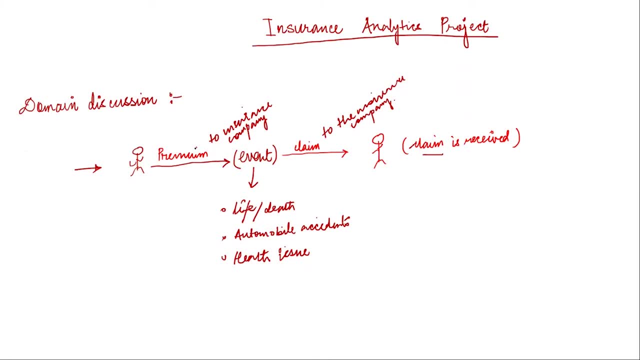 companies use a lot of math, a lot of stats to actually determine the right premium to charge for an individual customer or for a group of customers, whoever is getting insured right, so that the risk of paying back the money is covered. so when you think about risk, right? let me just add: 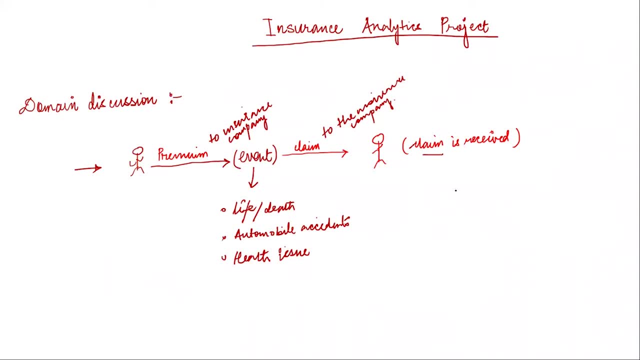 a note here: the difference between banking and insurance. so in case of, say, risk, right in banking, the risk is when people don't pay back the money, when customers do not pay that. so in this case, where the customer do not pay back, in this case customer expects a payback is right. so it's a very 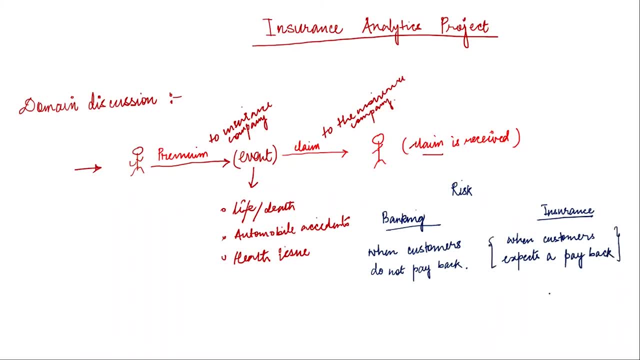 can you think about like it's hugely profitable. so one of the major private players in the economic india for insurance is sbi, life and html. i don't know if you guys uh get a chance to think about investment, but you should definitely have, uh you know, some of your investments in that domain. 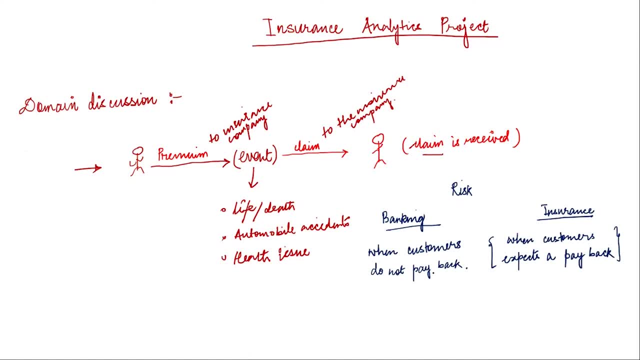 it's massively profitable because there's only a certain amount of money that ultimately will be paid back. otherwise all the money is practically free money for the company. so if uh like, for example, i mean i have taken a term insurance right, um, in my policy, if i'm alive, 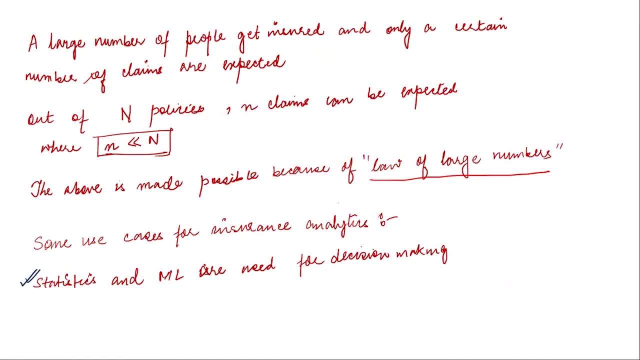 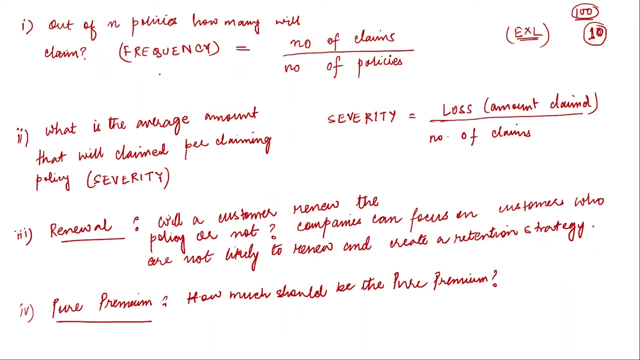 after 75 it is a total loss. i better be dead before 75 for my family to get the money. you see, you see the uh challenge here. so it's hugely profitable uh for the insurance company as a whole. okay, so now we're going to talk about certain basic terms. i want you to learn frequency. 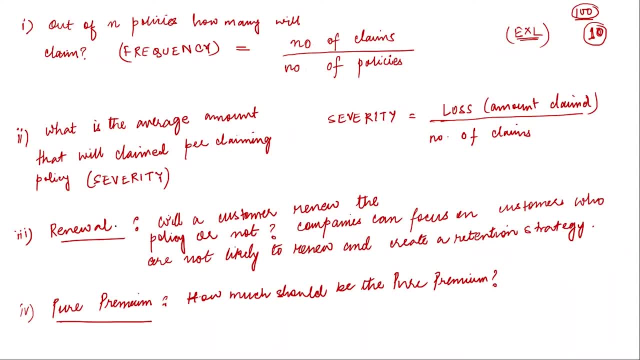 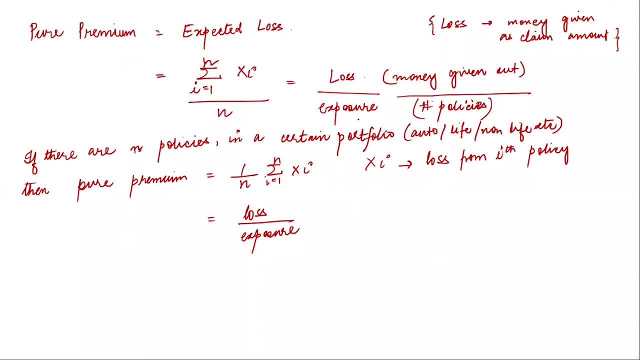 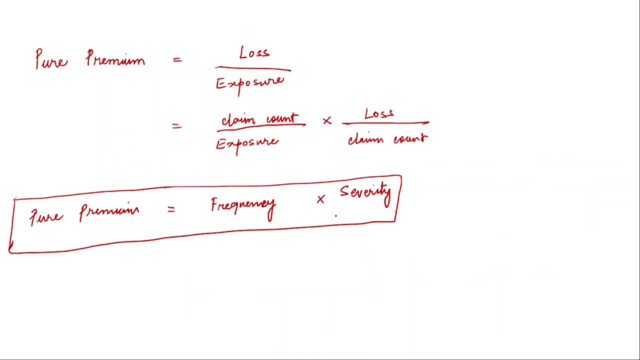 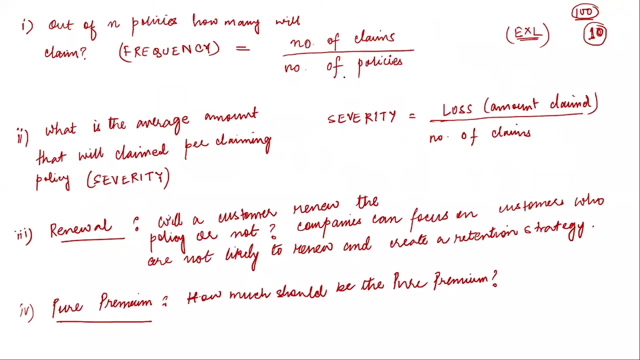 and severity, uh, are the two fundamental terms. then we'll talk about pure premium. we'll discuss what is renewal, uh, what is pure premium, what is loss, exposures, etc. and then, finally, the uh relationship of pure premium with frequency and severity. okay, so what is frequency? frequency is that, out of so many policies that you have, how many policies? 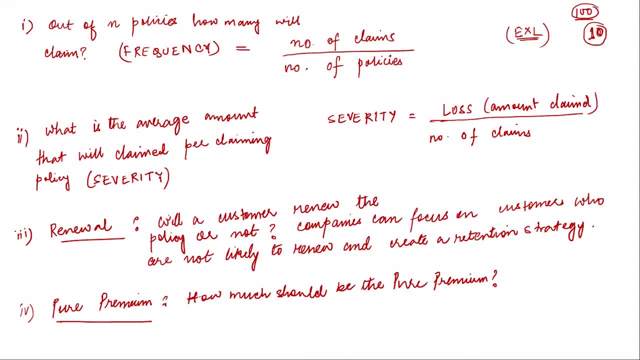 will result in a claim, or how many claims will take. this total number of claims divided by number of policies, that's the frequency of claim. okay, i am putting a question across to all of you. just think about it, don't answer, we'll get to it when we get to it. if you want to, uh, build a model to, 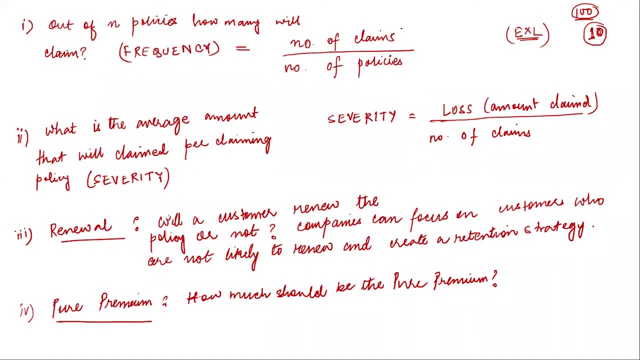 predict number of claims. uh, what regression technique will you apply? don't answer, but just keep this with you as a question. okay, think about it, we'll, we'll get to it. when we get to it, we'll come to it and we'll discuss it later. um, now, now comes severity. severity is that whenever 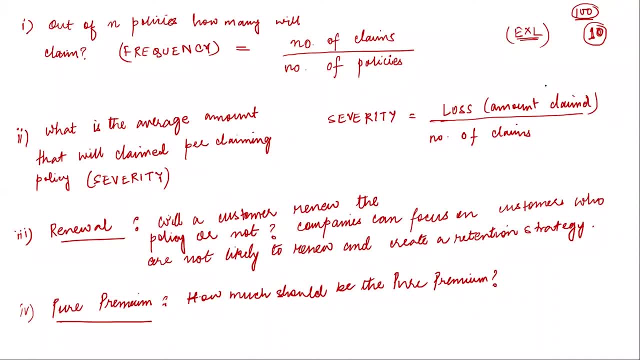 there are claims, right, how much money will be claimed? for example, um, if i do a car insurance and i insure my car for, say, three lakh rupees, right? um, if i claim total three lakh rupees, then i have to show that my car is completely smashed. it's a completely like total loss out of three. 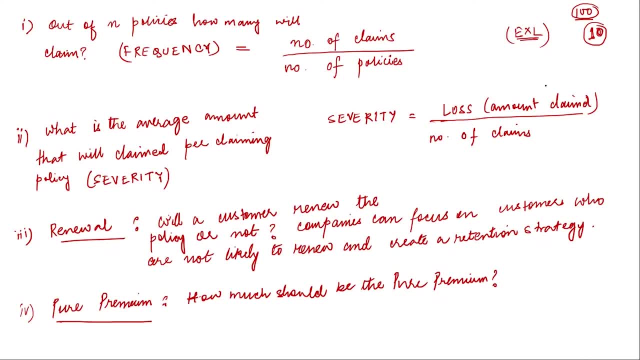 lakh. how much money am i going to claim? so what is uh going to be the extent of my claims that i am going to claim it is considered tea. how much does it cost if i am in the auto service? i can essentially give you an average amount of total amount of money out of total number. 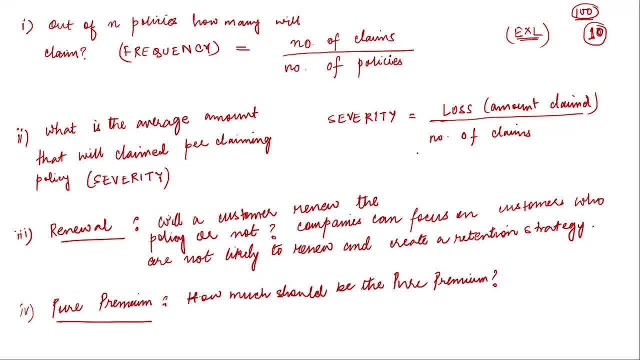 of decisions out of taking animal Labor and how much are you claiming? so? how can you apply out of total number of claims, that's the area where they claim the most, because number of preference. so the Scottish index, it's not the date, it's not the Ecological year, the for their 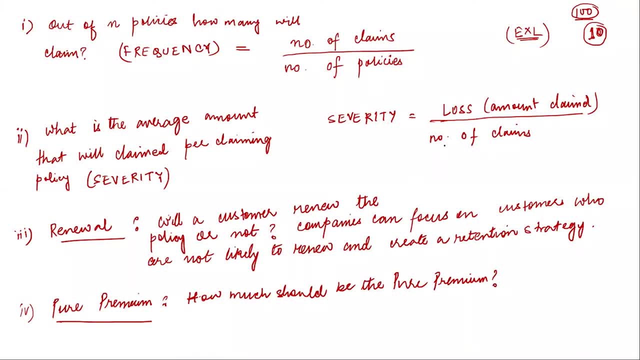 ild question: right, right, what's the average amount to claim? 100 people, right? what is your number of claims? so under that? not that mean you're over retirement, of that point it will only be. and for a total, if you take all the claimed amount, that comes to x. so x divided by 100. 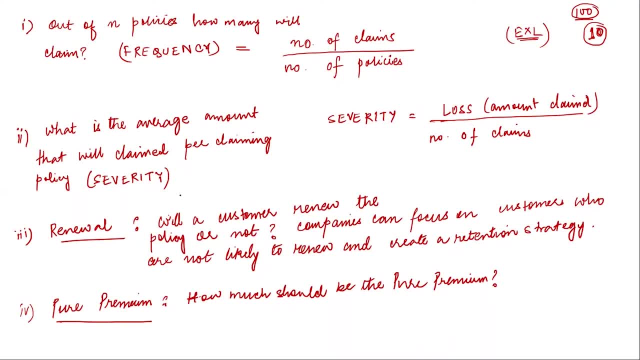 will give you the severity. okay, now comes a renewal. renewal essentially is the uh question that: will the customer renew the policy or not? now some, some people, some companies can focus on customers who do not likely to renew and then create a return strategy essentially, um, you know, 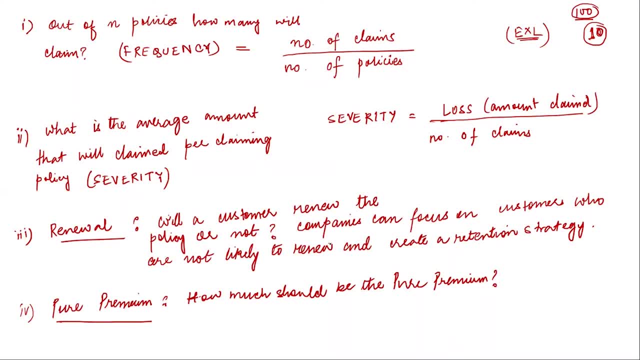 you want to figure out who's likely to renew and who is not likely to renew and you can go and create a strategy for getting more and more renewals right. okay, so there are projects, or machine learning project, associated with every single thing, on frequency, on severity, so there is. 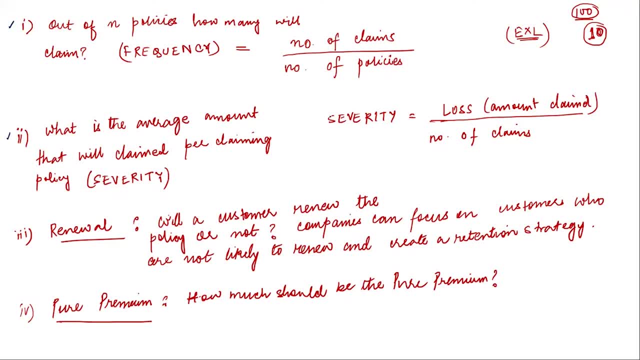 a. there is a. you know there will be model modeling on machine learning activity done on severity also also. or you will have to do prediction on frequency also, not on this project, but anybody working in insurance will be expected to do frequency modeling. severity modeling- uh renewal is the uh is a dichotomous situation where a customer is going to renew or not. that 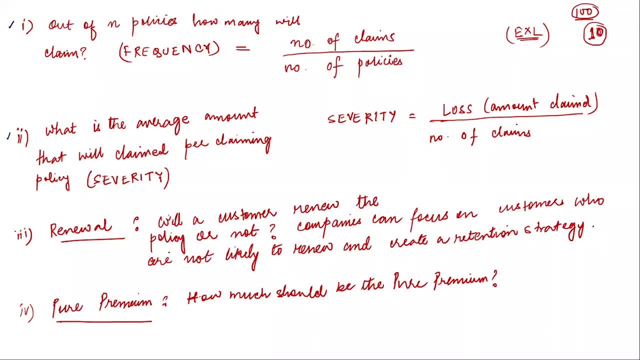 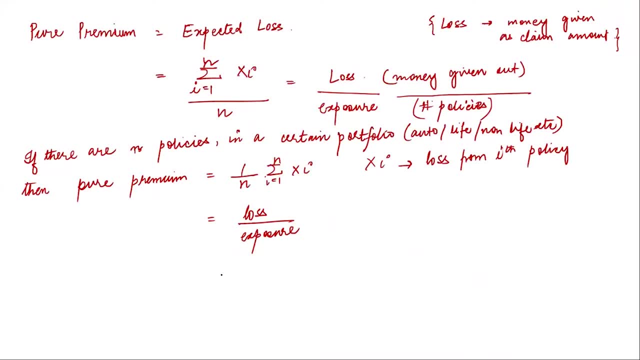 is basically the classification um problem treatment. now comes pure premium. how much should be the pure premium? that's a question that uh insurance companies have. so if you look at a pure premium, that is defined as expected loss or expected money, that is given out okay. so if you 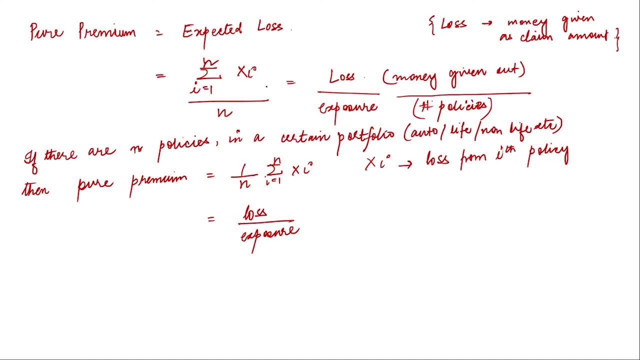 take uh the money from the money paid out in one single claim, right, or if if you sum it up across n different claims, so then you get the total loss or the total money that is given out and you divide this by the- uh, you know- exposure actually so number of policies that you have. so if you have 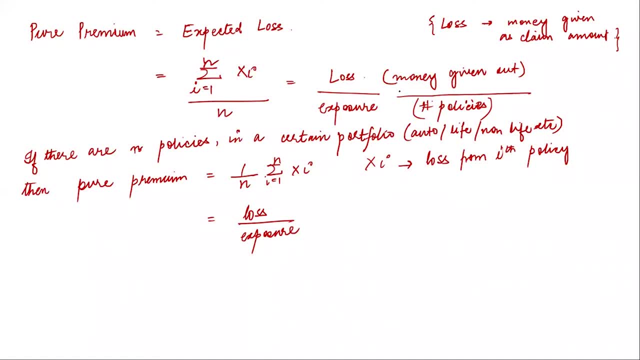 uh, one million policies, potentially one million people can come to you to make a claim. right, that is the total exposure of the insurance company and then in the numerator you have got the total money that went out. okay, so that is the. that's basically the pure premium. so, if there are, 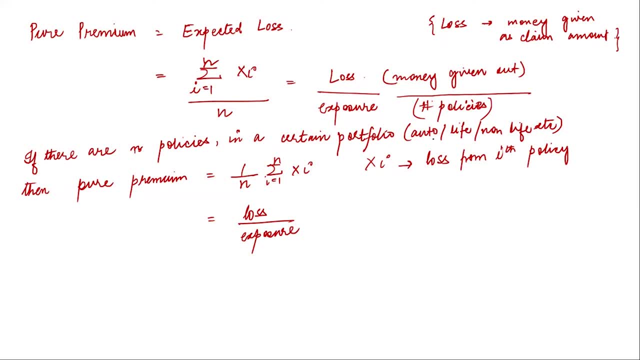 smaller policies in a certain portfolio. uh, it can be any: auto life, non-life, etc. then pure premium is basically one by n. summation of x- i, where xi is the loss from the is policy. no questions, uh, so yeah, so is this a pnc insurance we are talking about? right, any kind of insurance, any, yeah, plc. 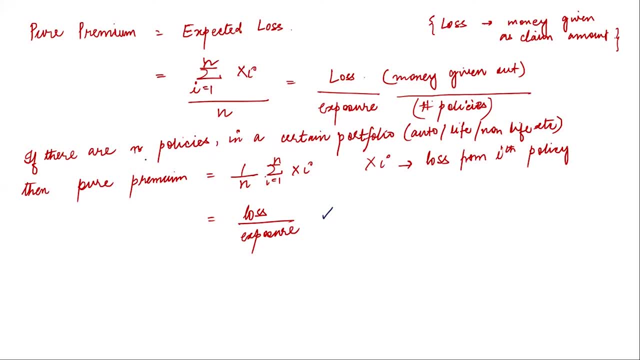 or any. i mean basically, um, you have n number of policies right out, of which some policies have resulted in a claim. okay, so what you do? you take all of those claim amounts, you sum up some of the total money that has gone out of your pocket to pay back the claimants. 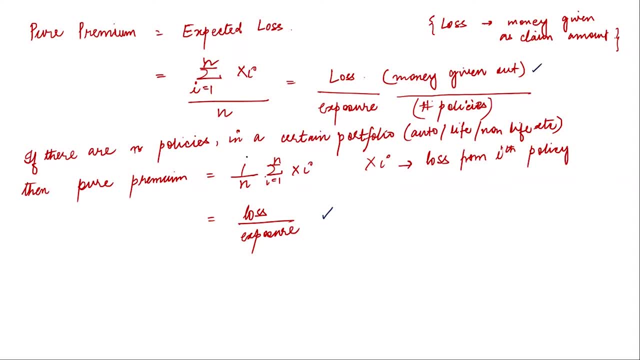 okay, and you divide that by the number of policies, that is basically the premium. so so think about it like this, right? so today you decide to start insuring people too, so that, uh, you know you can, you want to start an insurance business actually, so you start insuring for cars. 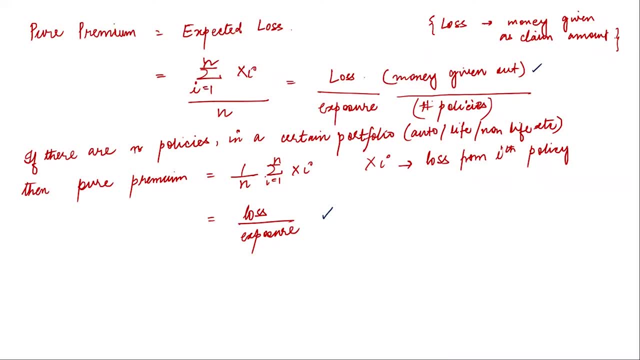 all right, and you start insuring for cars. and you start insuring for cars, and you start insuring for cars and you said, okay, i want to insure 100 people. fine, so you want to ensure 100 people? uh, what should be the policy? rip your premium that you want to, uh, that you want to like. basically, how? 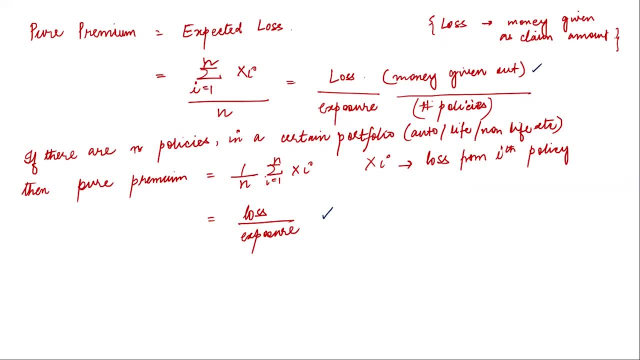 much premium do you want to? like you know minimum premium that you want to charge. so how do you want to get to that? you want to figure out: uh, your premium that you want to charge should cover for all the claims that will come to you, yes or no? you need to meet the customer expectations, right? 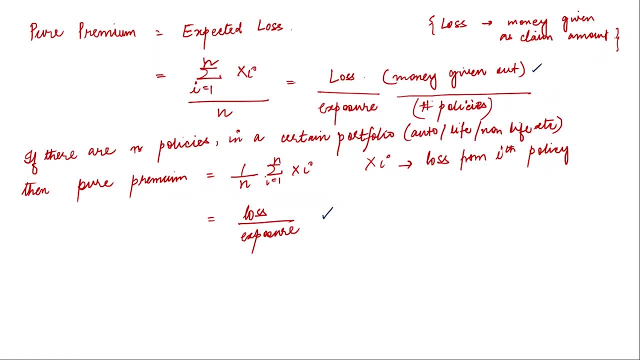 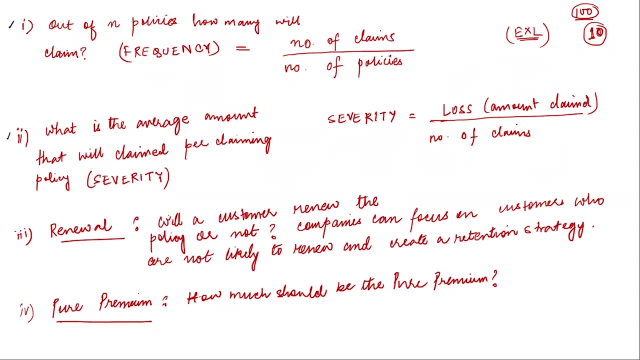 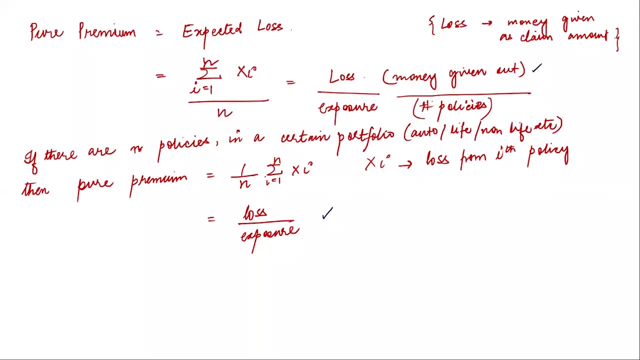 yes, right. so out of 100, say that. uh, by doing machine learning predictions etc. you figure out that you are likely to have not more than five planes out of hundred. five percent, and five to seven percent, right. so you need to make sure that the loss that you incur out of those five or six 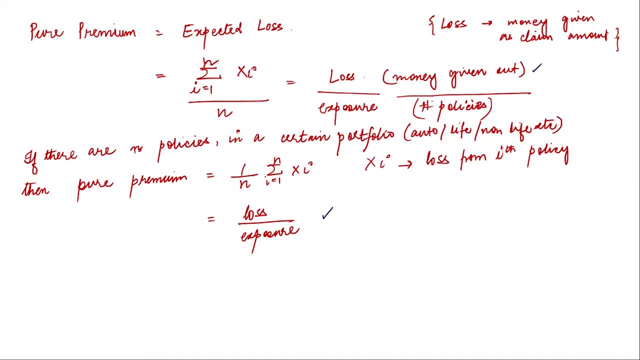 cases, divide. you want to distribute the total loss over the entire list of policies, right? so the money that five people will charge you, you need to make the rest you. you need to distribute that loss over the entire portfolio of policies. so that is why you are basically going to take 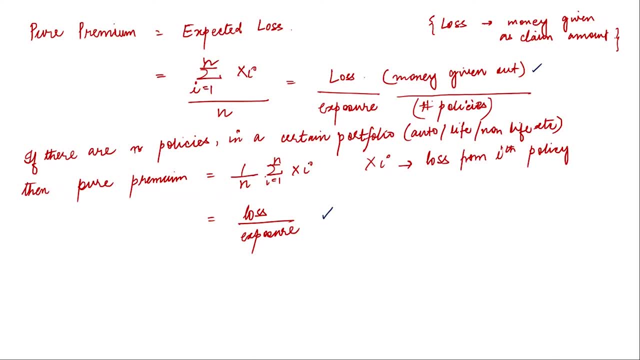 your total, the loss that is coming to you, the complete total loss and total money given out, and you divide that by the total exposure or total number of policies, that becomes your peer premium. that is the minimum amount you should charge. okay, so, uh, just you know, hypothetically just asking one more question, um, so this is fine, right? 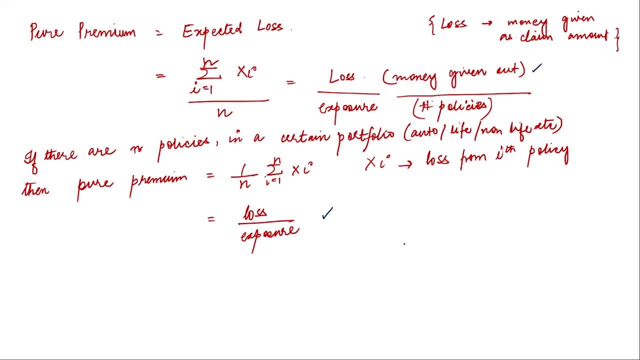 when we have a data of that for a particular year, you know how many qualities being claimed and what is the premium being paid. so we could, we could get this loss and what is the exposure. but then how about when somebody is just starting? you know don't be having, they are just going to. 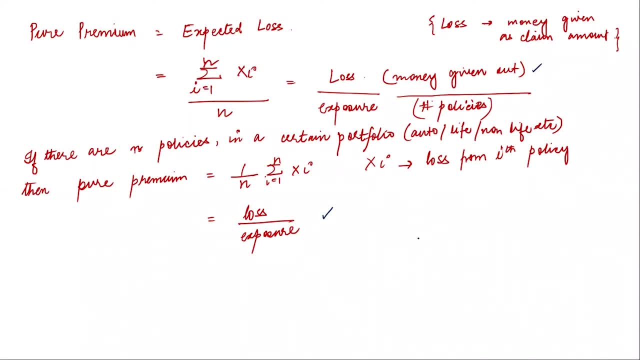 get the premium. they are not. nobody has yet claimed that time. how do they decide them? yeah, good question. so irda, regulatory authority, right insurance, so what they will do? they will have all these data. so they are going to have, um the. you know the frequency models for various portfolios, so you 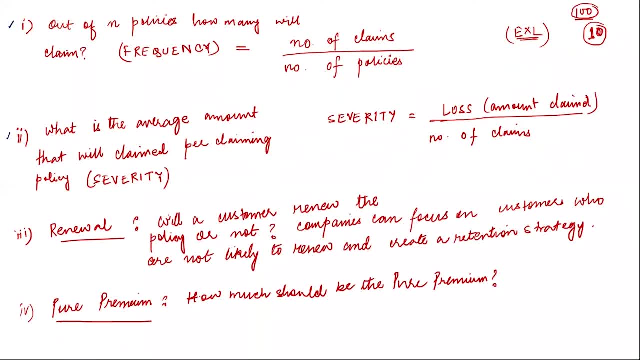 if you can, you know, get guidance over there. for example, what's the total death rate in india? mortality rate, i think for kovid it has really been skewed, but uh, the total number of, uh, i think, even even i think the total number of deaths reported have also been, uh, very different. i. 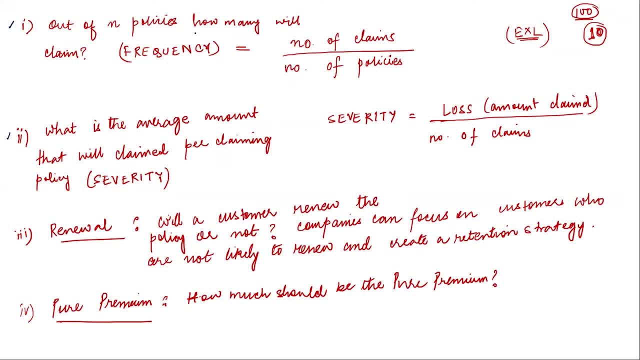 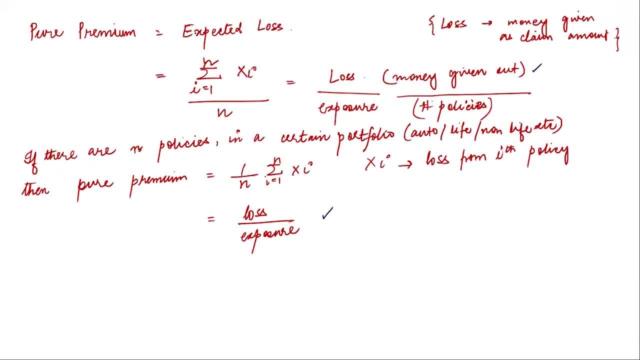 mean deaths due to kovid have gone up that's due to other other reasons would have really fallen down, so maybe the death rate hasn't really changed that much. but if the death rate changes dramatically then that can have an impact on the uh insurance company. so, uh, your question is: if you 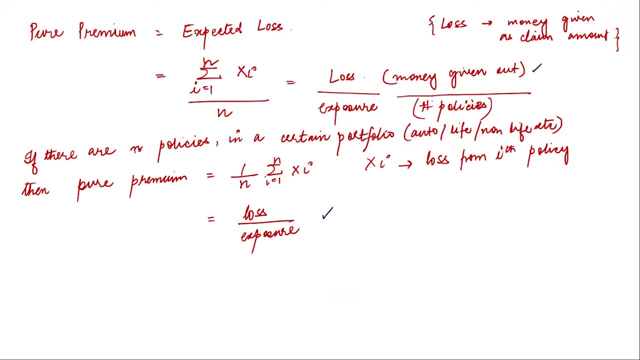 don't have your data, then what do you do? so? you use industry level averages, industry level estimates, to start with, and then start building your own data capacity, your own data infrastructure, so that, yeah, as a company, you can start leveraging your own data in order to take decisions from the next year onwards. okay, so this, both are data science problem, right? 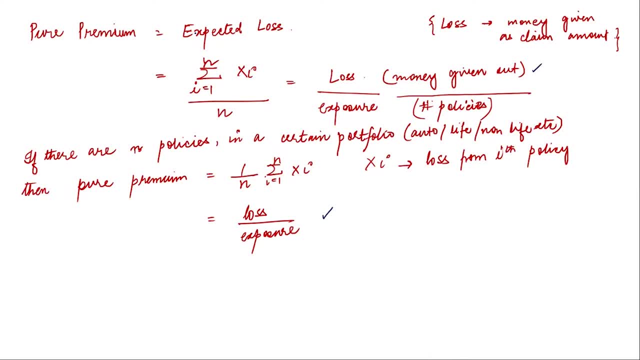 everything related to insurance is probably the only domain that will never survive. without mathematics and statistics, it cannot survive. so imagine this, right? i mean, uh, in order to figure out how much premium you want to charge- this is really the backbone of insurance, right? i should know how much premium i should charge you. if i don't know that amount, then i i cannot. 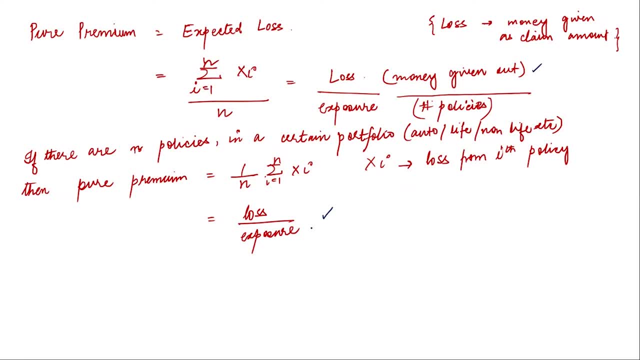 be in the business of insurance. is everybody able to relate to this, please? so, out of 100 policies, uh, five policies are clearly okay. now if say, i'm expecting them to make a claim of, say, one lakh each, so then i am looking at a total exposure of five lakh rupees, right? 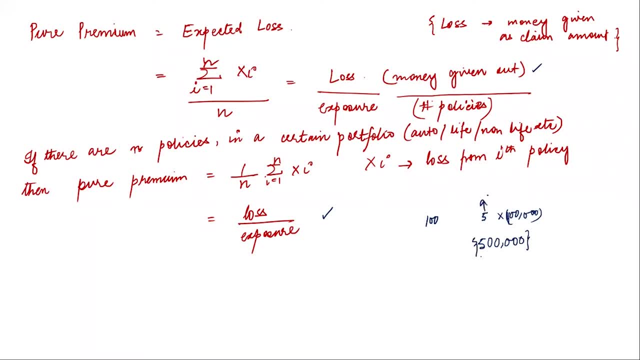 how did i get these numbers? so this came from a general claim rate, right, and this is your general severity. so you have uh number of claims and you have the severity. so you know this much is there. so how much. so if, if you're expected to give out this much money, how much premium will you charge? 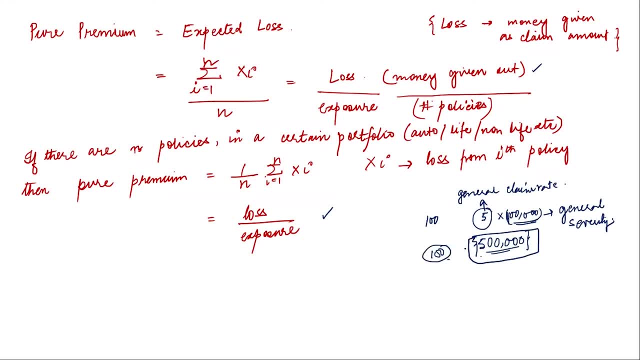 you have 100 policies, you want to make only 100 policies, so you will take this and you distribute the risk over here. right? you will say i am going to charge 5k premium from everyone so that, according to my calculations, i i am most likely to encounter five claims and each claim is not going to be more than one lakh rupees. 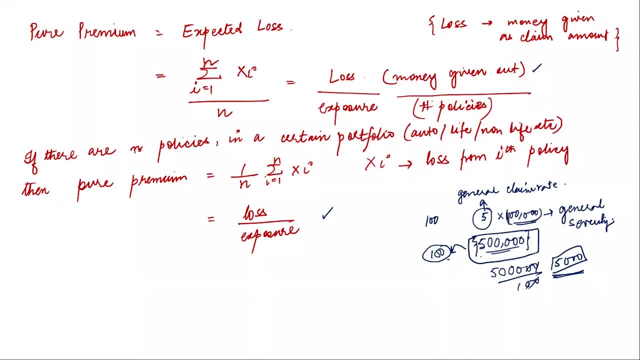 therefore, i always will be in a position to pay back the money and meet my customer liabilities and expectations. is that understood? others, others in the group? is it making sense? yes, so far, so good. right, okay, one more question. yeah, um, in the premium that is charged is on the basis of age, so how do they calculate that? 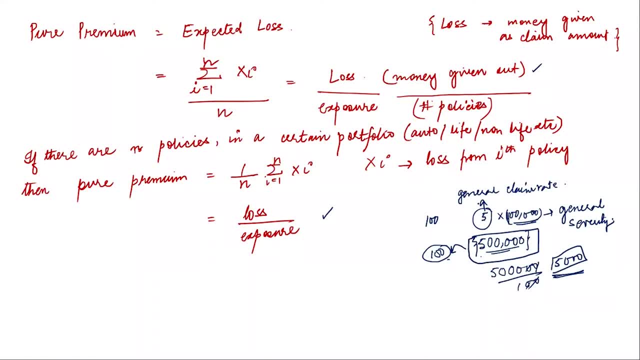 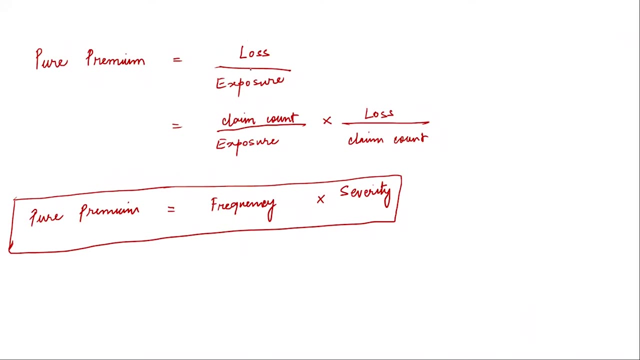 how do they calculate how much premium should be charged? yes, yeah, coming to that, but not only age, other factors also. so let's have a look. um, pure premium is lost by exposure loss. what is loss? loss is basically claim amount divided by exposure and, um, i mean, i can, i'm sorry. loss by exposure can be expressed as: 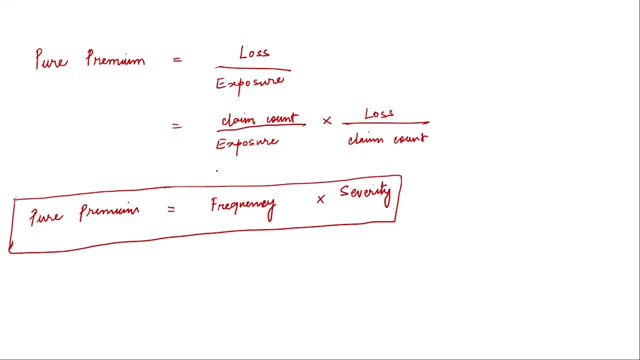 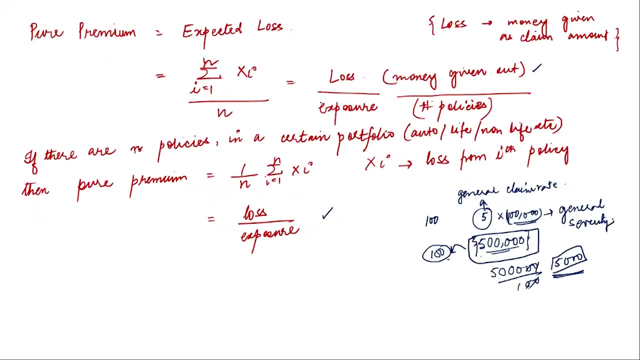 if i can put claim amount here, claim amount here, then i can cancel out claim amount right and by formula. this is nothing but frequency and this is nothing but cv rate. so if you go back to your notes here you will see number of policies by number of claims. the number of policies is nothing but exposure. number of claims. 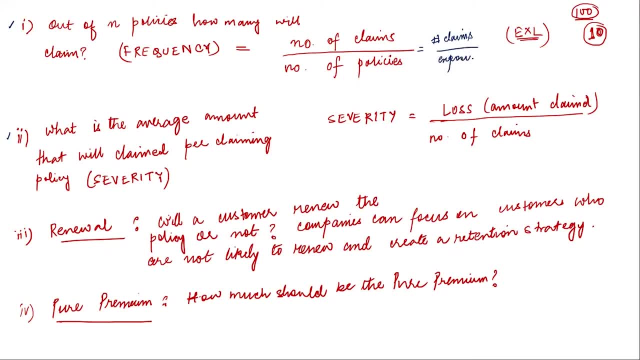 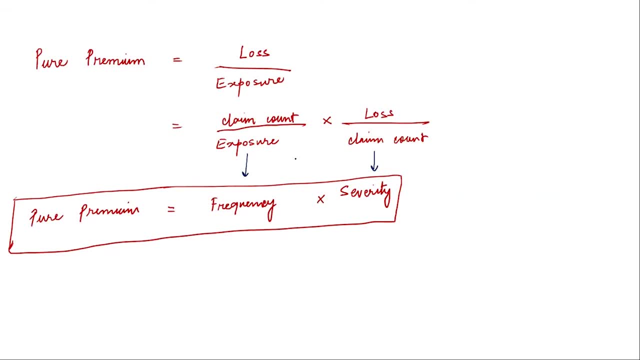 by exposure. so you have number of claim count, or number of claims by exposure, multiplied by per per claim, how much money has gone out? so frequency multiplied by cv, and so premium is calculated. basis predicted: pure premium is predicted frequency multiplied by predicted- uh, severity. okay, so there is a separate model for this and there is a separate model for this. 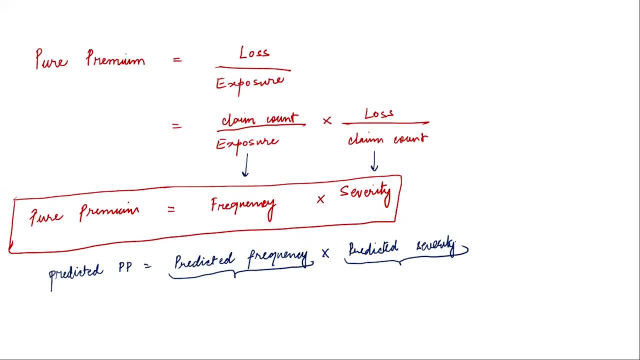 so far, so good. did i answer your question how to get the? i mean? obviously now you might ask me, how is frequency predicted? we will come to that, but but at a high level, are you getting the storyline so far? uh, your exposure means, uh, the total number of policies. yes, okay, always remember, right guys. uh, 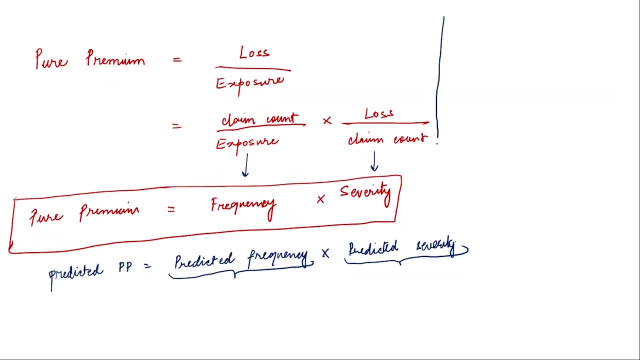 always remember that whenever you're dealing with any business context, especially in the context of risk right. exposure as a term it defines the extent of, i would say, the full extent of risk. okay, in case of banking, the risk lies in giving the loan right. so therefore, exposure. 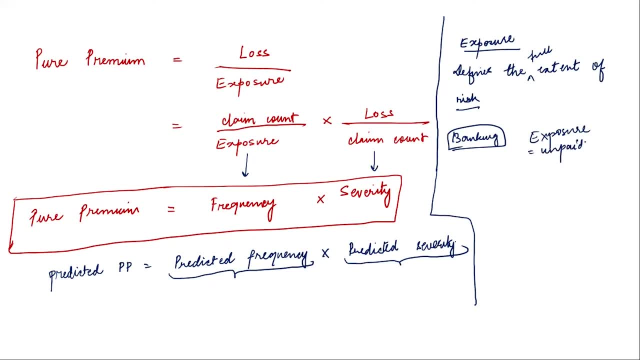 is equal to unpaid money. how much money is unpaid? okay, and in case of insurance, is the number of policies. so what happens here is that total unpaid money for a bank is they're waiting to get the money back and they're not going to that. they will be in trouble if they don't get the money back right. so always ask yourself what. 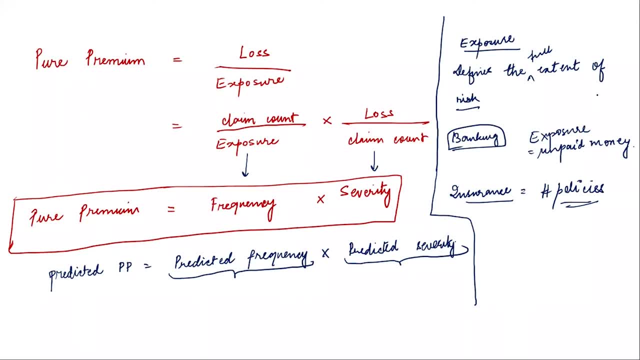 will happen so that the business will get into trouble. so in case of a bank, the money not coming back will get into trouble with get the bank into trouble and therefore the unpaid money becomes the exposure. okay, in case of insurance, the insurance company will be in trouble if everybody starts. 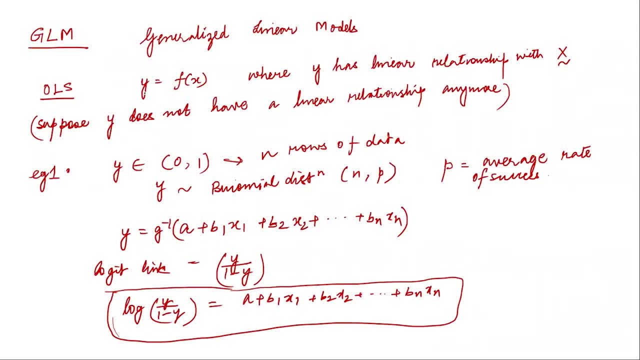 claiming their money correct. think about it. um, i'm going to teach you a little bit about generalized linear models and how that helps in insurance. why this discussion will help you is because obviously, in this class we will take a use case, we will do a project right, but then there are so. 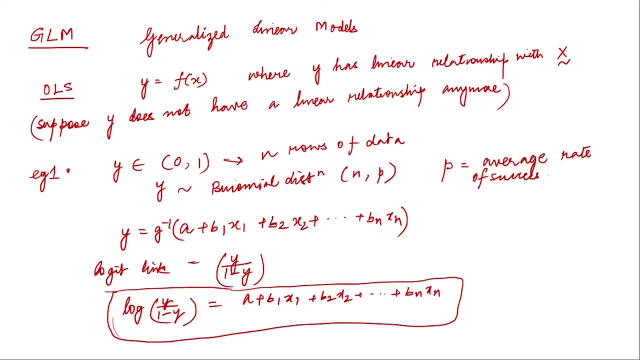 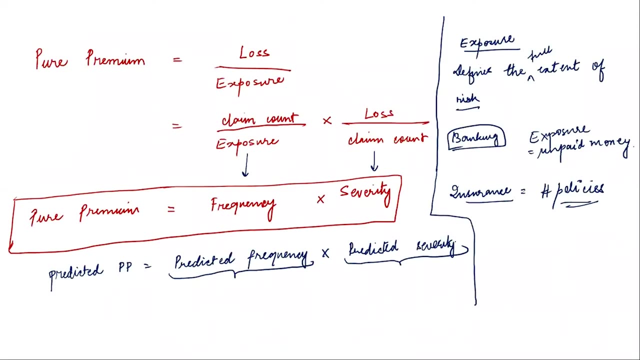 many other projects out there and, uh, the concepts of insurance can be applied to diverse cases. uh, we'll talk about that also in just a bit. but first we'll come to generalized linear models. but the basics are the definitions we just covered. we are premium equal to frequency multiplied by. 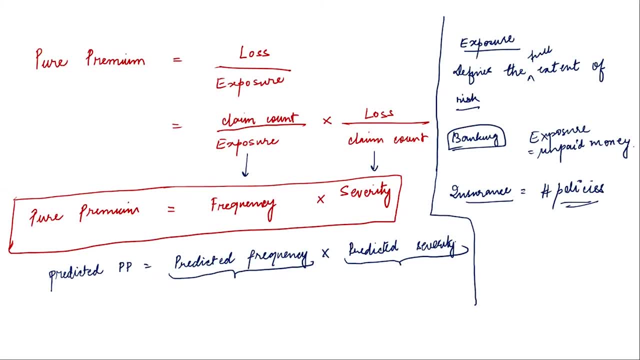 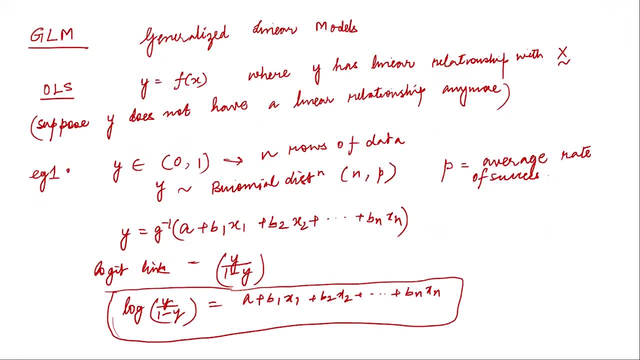 severity and uh talked about what exposure is. we talked about each of these metrics and these are basic quantities that we should be aware of- and what type of models used to solve each frequency: severity, renewal, uh, what type of model will be used? okay, we will be using something. 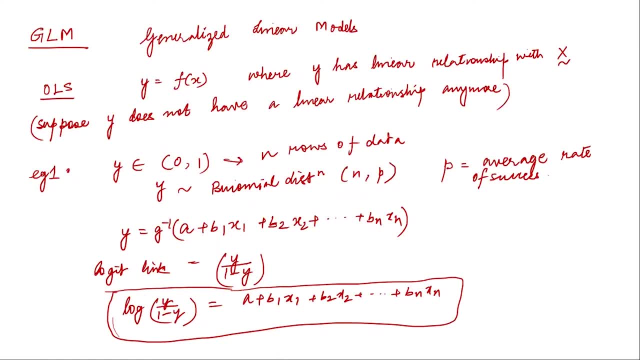 called generalized linear models. okay now, um, everybody has learned, uh, a regression, but we will do a quick division of that. so in case of ols ordinary least squares, what we have is we have a functional relationship, y equal to fx right, in which y are the dependent variable. 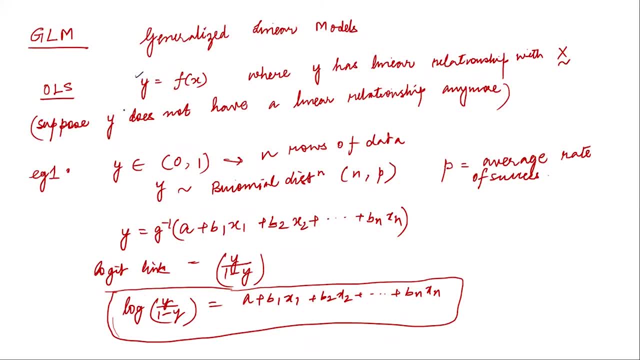 it has a linear relationship with x values. that's what happens in case of olx, so we are able to write that, okay, y equals 2 plus 3 x 1 plus 4 x 2. this is something we it's like an it's an ols. 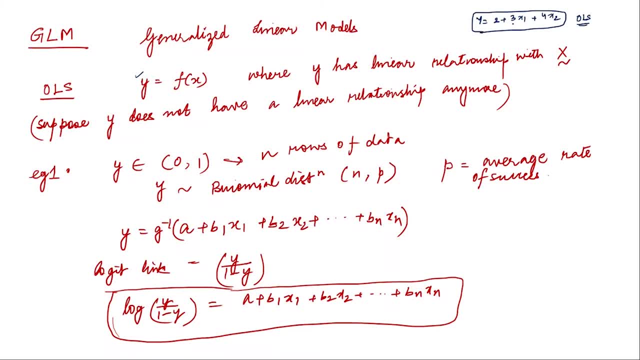 model. this is an ols model, so we are able to make this some something like this. uh, build an equation like this because we know that y will have a linear relationship with all the x's- everybody with me so far, okay. now imagine that your hands are tied. 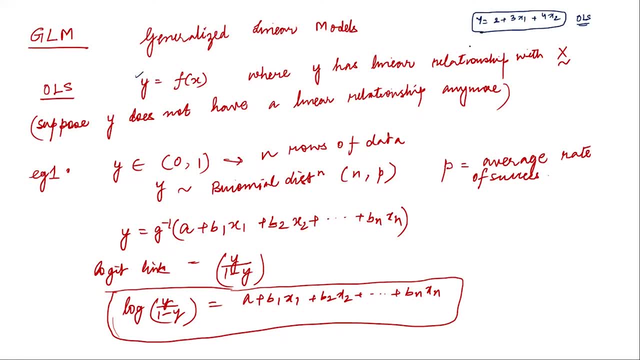 you, you, you cannot mathematically express the relationship between the dependent variable and the independent variable in this format. then what do you do? suppose y does not have a linear relationship anymore? imagine that y takes only two values, zero and one, and you have n rows of data, right? 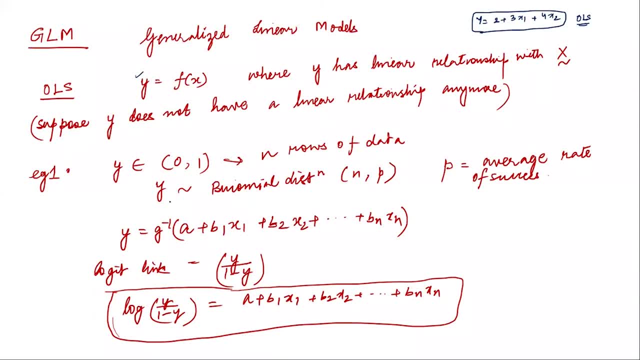 and uh- number of rows of data you have. so y does not come from normal distribution. y comes from binomial distribution where parameters are np, n is nothing but number of data, uh- number of rows of data, and p is the average rate of success. so, out of n rows of your data, number of rows where target equal to one and number of rows equal to. 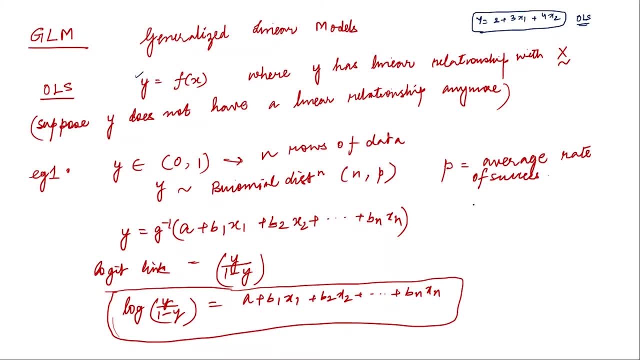 where target equal to zero. you will be looking at all of that and essentially calculate, uh, the percentage of rows where target is equal to one. that becomes your probability of one right. so therefore, uh, why can be said that y belongs to binomial distribution with parameter np? 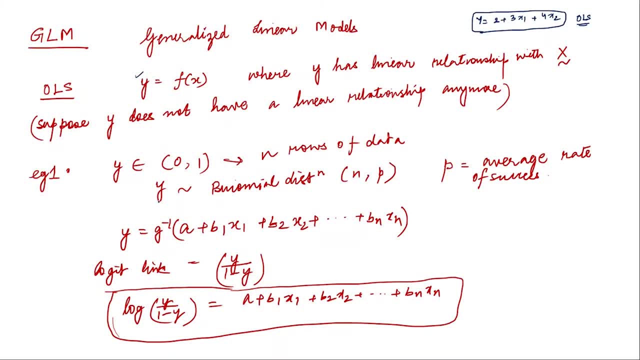 now, in this kind of a context, right where y comes from binomial distribution, you cannot expect to write something like this. so what do you do? you introduce a certain function called a link function. you say that, okay, i know that directly. i cannot write this: y equal to a1, a plus b1, x1 plus b2, x2. 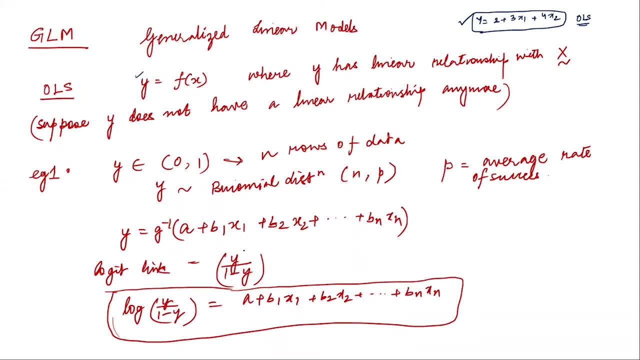 directly. you cannot write. therefore, let me bring in a intervening function called link function and let's use that link over here. so in case of logistic regression, the link function will be called logit link. it is: this is the logit link. okay, so you can't say y equal to a1, a plus b1, x1. 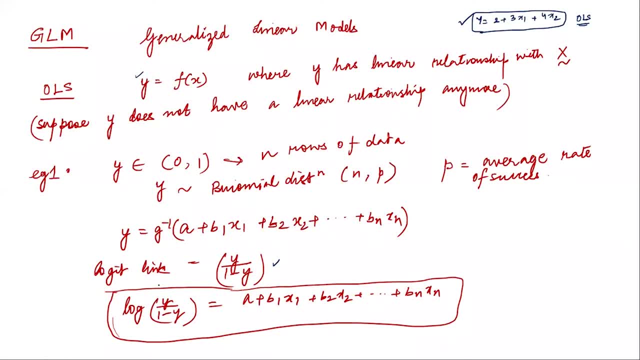 linear combination. but you can say that logit of y, you can express the logit of y equal to a linear combination. that you can do okay. so you can't say that y has a linear combination for sure. but if you apply the logit function on y and say logit of y, logit of y has a linear combination. 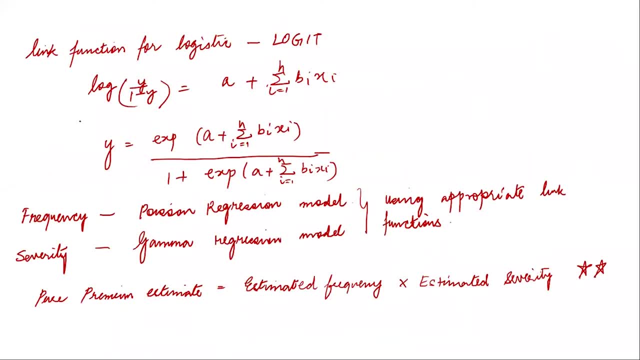 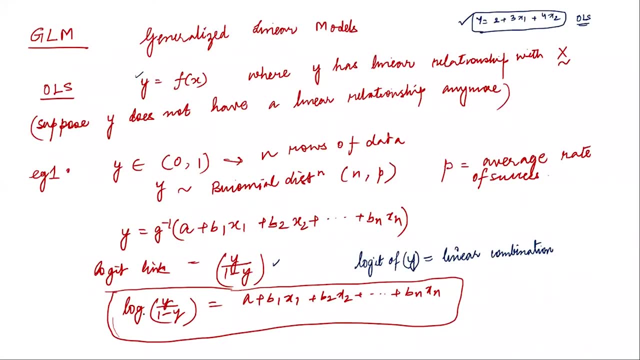 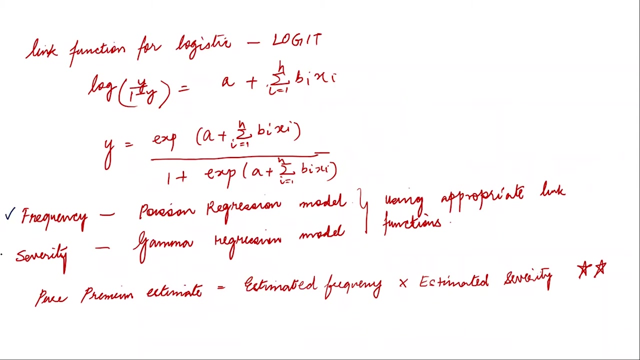 okay, so this becomes your uh. it's a generalized linear model. so once the moment i write this uh log of y by 1 minus y, equal to a plus b1, x1 plus b2, x2, this one. so this is an example of glm. now, in case of frequency, we use poison regression model and we use gamma regression model for 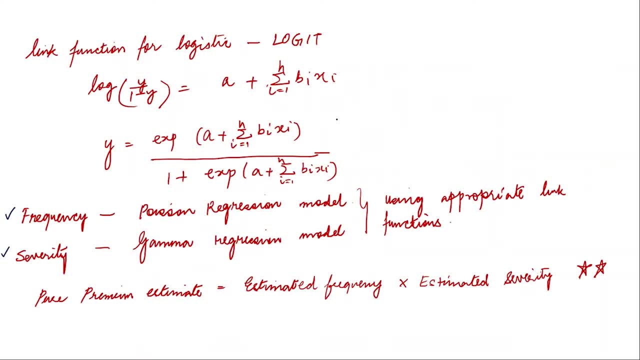 severity. so they are a different link function, mostly log link functions. but uh, there's a separate kind of models called poison regression model and gamma regression model. both of these models, uh, they are going to be outside of our discussion right now but we can check. i, we can. 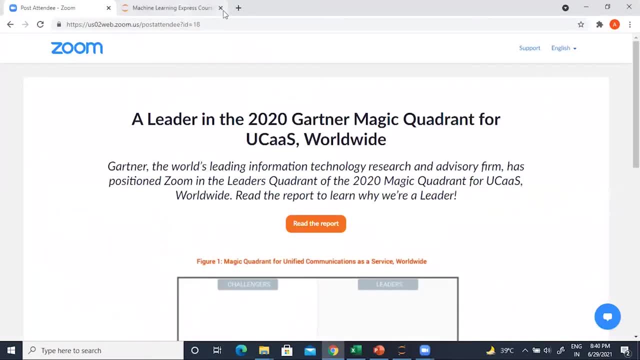 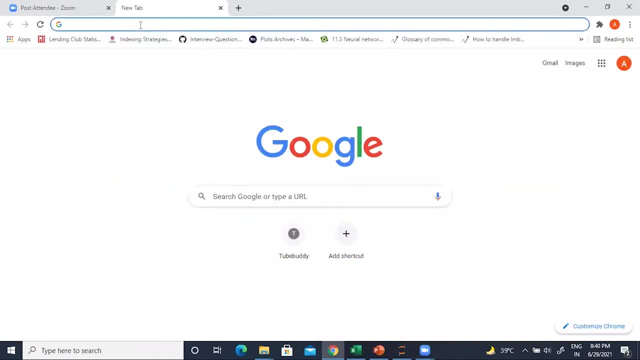 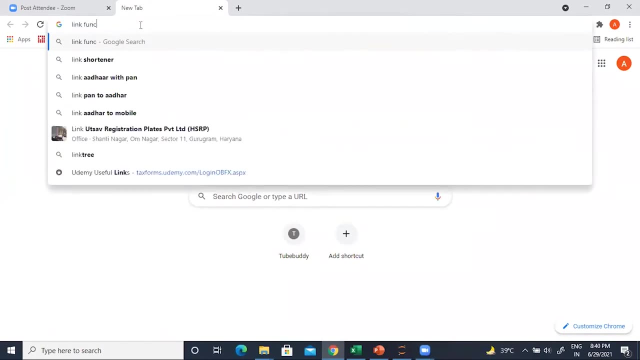 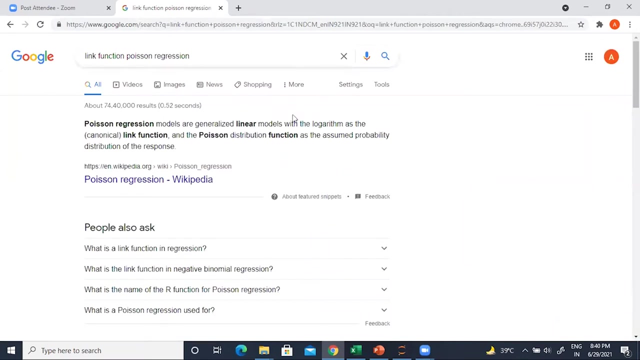 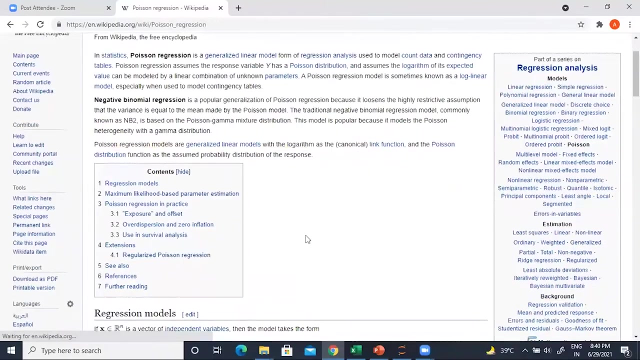 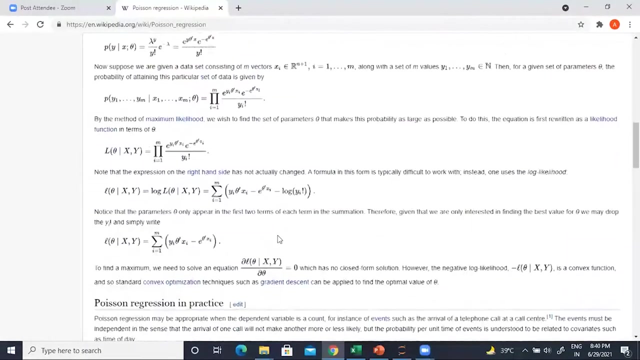 check online. i think, just give me one moment, let's go here. yep, yeah, uh, our generalized linear models with the logarithm as the canonical link function. so it's basically log link. okay, so log link will be there. yeah, log of y will have a linear relationship with: 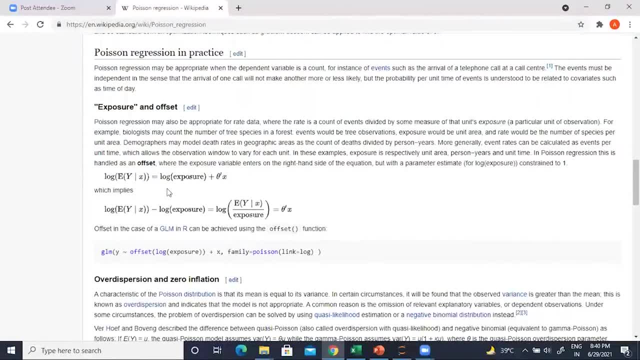 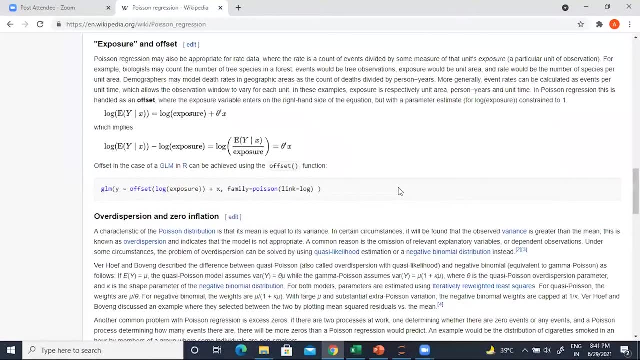 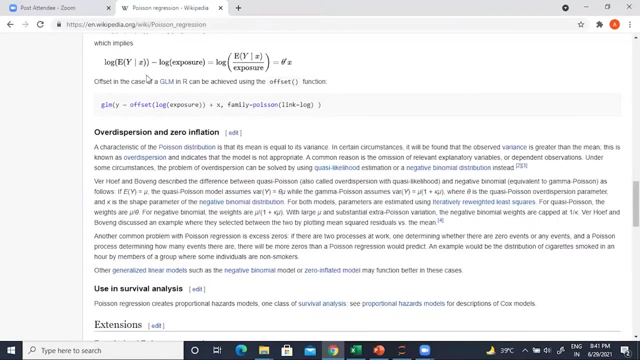 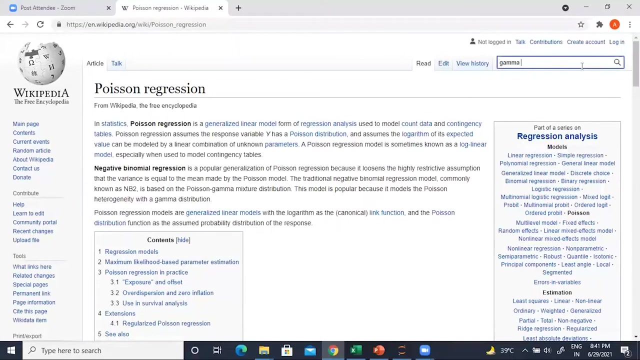 there you go. you can uh do glm in r. or if you want to do glm in r, you can do glm in r. you can do glm in this thing also, python also uh. essentially, um, the log link. log function will serve as the link function. okay for poison distribution, but for uh comma regression. 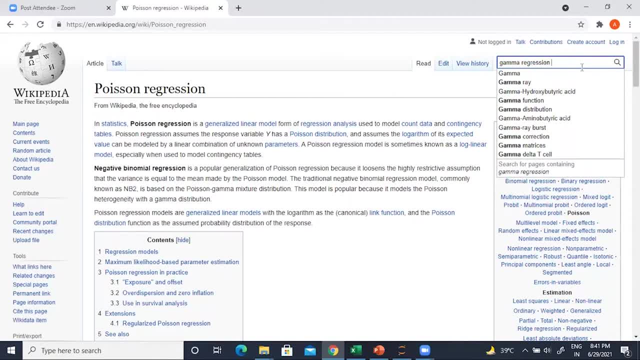 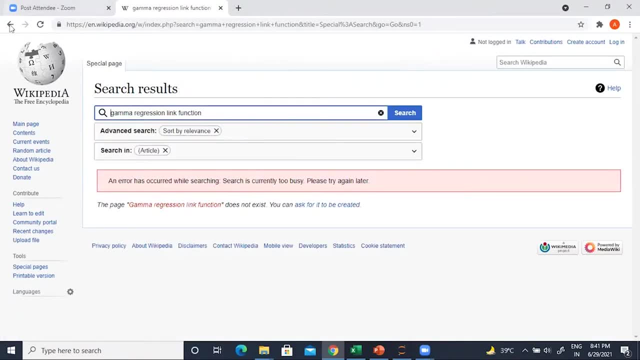 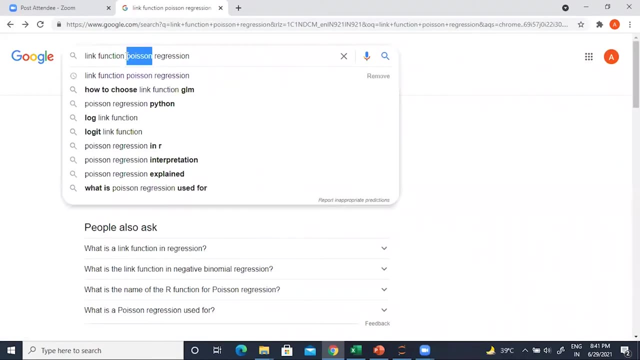 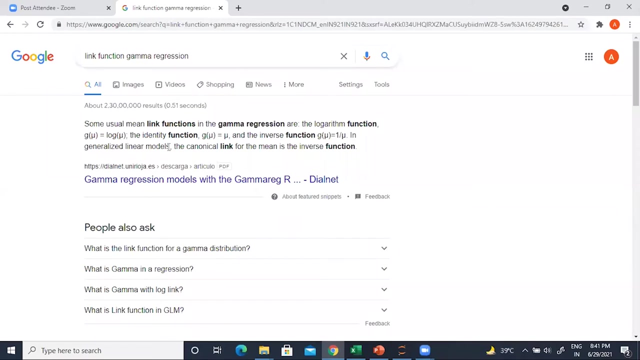 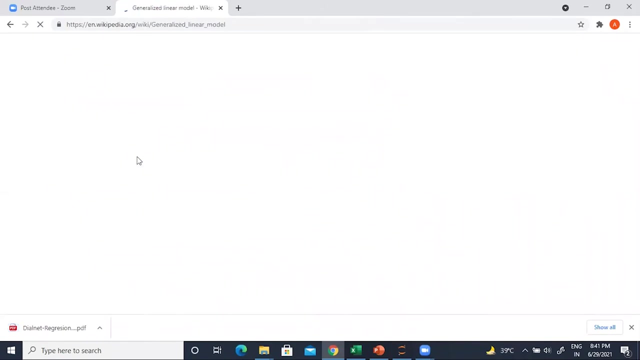 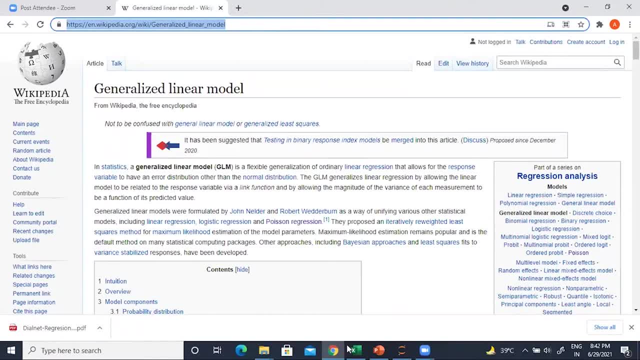 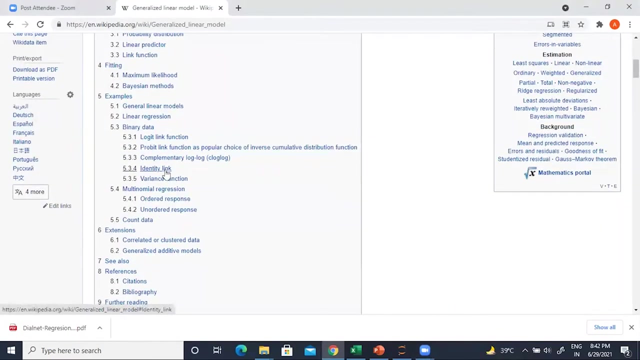 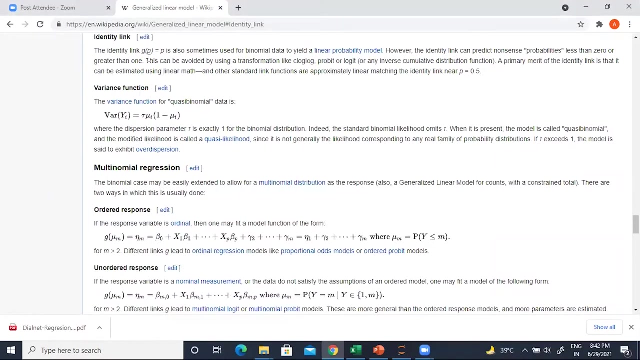 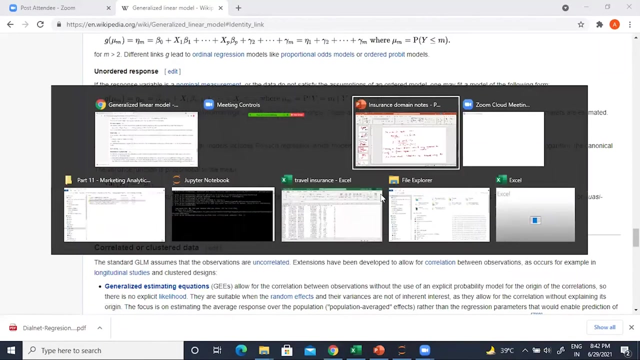 Just a bit. I'll share this with the chat window, So for you've got simple linear. They're also family of all these things. Identity link is case of comma, So you can do some more research on this. but the thing to note here is that in the context of today's discussion, 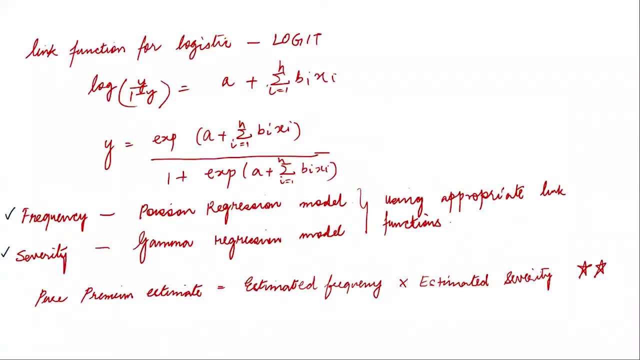 is that you know there are other models, other than OLS models or even normal regression models, which are used in case of insurance, And that's why this is a very data science-heavy industry where especially stats related work is like heavily done because you have to come up with all these things. 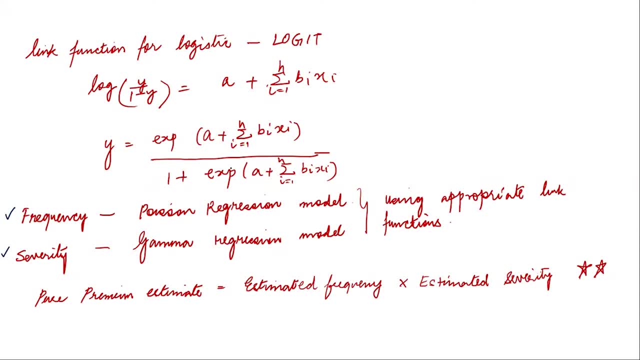 you know, specific models was predicting specific outcomes. Now, why did I? why are you choosing poison regression for number of games? What reason for this? I'm going to do a little bit of research and you can see how the data science could be used here. 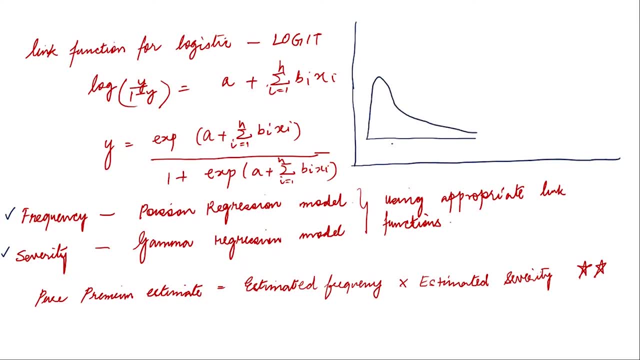 We are looking at there right now. So we can see that this is a number of these in a very simple way. So we can see- I'm going to get a comparison here- We can see that this is the number of games, right? 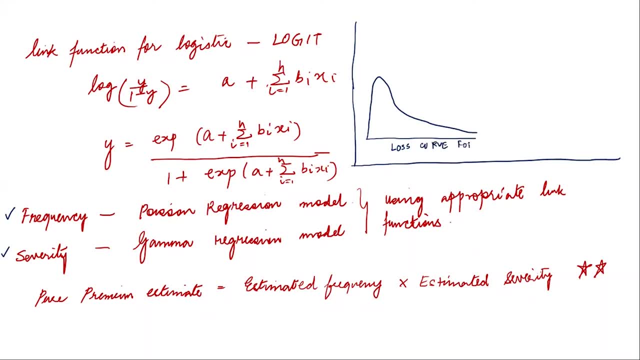 We can use. you know, this is the number of games and this is number of venues And we can see how people the market is going. then we can also see that we have some data we can also see. let's see. 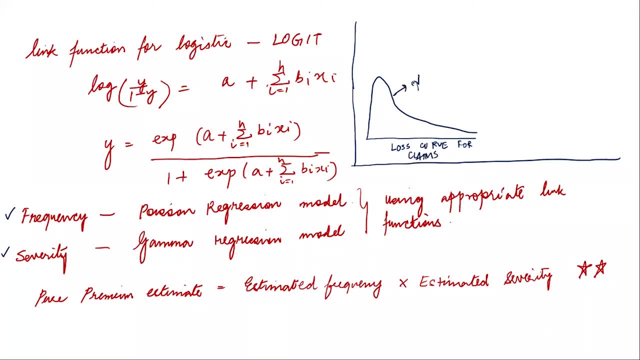 that these are the games that we are going to use. You will see we do not have stock of these games. I can see the number of games that we are going to use. Now that I have the data, let me see if I have enough of them. 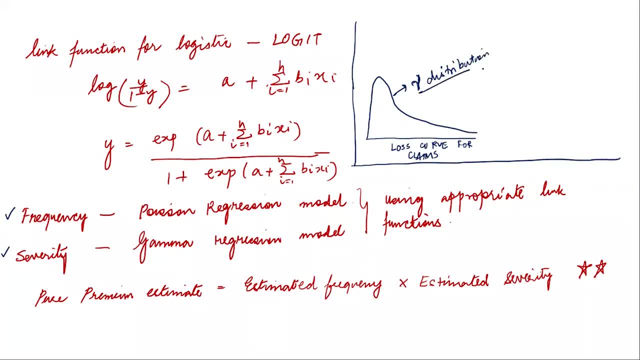 so we can make sense. but number of claims. number of claims is it is supposed to follow poison distribution. so always remember that poison distribution is used to estimate number of events. it is always used to estimate the probability of number of events. so basically, um, that is why you are using poison regression process here for frequency. now coming to our 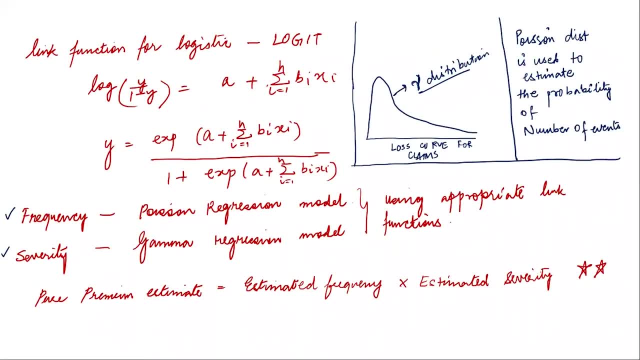 problem statement. the problem statement that we are dealing with is the probability of changing, so basically that uh people have almost, uh they're at the end of their uh- you know- term as a customer and they have to basically renew their um premium right. so what are they gonna do? 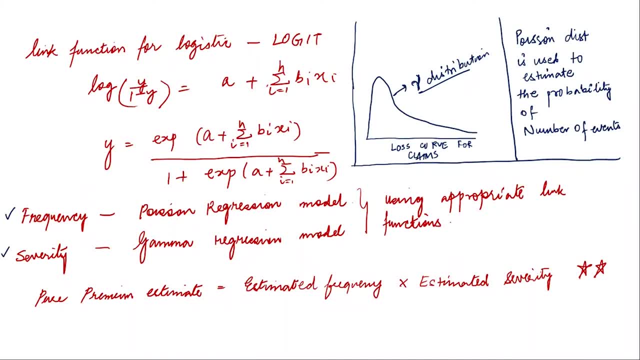 uh, how? how can you figure out who's likely to get give their, you know, get a renewal done and who's not likely to get a renewal done? so that is a statement that can we predict which customers are likely to get a renewal done and who's not likely to get a renewal done? so that is a statement. 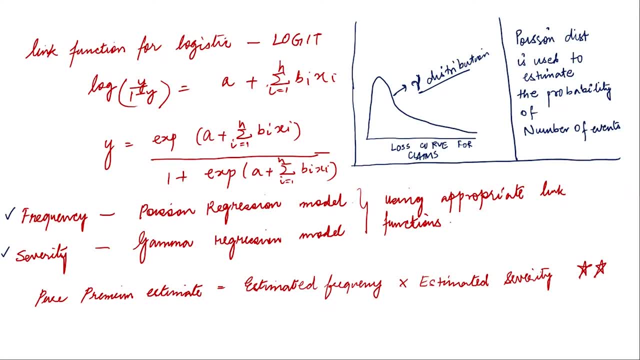 that, can we predict which customers are likely to give us- um, you know, renew their policies and which customers are not likely to do their policies? so that's the statement and then i'll walk you through the data to see uh, you know, discuss the quest, different uh features that are there and 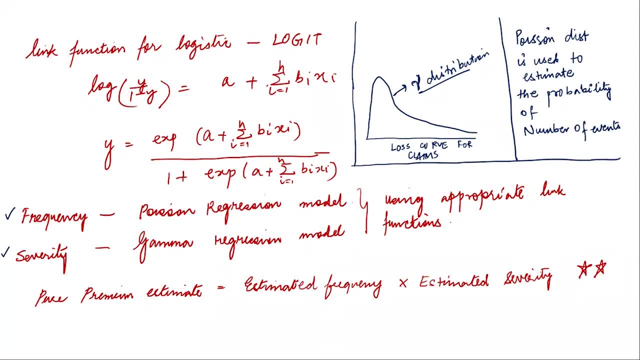 explain the, uh, the approach that we will take, but before that i just want to pause and see if you have any questions. can you please explain this graph, like blaster for things, how to read this? okay, so, um, okay, the only way to do this is, uh, into two sentences, basically: majority. 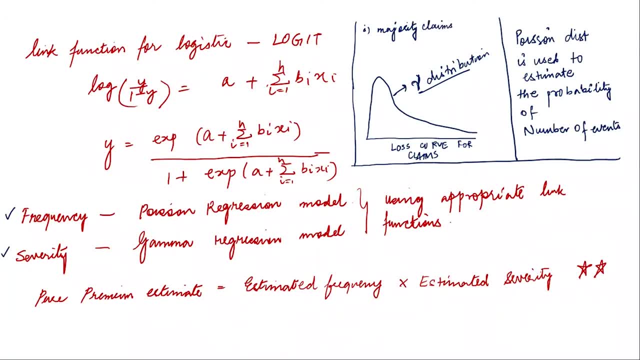 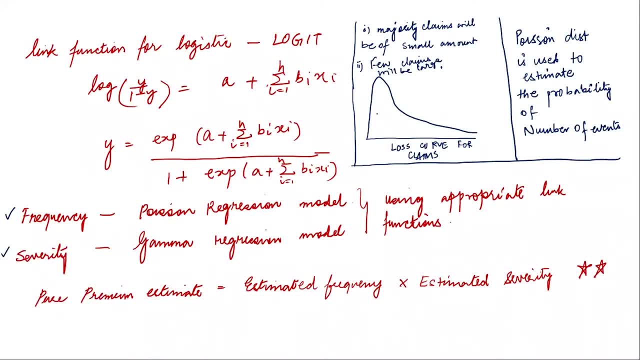 one moment. this is where. this is where this is where larger claims are taking place, right, large claims, large claims, large claims. and this is where smaller claims are, and this is where smaller claims are, and this is where smaller claims are taking place. so you can see taking place, so you can see. 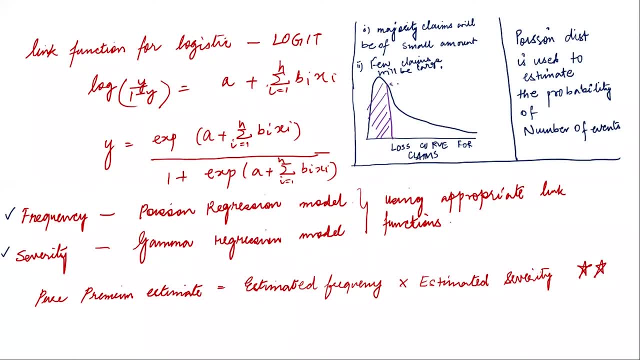 taking place so you can see the number of people, the number of people, the number of people who are claiming small amounts are from. who are claiming small amounts are from. who are claiming small amounts are from year to year, but only year to year, but only year to year, but only people who are claiming like big amount. 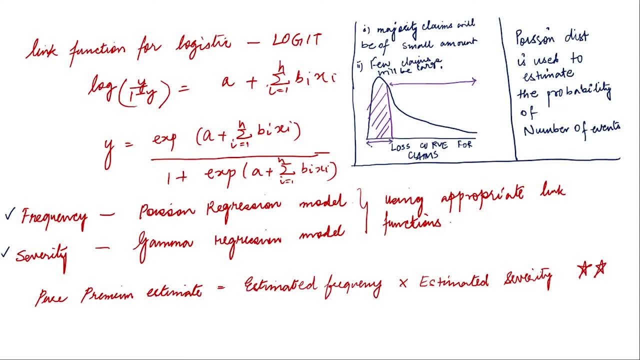 people who are claiming like big amount. people who are claiming like big amount of money are only this much right of money are only this much right. it's a right, skewed distribution making sense. yeah, thank you for this. where have you seen this distribution in your stats classes? 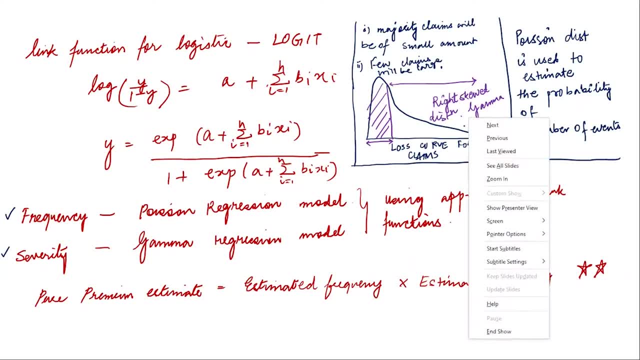 what is? what is the? uh? you know, in hypothesis testing you would have done chi square test. remember, all of you would have done chi square test. chi square curve is also like this, because chi square is a modified gamma distribution curve. so it says, uh, it's the chi square distribution is. 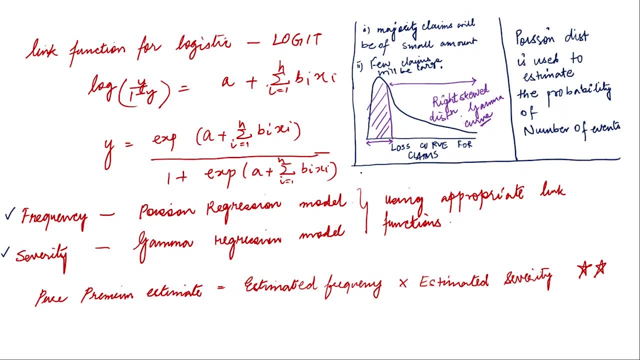 derived by some of the individual gamma variance. so that's why chi square curve will also be something like this. but the point to note- i will forget about the curve and the distribution. the point to notice that um majority of claims are going to be small amount. only few people will claim that. let me take an. 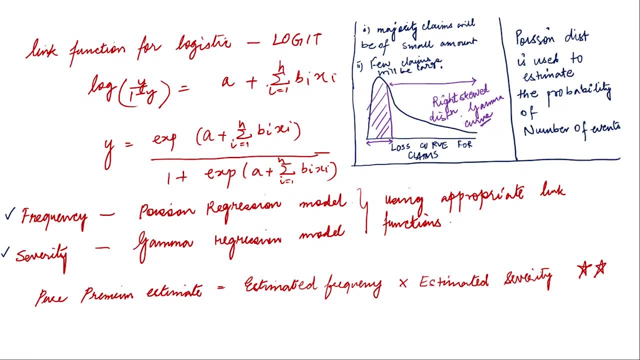 example. this will clarify everybody. say: all of you have cars, okay, and you have insured your cars. can everybody relate to that, please, okay, okay. now it is likely that some of your cars will get some damage during the year, so you might just- uh, you know- get some claims. that is possible, but how much chance is there? 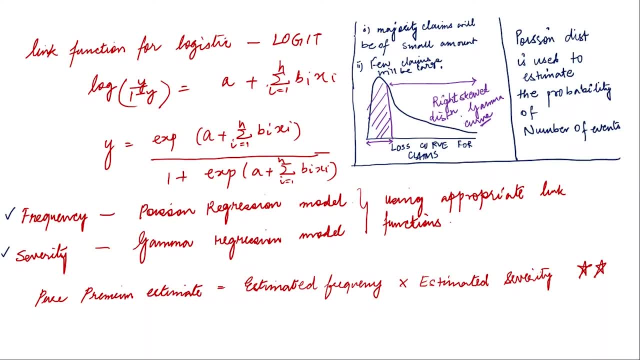 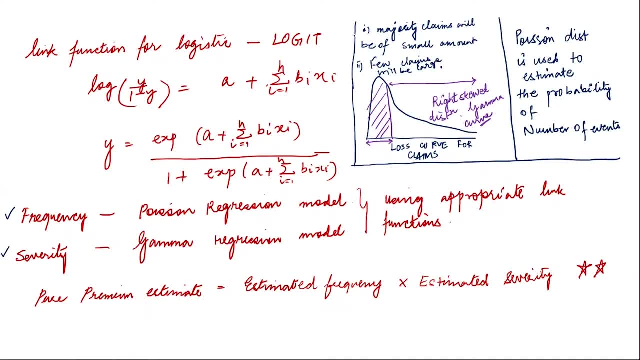 literally smash. some trailer has literally, you know, bulldozed your car and gone away like you know, something like that. there was a picture of, uh, i think, kia seltos, where the kia center broke into two halves. that is a total loss. there was a picture of a maruti bolino once after it was. 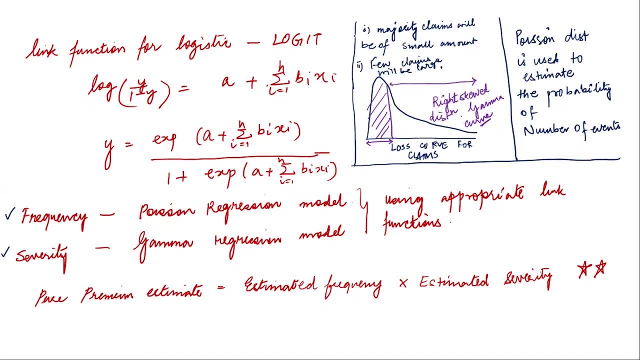 i think shortly after it got launched, a few years back, there was a very bad accident. it happened close to punjab, uh, i think it was a complete block. i mean, think about it, right, but those are rare events. so therefore, uh, large claims are not very common, but small claims are very frequent. 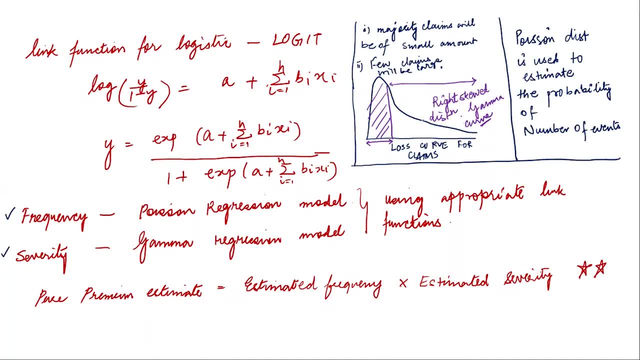 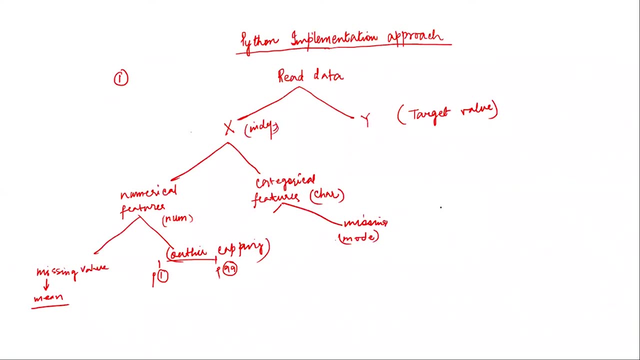 very, very, you know, quite common that that is fine. so that that is why this is. this is the nature of the graph. it is because of that reason is it making sense. everyone, okay, all right. so, uh, now we are going to, uh, okay, come up with a, you know, implementation strategy. but let's have a look at the data. 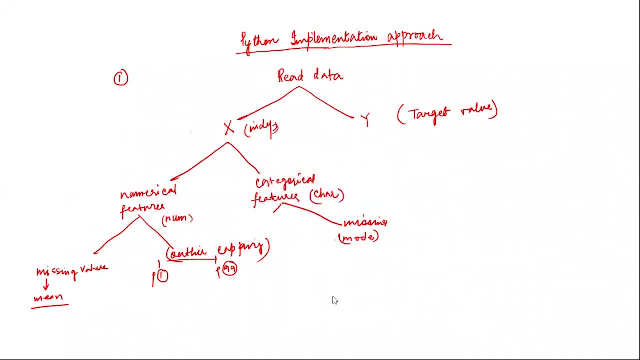 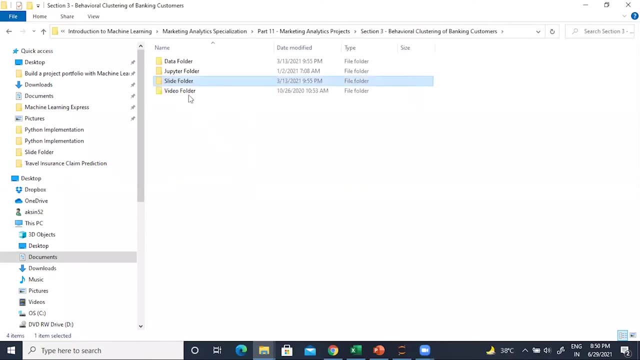 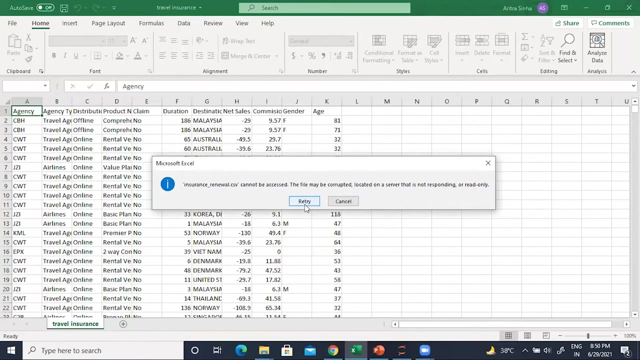 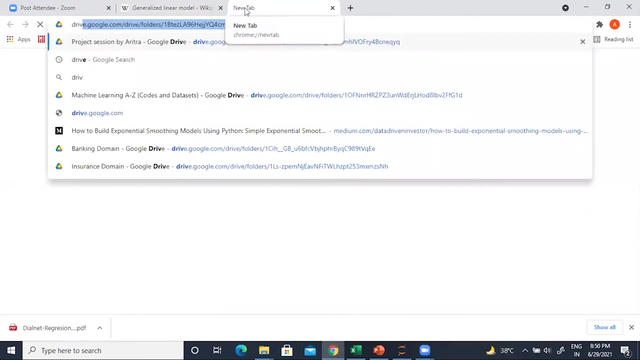 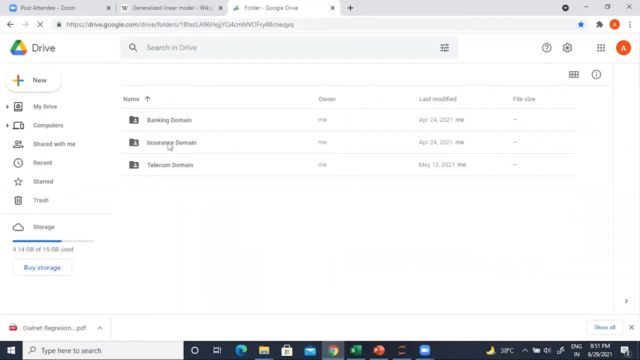 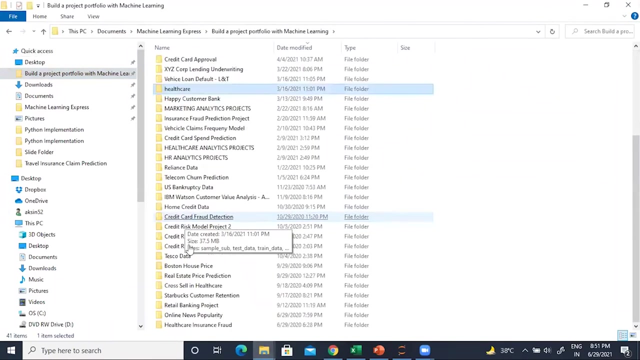 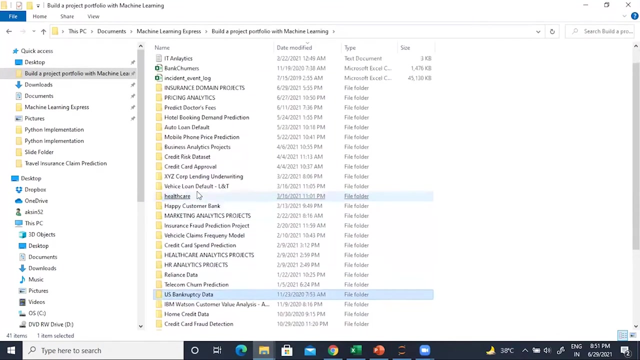 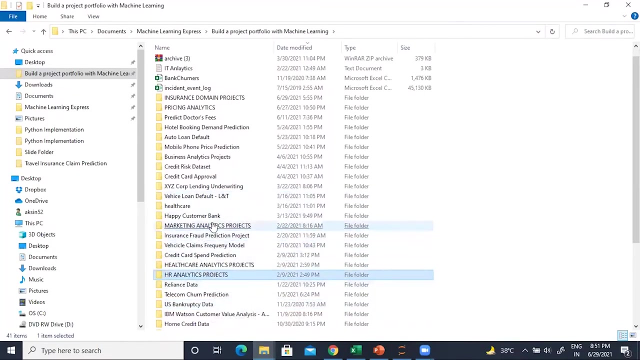 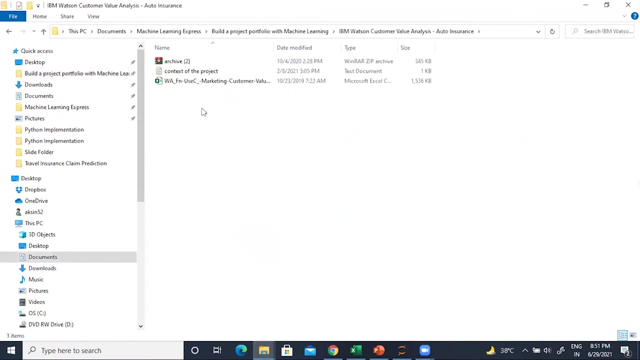 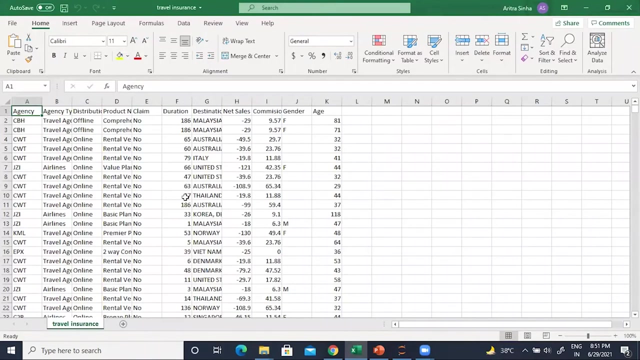 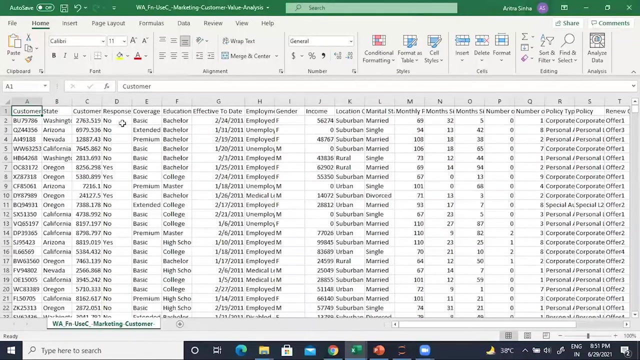 to get a feel of the overall data, to see you know what kind of variables are there and what can we expect from the data. oh o, okay, looks like there is an issue. let me download this stuff once again. Why would that be an issue? Yeah, okay, we have it alright. so you've got all the customers here. how many customers? 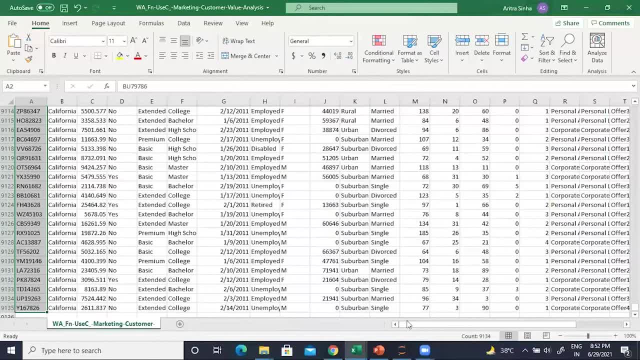 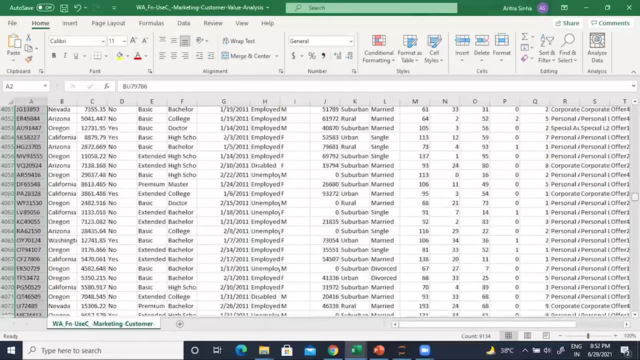 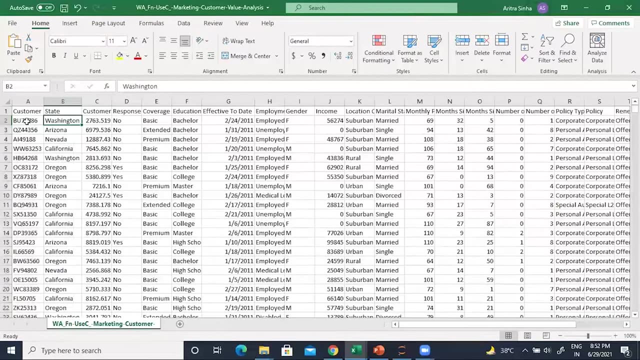 do we have? We've got data for 9000 of customers. okay, not a very large data set. This is a data set that IBM has come up with for practice purposes, so that's fine. So we've got about 9000 odd customers. then we know where they live, which part of the US they live. that's there. Now the other part comes, the other feature content: lifetime value. Lifetime value is a marketing concept where when a customer is acquired, then the customer you know, you can try to project that if the customer is with you, you define something. 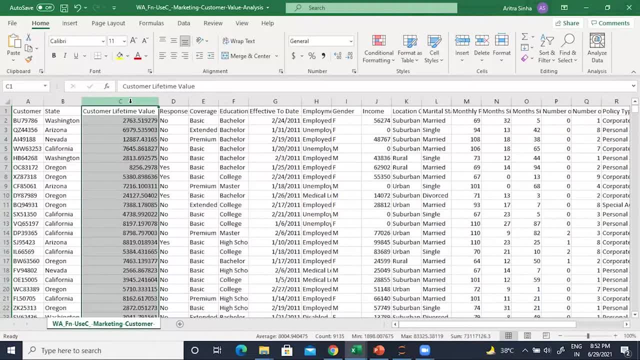 called a lifetime. That okay. if five years is a lifetime for a customer, okay. now if a customer is with you for five years, then how much value can you derive out of the customer just because the customer spends like that much time with you? 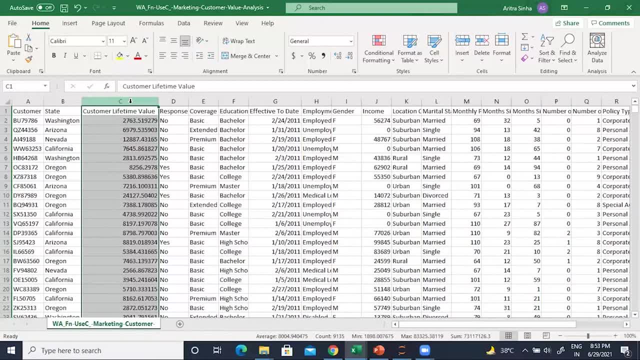 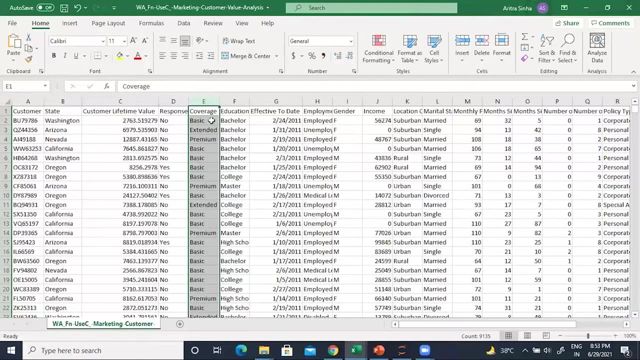 So it becomes customer lifetime value. Now, in the past, whether somebody has responded to a renewal offer or not, that is there as a response, Yes or no. then you've got the nature of coverage. So some coverages can be very basic. it does not come with a lot of features, not a lot. 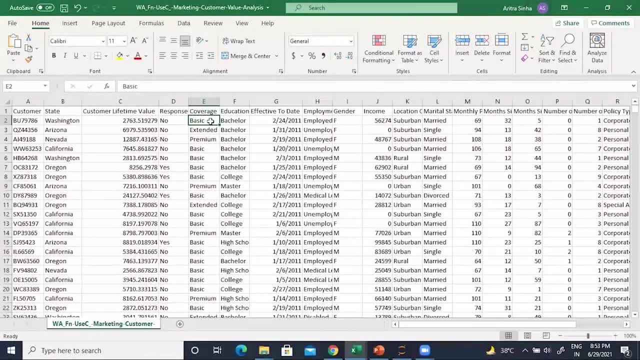 of riders, etc. Sometimes you know you might come across things like if you take basic coverage, then on roadside assistance is not included in your coverage. I don't know, some of you may have come across this in your car insurances. but basic coverage 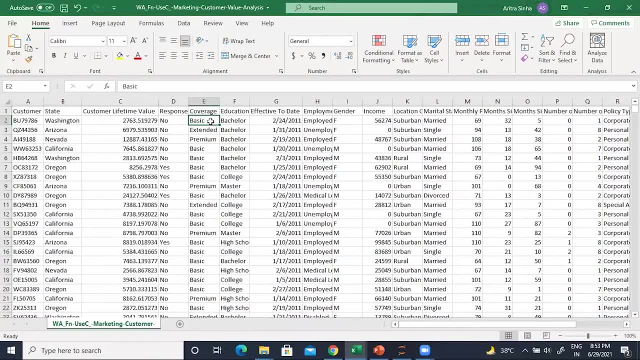 does not. It essentially contains any frills or any extended services. Now comes extended as a another type of coverage, where you have slightly, you know, additional, few additional facilities and a few additional riders. Then the third comes, premium, where you can expect more one on one kind of service, where 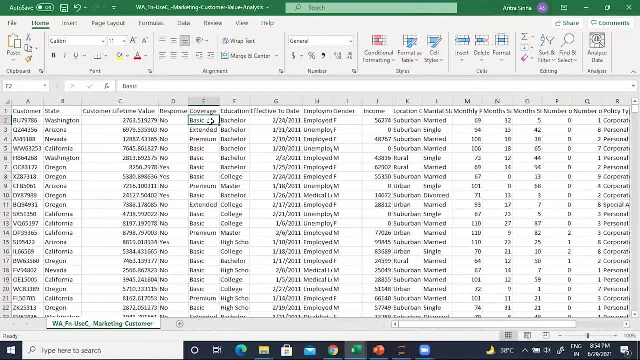 you could potentially have a concierge for your insurance requirements. If you get into issues, then you don't have to call a. you know a number where you have to be in a queue. Okay, There's a dedicated line given to these segment of customers where the queue is much shorter. 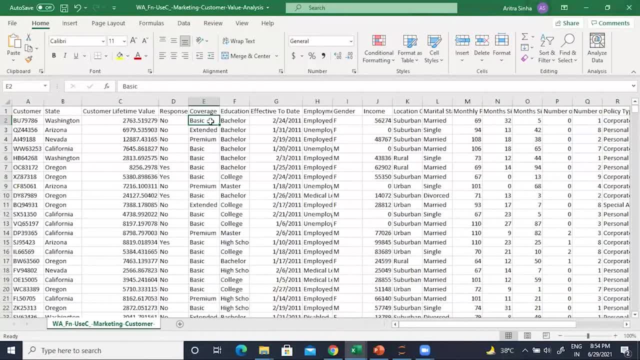 So those kinds of things can happen. Basic, extended and premium are the three types of coverage coverages that is provided. Now comes education of the person who has insured, the insured individual. That's there in various degrees. So let's have a look at what are the levels of insurance. 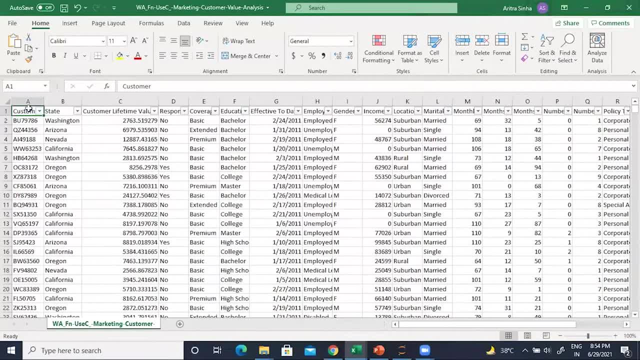 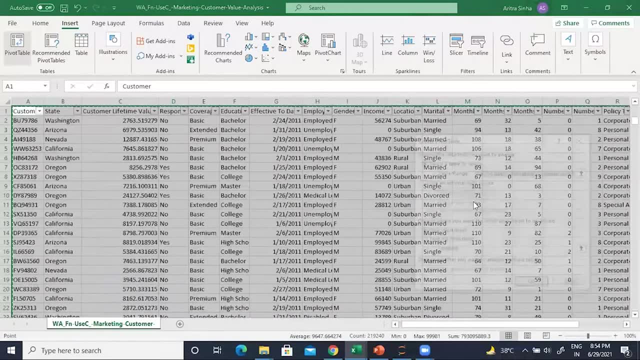 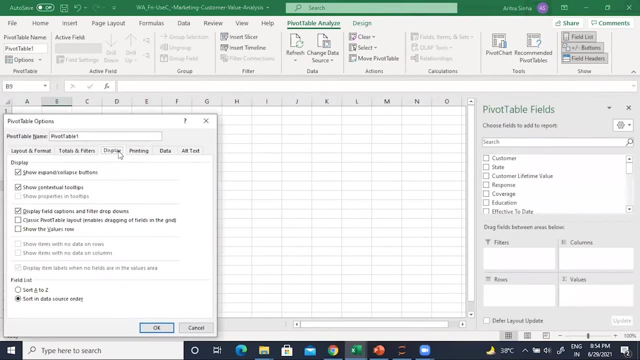 So one of my sorry education, So one of my favorite ways to look at the data is just, you know, select it all in Excel, go to insert, go to a pivot table and simply explore the data quickly. So if I just stick to the classic layout, I can quickly see what is going on, although 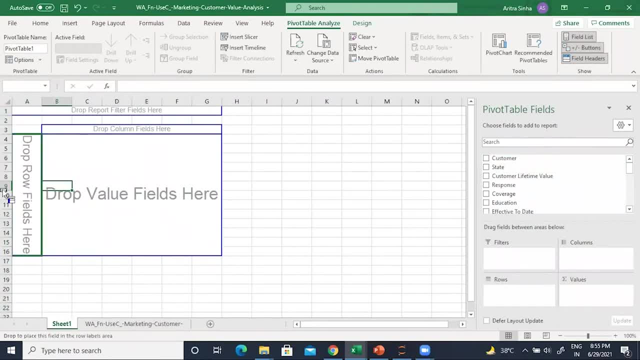 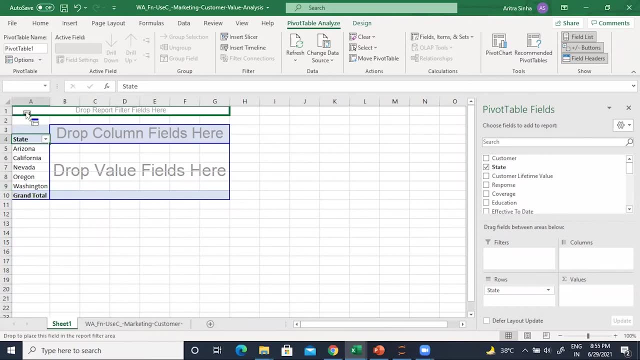 in Python we will be doing it systematically, But in case of states, so let's say, I bring it here So I can see that people are, you know, people who are insured are from these five states. only Awesome, What's the overall response rate? 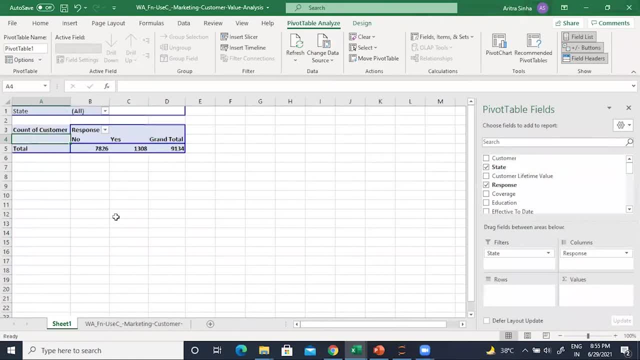 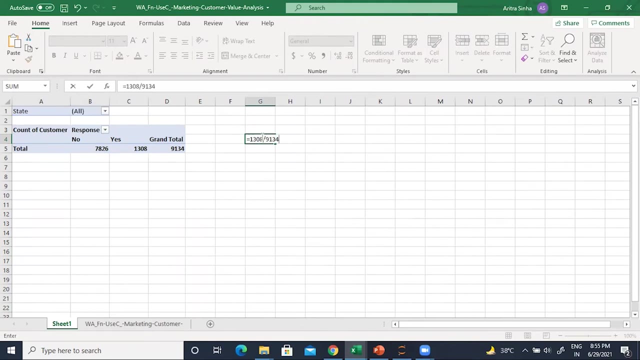 If I want to find out yes or no, then let's get the number of customers. So these many people have responded, these many people have not responded right. So 1308, typically divided by 9134, 14%, is my response rate or chance of success to a. 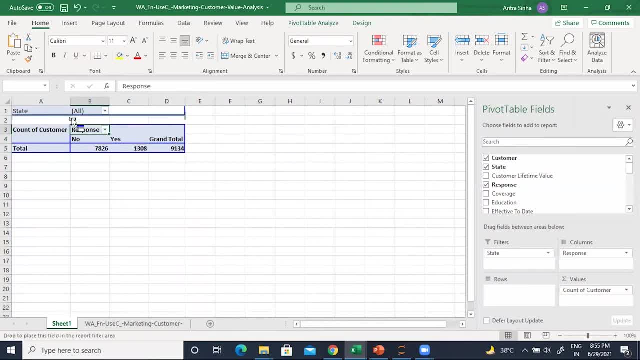 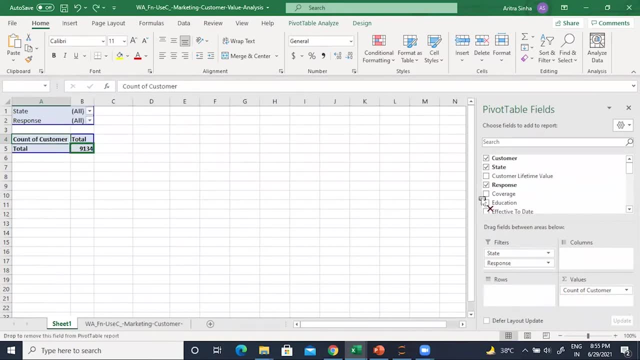 prior campaign. So that is what I'm going to use for any further analysis. Okay, Now, if you bring in lifetime customers, I'm sorry. let's get rid of count of customers, Let's begin lifetime and let's begin response over here. yeah. 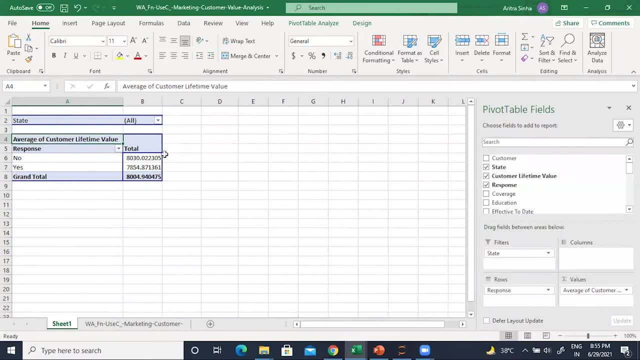 And if I double click on this and I get average, I can then compare the numbers. So we can see that whether you're a responder or you're not a responder, it doesn't really matter, You can. essentially, you know you're similar. 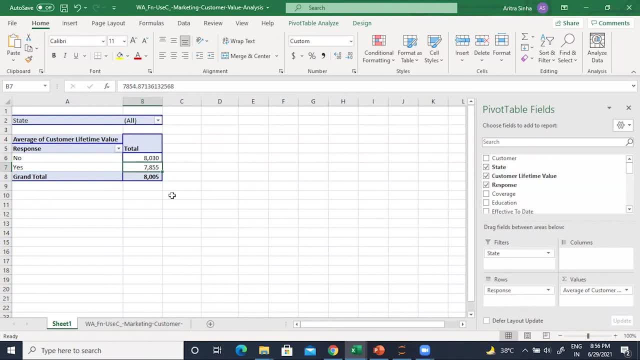 So lifetime value is not Okay. It's not going to help us identify who's going to respond, because people who have not responded, they have slightly higher lifetime value and only very slight difference. The difference between these two values are not that much. 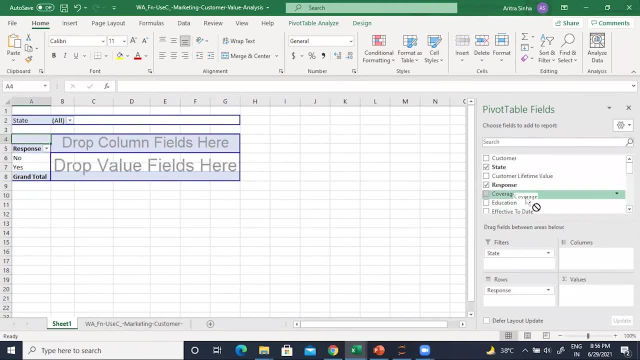 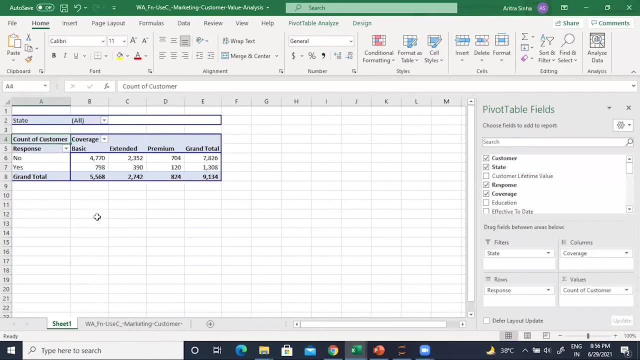 So that doesn't help us. Now comes coverage, So we bring it here. Can we bring in the number of customers? We can see what's going on? So majority of the responders are from basic coverage. That is because most of the customers are from basic coverage. 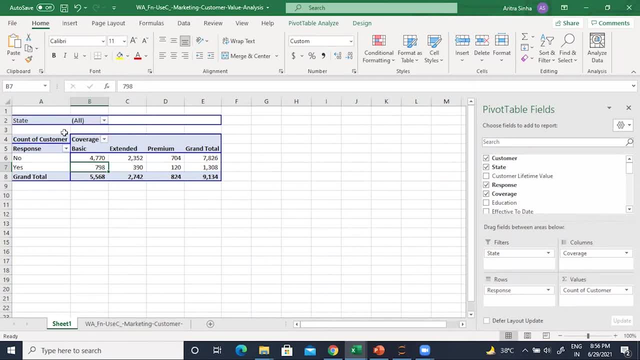 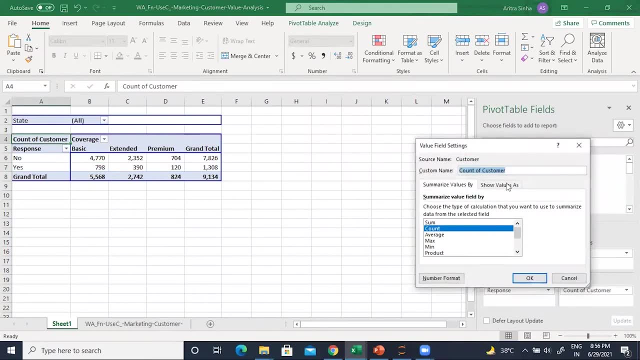 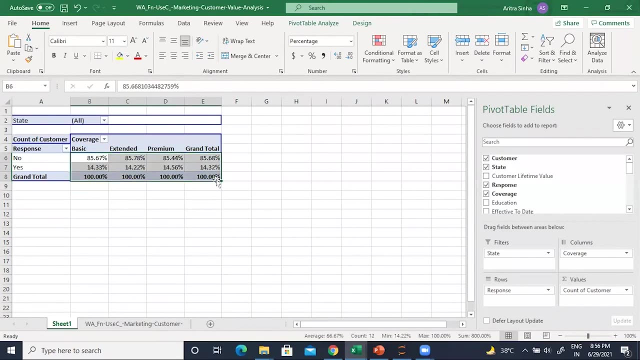 Okay, But if you want to find out the chance of responses, so let me just double click on this and show values as percentage of columns. We can now see that. what's the overall response rate? right? So 14% is the overall response rate. 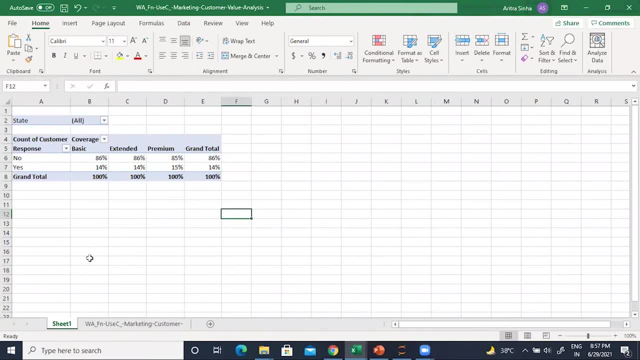 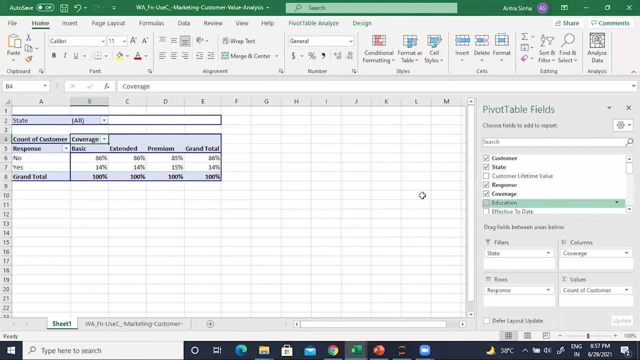 It doesn't really change. So by coverage, whatever coverage you choose, right response rate, chance of response doesn't really change. So by coverage, Can all of you see what's happening here? Okay, Sorry, I was just drinking some water. 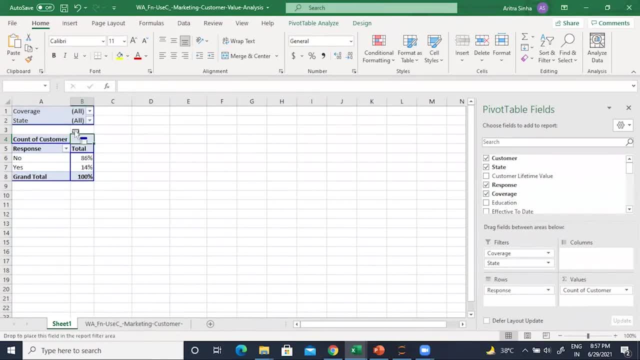 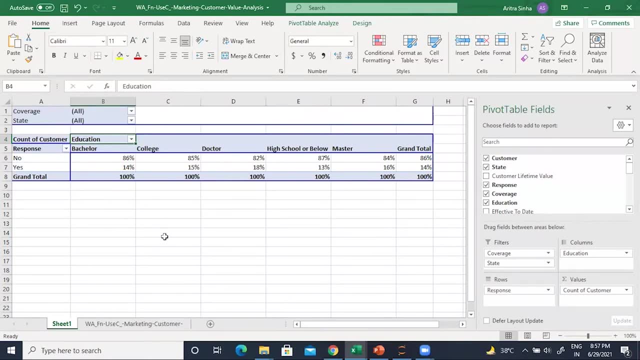 Now let's see for education. Does education make a difference? Education makes a difference. Some extent, right. We can see doctors are more likely to renew their laws, renew their policies. High school or below Somewhere. It's somewhat lower, but again, not a earth shattering difference, right? 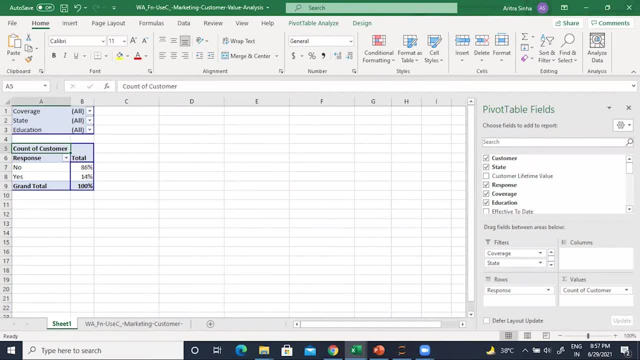 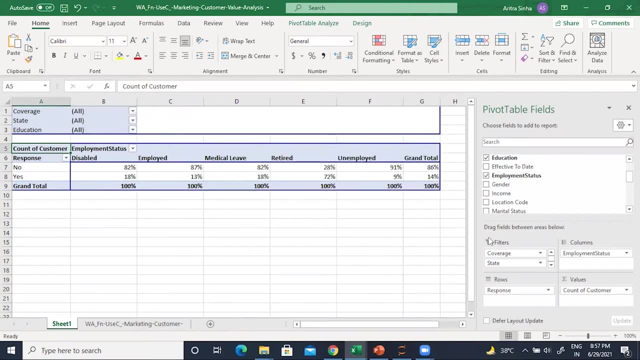 It's not like it's very, very stark as basically chance of success as compared to this. Now look at this. People who are retired seems like they are phenomenally higher. The chance of renewal is much, much higher. In fact, it's so much higher that it is like what? 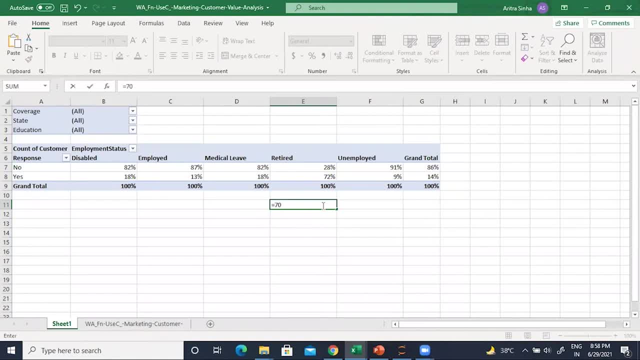 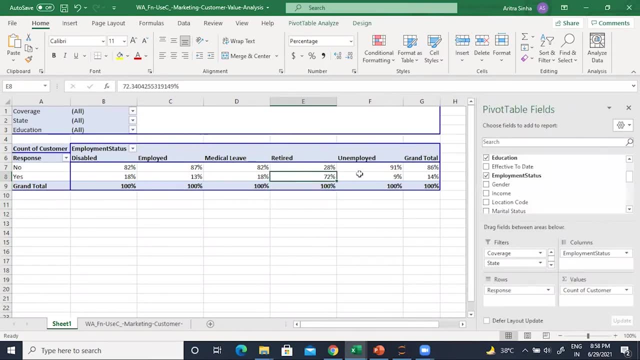 Five times higher, right. So 70 divided by 14,, five times higher. So it's five times more likely for the retired people to renew their loans. Now this is good insight, because employment status can potentially be a good predictor or discriminator. 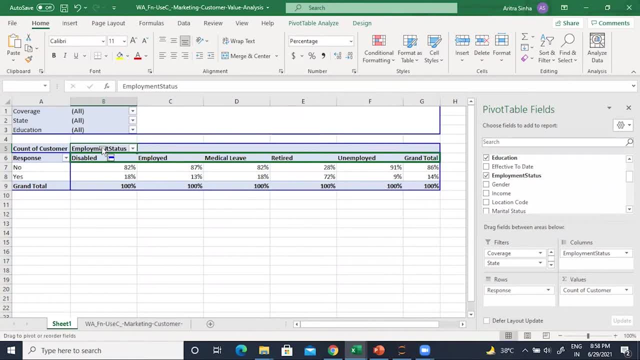 But yeah, this is not feature selection that we're doing in Excel. Of course, if we have to do this whole analysis in Excel, we could have done feature selection this way. But for the purpose of discussion today, where we're exploring the data, we are looking at, 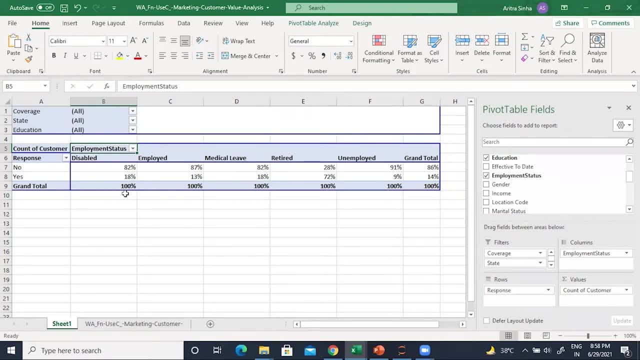 various features and their combination with the response variable. So yeah, we're exploring. So it looks like retired can help you, But of course we need to put this through a select K: best, et cetera, to see from a chi. 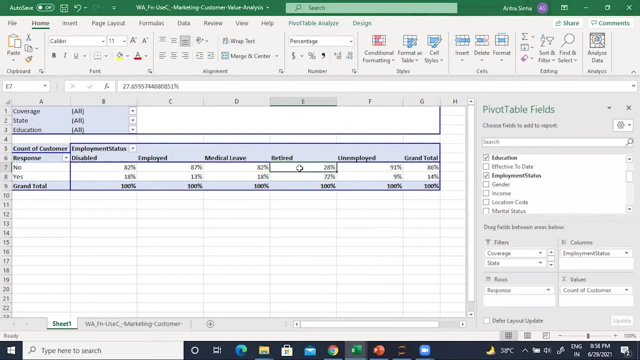 square perspective does it make sense? So is the difference between this and this statistically significant or not? So that is something select K best will do for us. But overall I think this has given us some clue that okay if the individual is retired. 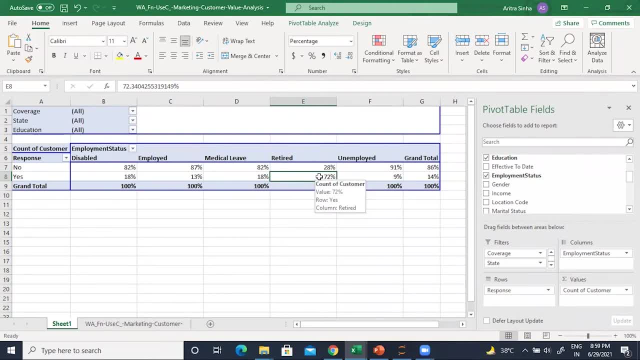 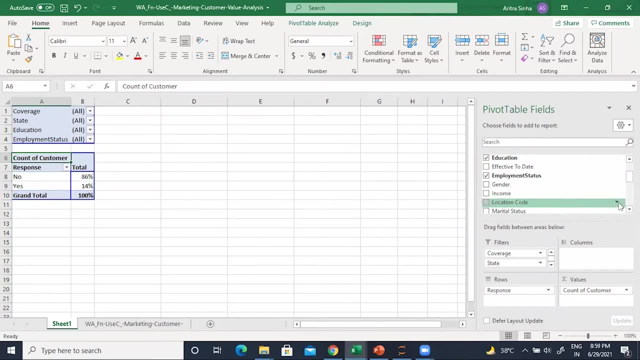 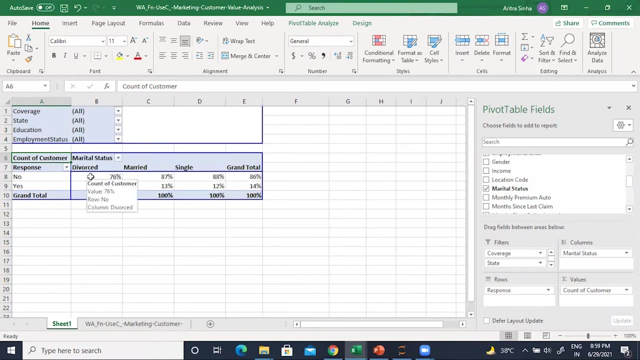 then chances are pretty high that renewal will probably happen. Okay, Now let's look at something like marital status. This actually becomes an important feature because- but very surprising that you know- this one is not showing any kind of I mean whether married or single. It was expected that for married individuals the renewal rates would be higher, but it's not the case For divorce. technically it turns out to be a little bit better. Monthly premium. Let's see How much is the monthly premium. 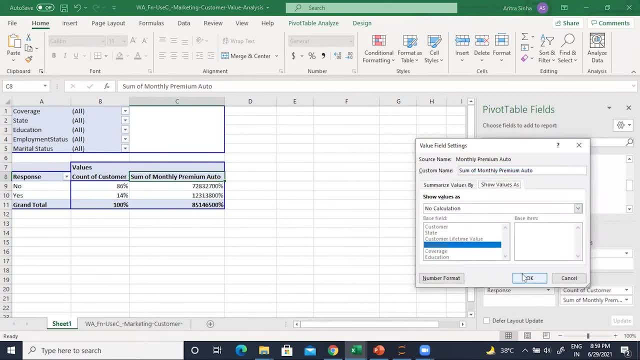 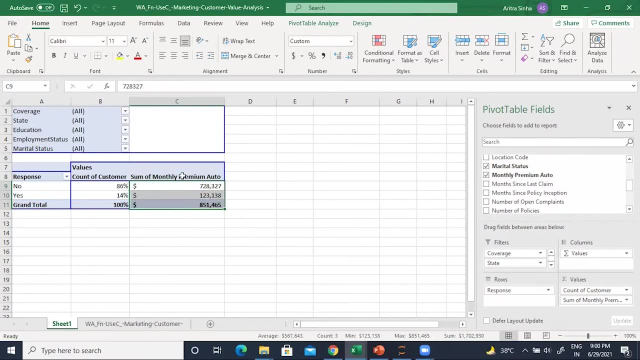 And this is again showing values as number. Okay, It's fine. So we just put it in dollar terms and take the average, because we are interested in per customer. So if you look at the numbers- right, if you look at these numbers, then you can see. 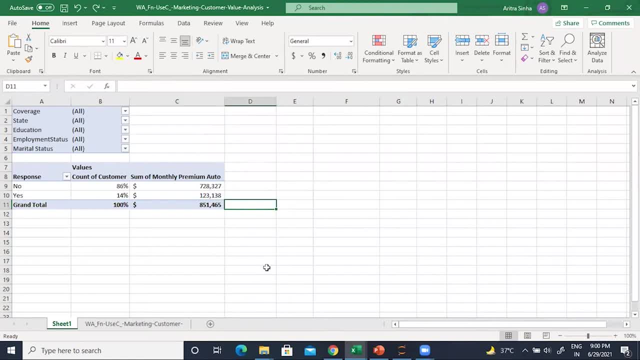 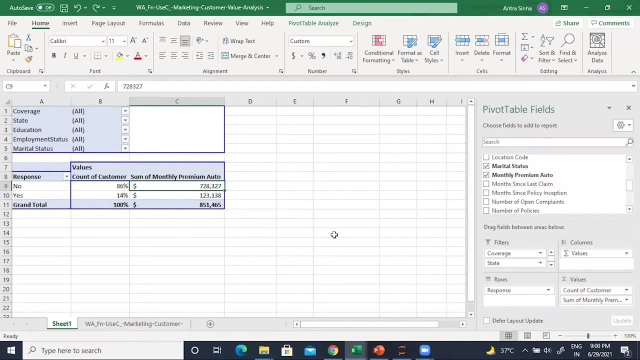 if you might. okay, this is an example of. I want all of you to pay attention. Look at this number: Sum of premium. What do you see? that people paying a higher premium. the chance of response goes down. right, What? how would you interpret this? 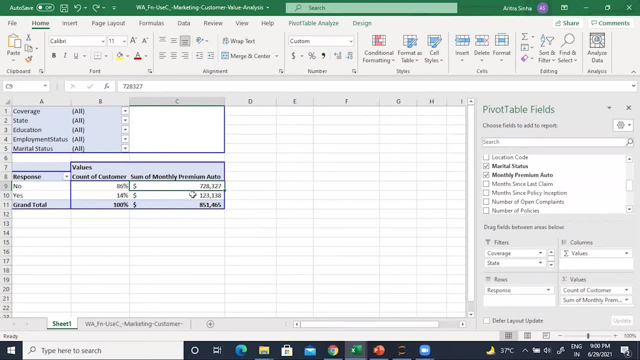 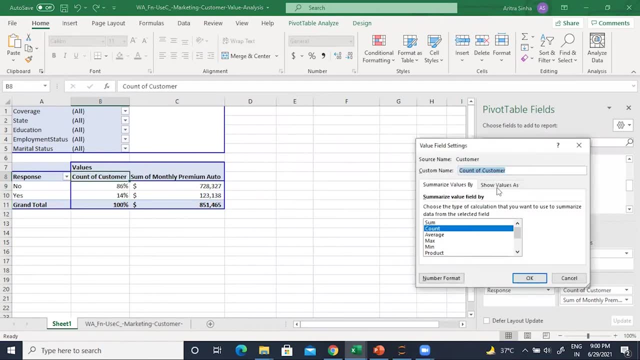 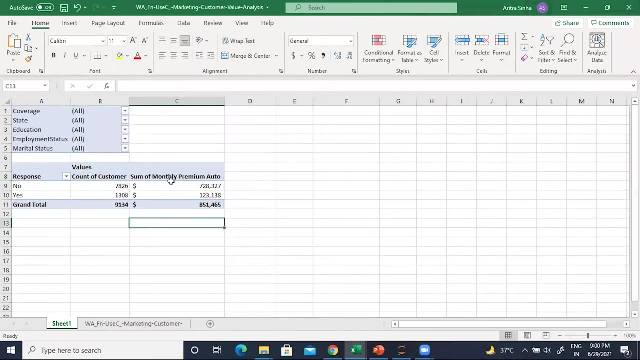 This particular stuff, guys. How would you interpret this? How would you interpret this? Actually, this, this is data interpretation question. okay, so how do you want to interpret this? is there any difference? like, if, uh, people who are responding to a renewal offer, uh, are they very different from a premium perspective or not? 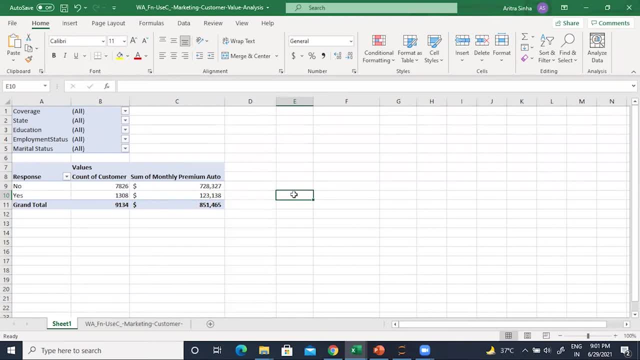 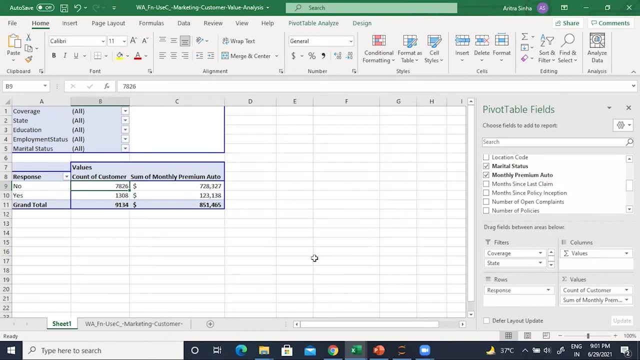 yeah, you are looking at this number. can you also look at this number? uh, this is very critical, everybody. uh, so it is not enough to look at just this number and make a decision. okay, whenever you're looking at data, right, yeah, always see what is the, what's the? 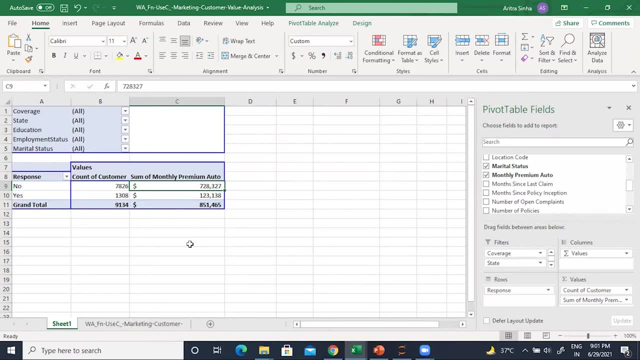 size of basically how many observations are contributing to that number? so 7 826 customers are contributing to a total market share of 7 826 customers. monthly premium: 7, 28 327.. now these guys- seven, eight, eight, two, six people- have not responded. 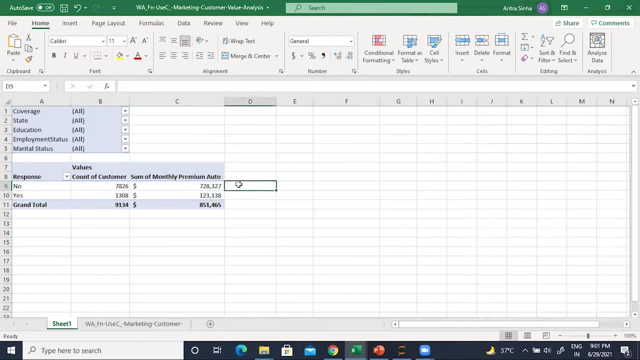 so on an average, what has happened here is that this is the average number, right? that on an average i mean, if you take a, if you take basically take per customer basis, then that's the total number of, uh, total amount of premium that has come. so 93 bucks has come from one single customer who. 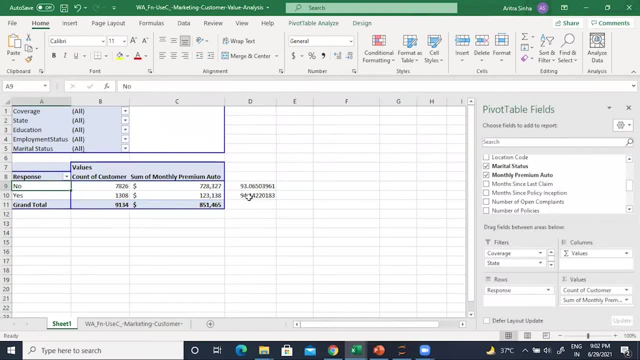 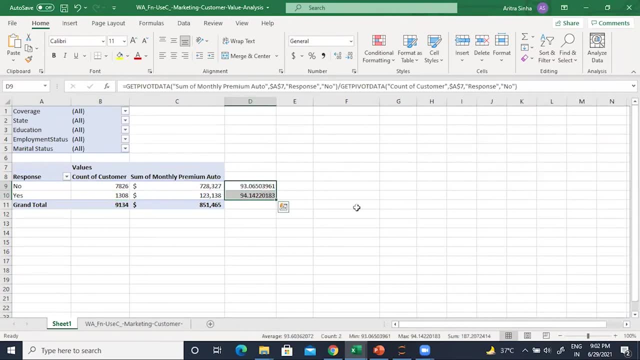 has not responded. as a monthly premium, 94 bucks has come from people who have, uh, i mean, on an average people who have responded. so there is no difference between, um, these numbers not not much different. so monthly premium cannot be a determinant for you to decide that. okay, you know these. people have higher monthly people. let's say, target them or no. so monthly premium cannot help you in targeting people for renewal policies, because average monthly premium does not differ is very clear. but here if we'll go with the cabins um analysis right, so it could have give a good. 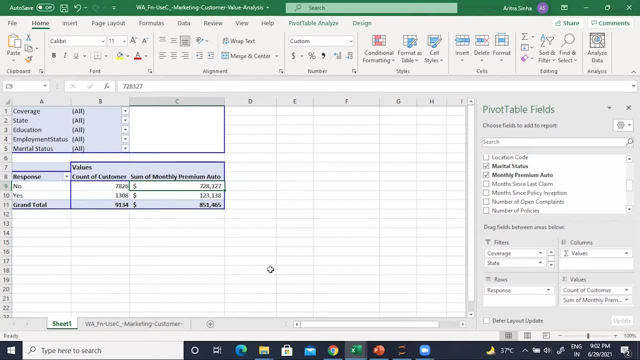 variable, saying that monthly premium is a good variable to include. but this is kind of an custom field that we have to create right to look at that. okay, you have to check with the count of customer, then monthly premium, um, so, when we do, no, no, so. so so here is then let's just do it. 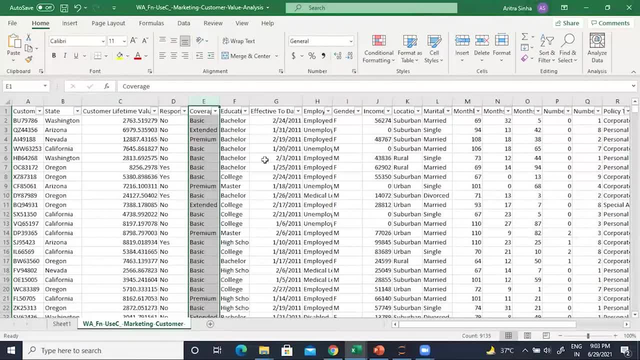 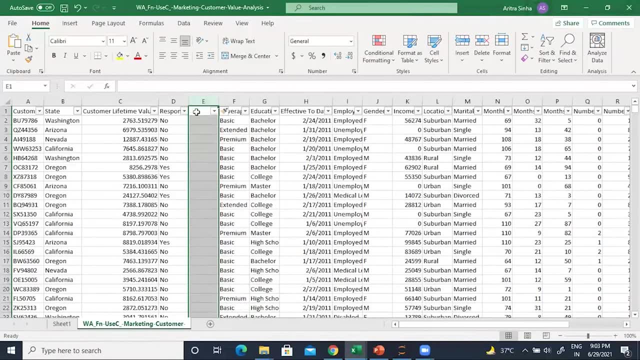 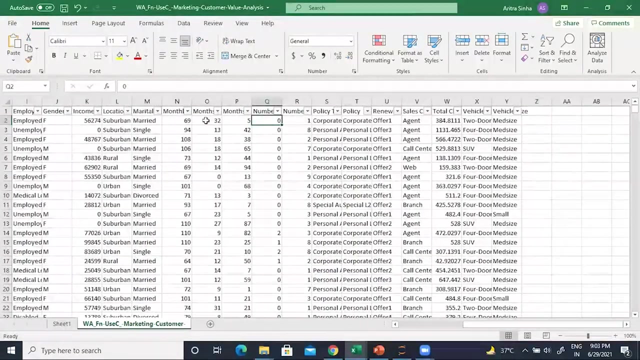 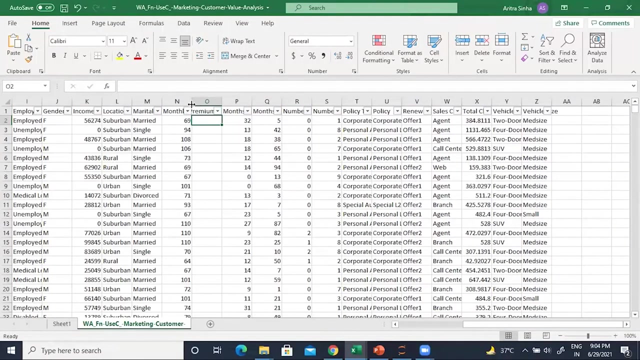 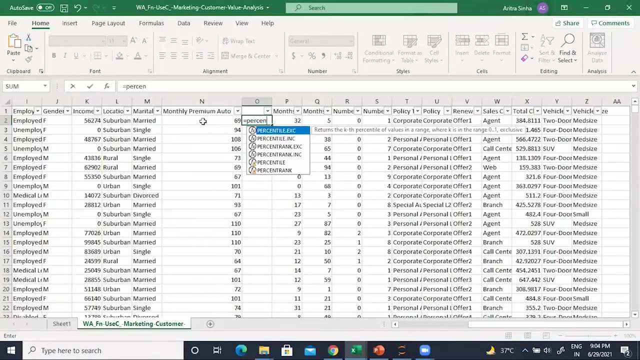 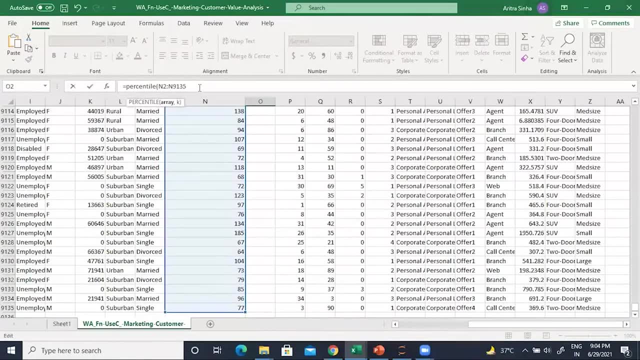 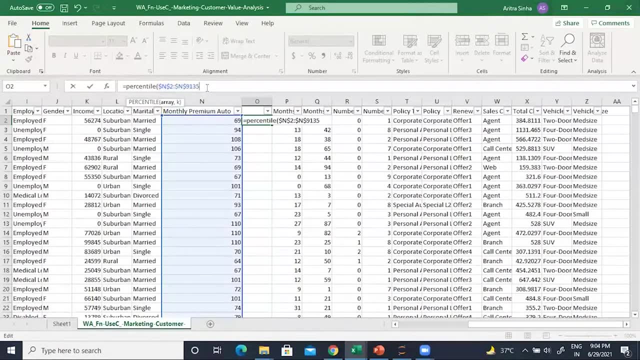 okay, let's do this. um, okay, i will try to do something like that. let me create a column called target. no, so zero one gets created. okay, average should be 14, something like that. yeah, it's there now, let's go to right now. um, um, so. 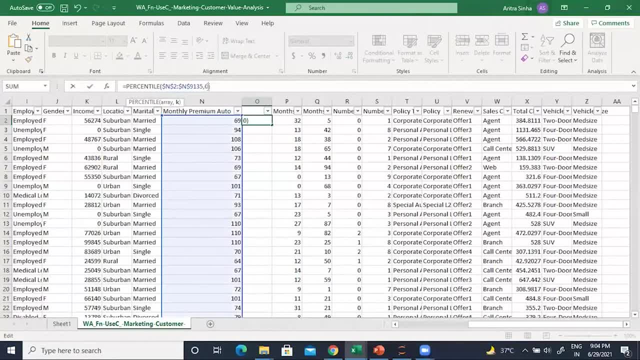 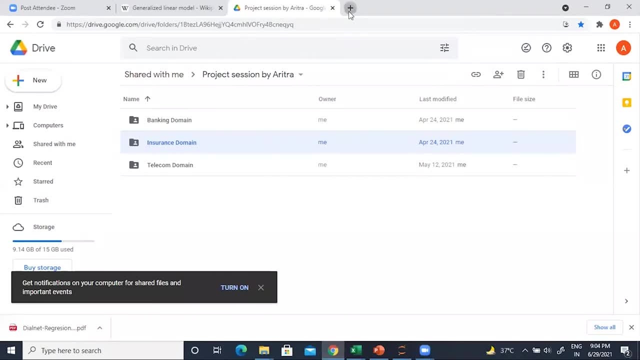 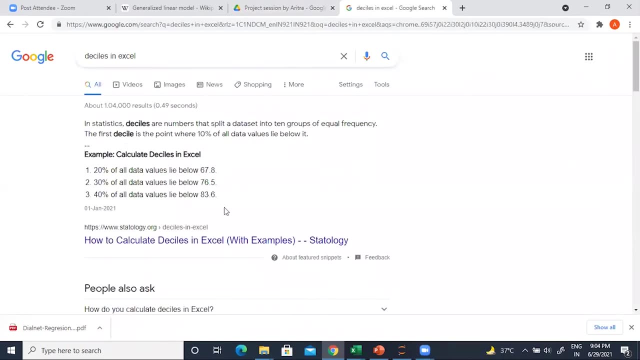 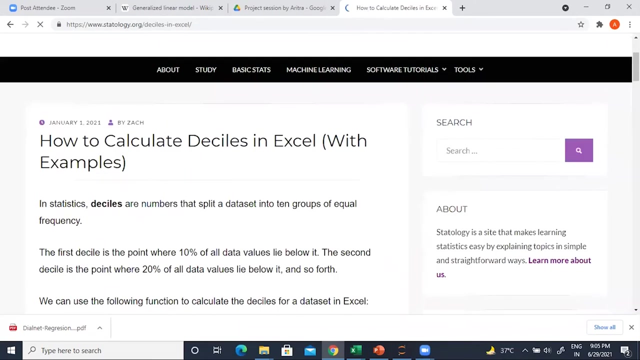 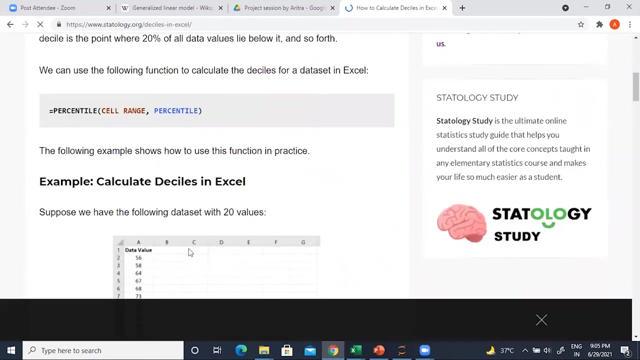 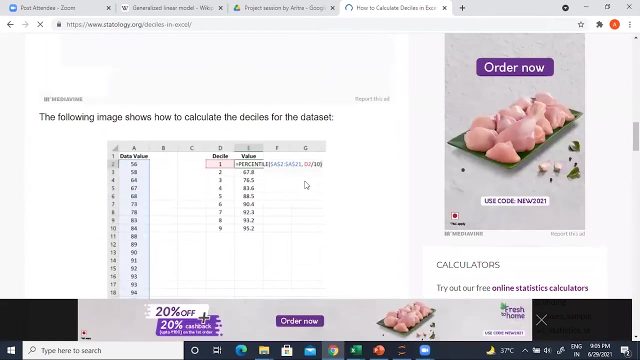 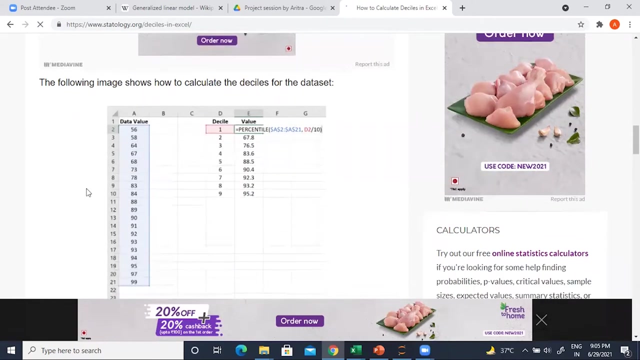 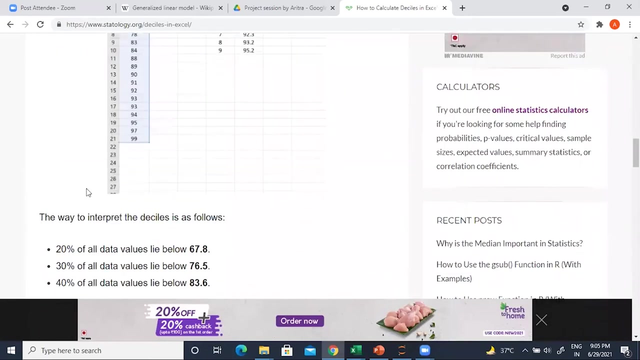 you see what that looks like. um, so, so this: i keep forgetting here how to do deciles in excel. allow me a moment. okay, let us find this out: percentile, cell range, percentile, that's what i did. equation 20: values here. okay, so okay, let's see. 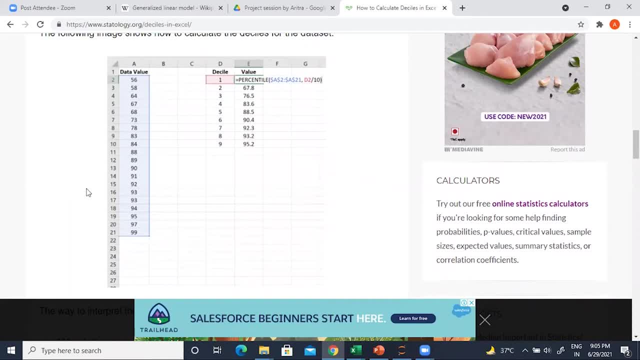 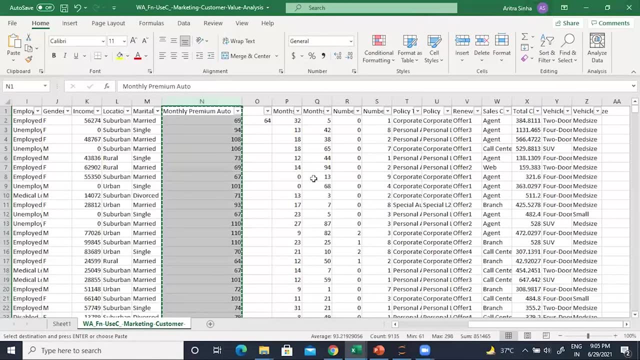 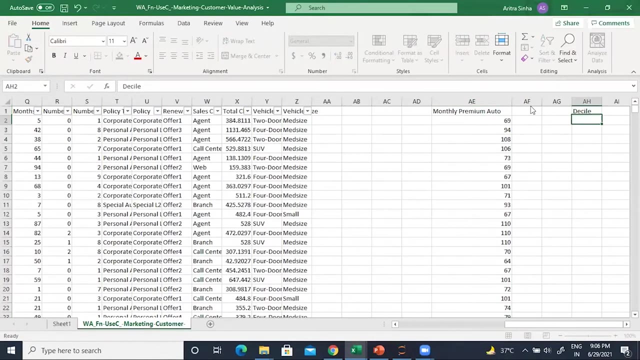 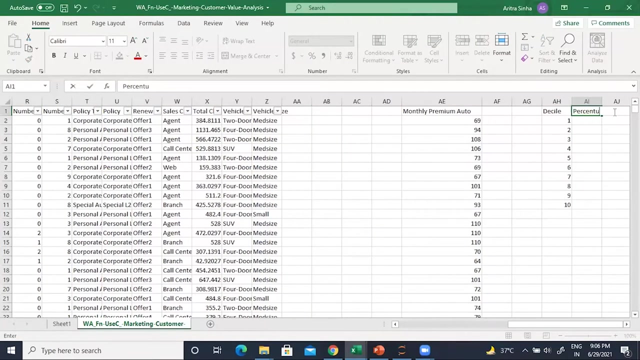 okay, so let us take this aside and let's create a column called design. okay, so let's see this one. so what we do is we create percentile for all these cases here, f4, fix it up and then we say this to happen: 10.. so this is 64. these are the cases. so how to set these cases. 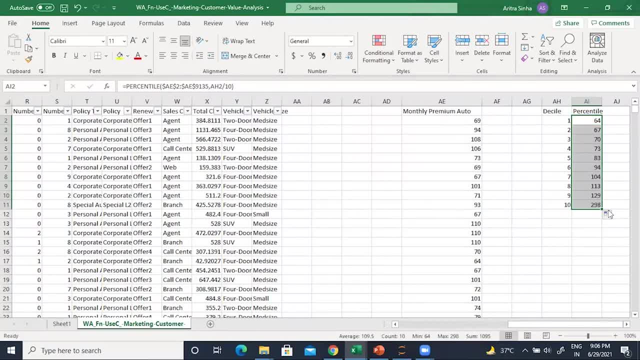 okay. so if we just create a column called design cutoff section, So if this one is less than or equal to this number, which is, then it becomes first assign. else, if, in a AND scenario, if this is greater than this and less than this, right, So we will have to say AE2 greater than AI2, which of course has to be. 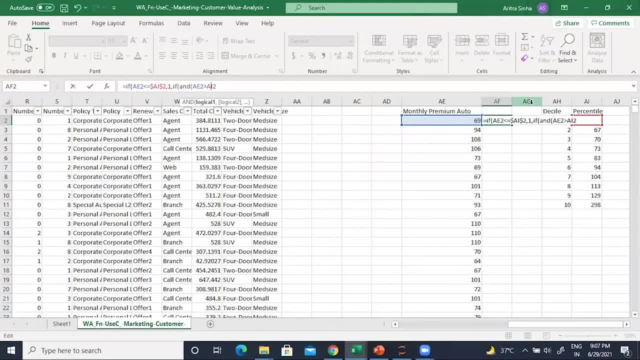 fixed Guys, bear with me a moment. okay, I'm trying to answer her question. actually, I hope it is okay with everyone. I'm sorry. I'm trying my best to answer the question. Did I catch your name correctly, the person who asked me the question? 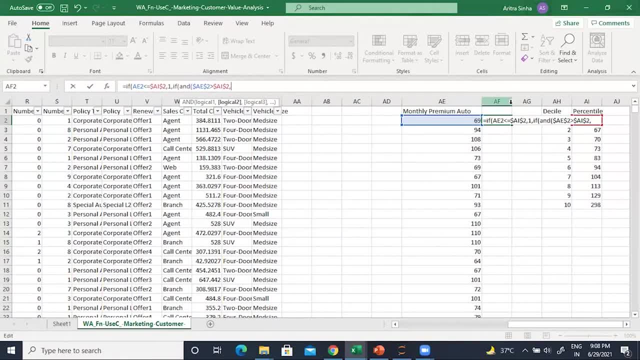 Yeah, I didn't get it. Yeah, it's okay. I mean it would take a time. then, yeah, No, no, no, just give me five minutes. Just take a minute. If AE2 greater than this one. wait, let me create some space here. Actually, I'm not able to figure out the columns. 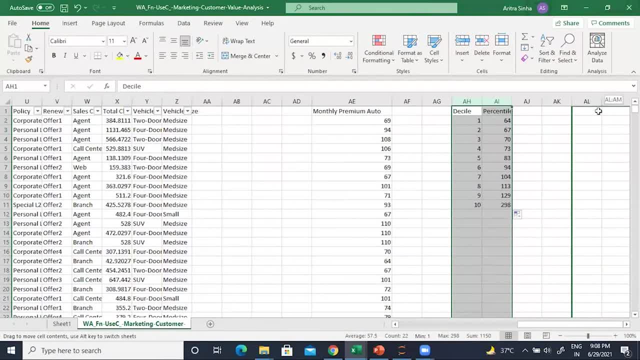 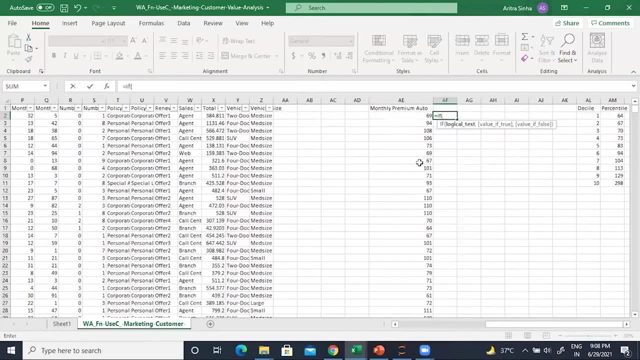 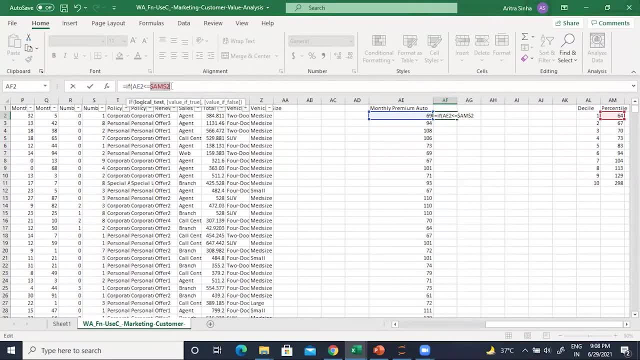 if it works. so all of us is in this sign. okay, we can see only thousand observations are going to and it is fine, which is making sense. so now another if condition will come in and bracket open same thing: a 2. this time it is greater than actually. why am i even doing this? 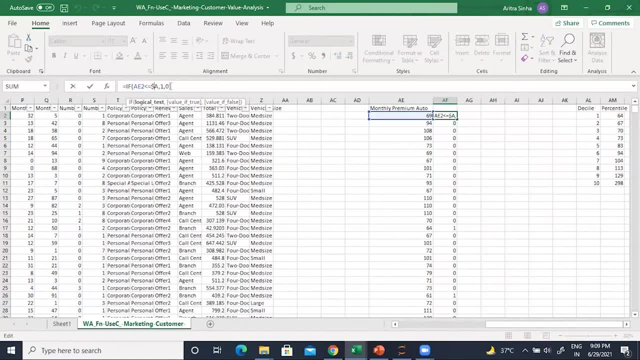 right, I don't have to write all these statements, just directly say: it is definitely 64, then one. if and a 2 is greater than 64 comma, a 2 less than equal to 67, then I give it to greater than 67 comma created. 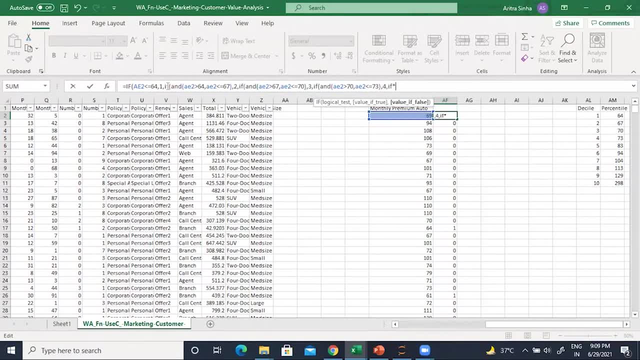 and sport, then you can use this template. then you can use this template. you can use this template later on. also, if you want to do this kind of analysis in excel, i'll be sharing this template today, will i don't know if you guys would like to have it. 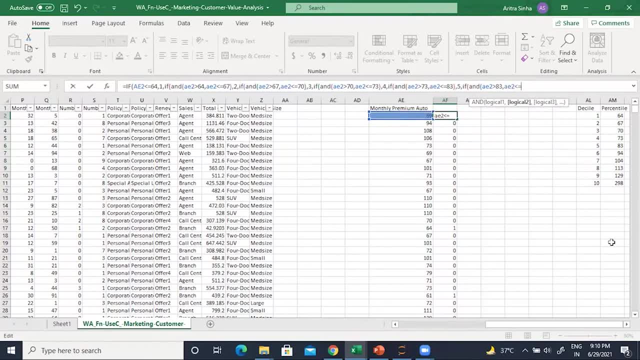 so, uh, instead of anybody has any questions at the meantime, i can answer while we are doing this. nope, all right, no worries you? uh, this becomes a challenge. i think i must have made some mistake in the formula in a rush to do it. in these situations, guys, it's always good to go to your good friend notepad and keep a copy of. 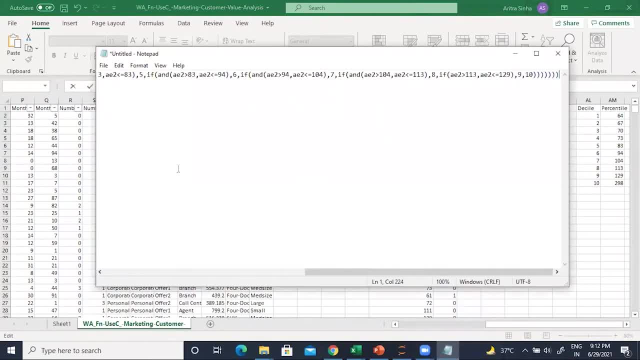 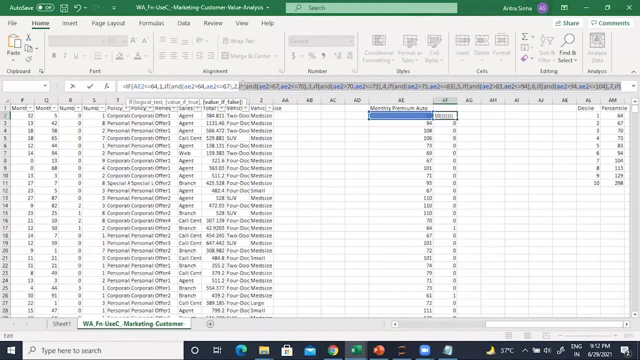 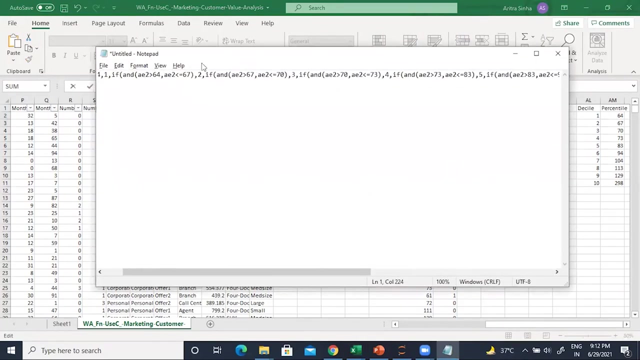 these cases or formula, right? you don't want to be writing it again and again. now let me see what went wrong here. if i want to do one and two, yeah, then this was working. then what happened in excuse treatment? uh, we have not written end, i guess. 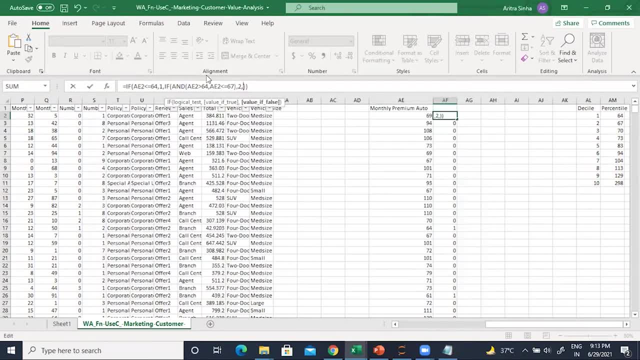 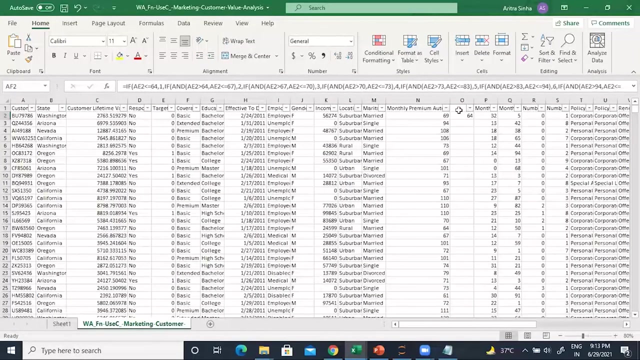 yeah, you're brilliant, right, absolutely right, and that is where it has become a problem. come on, okay. oh, thank god, thank you so much for helping out here. all right, so let's do a look up. let's do a look up up. okay, if you want to work like this in excel, you can pretty much do your bivariate analysis like. 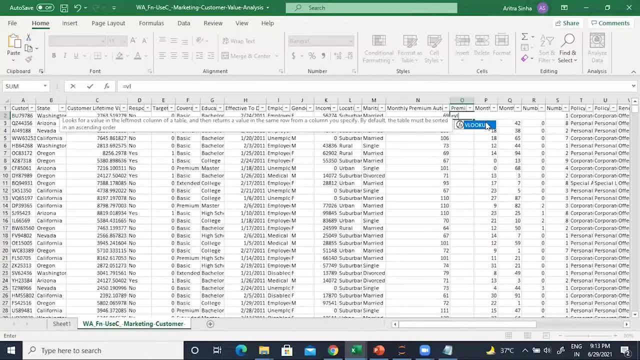 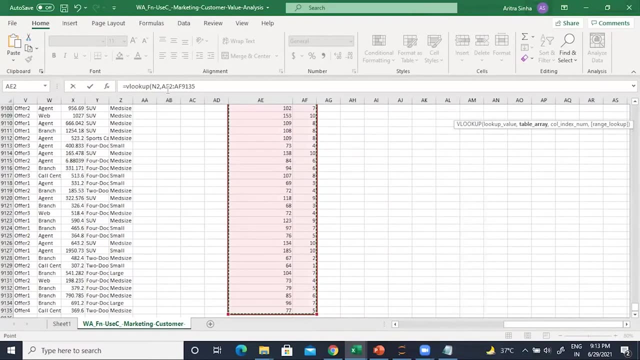 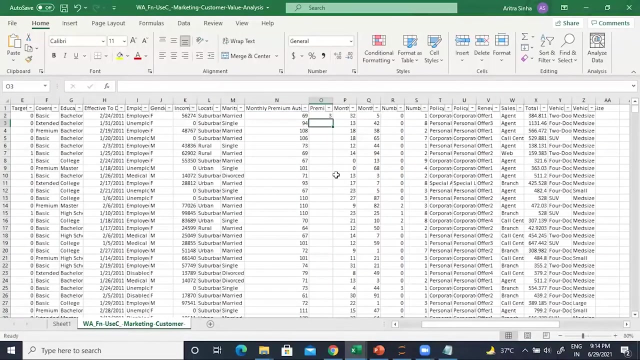 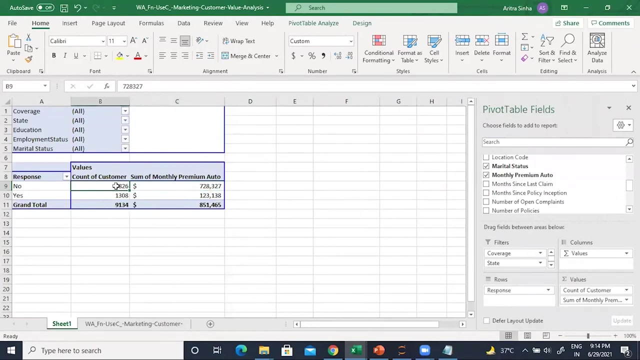 this. in fact, if you guys are interested, i i am more than happy to show you how you can use excel for classification problems. if you guys are interested, let me know. would you be open to learning how to do scoring, classification, modeling or some? yeah, you can achieve the same objective using excel. also, let me know if that makes sense. okay, so now? uh, let's see. 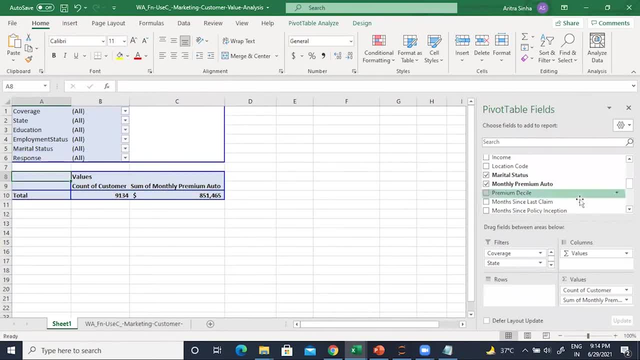 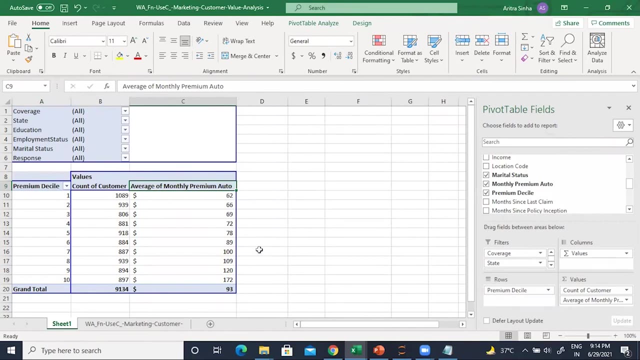 we move this and we bring it here. come on now. yep, pretty much the same premium. okay, now we're supposed to take average premium, so that will change, okay, yeah. oh yeah, it has to be same because ultimately you're pretty much the same number of customers getting captured, so desires are fine. uh, in python, of course it can. 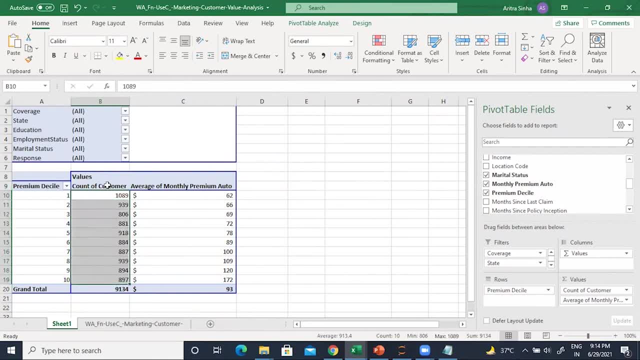 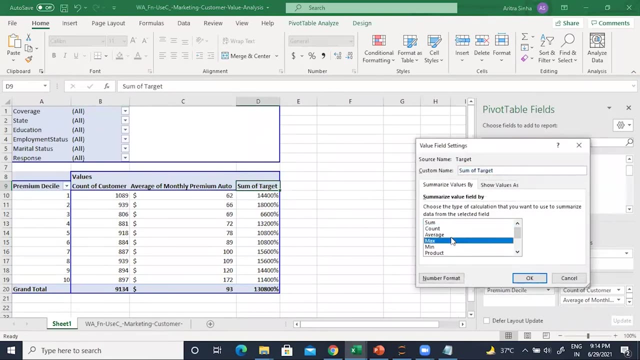 be a little bit different here and there. some, uh, some changes can happen, but if i take this out for now, okay, i am interested to get the target. yeah, 3d, 4d, 5d, 6d, 7d, 8d, 9d. 10d, 11d, 12d, 13d, 14d, 13d, 14d, 15.. 22, 23, 24, 25, 26, 27, 28, 29, 30, 31, 32, 32, 33, 33. 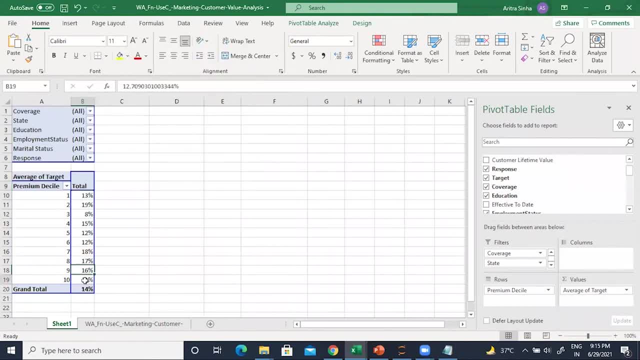 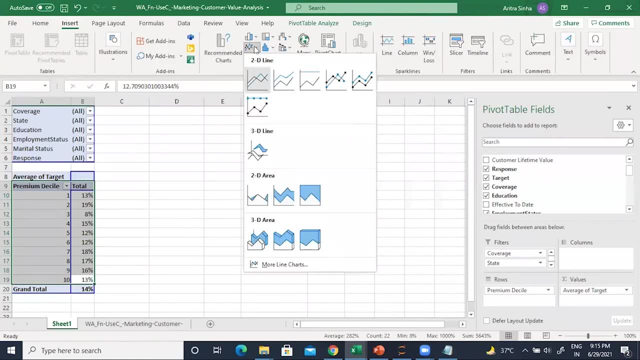 34, 35, 34, 35, 36, 37, 38, 37, 38, 38, 38, 39, 40, 41, 42, 43, 43, 44, 46, 47, 47, 48. so i just want to mention here is that there's a lot of things in there to do with this. 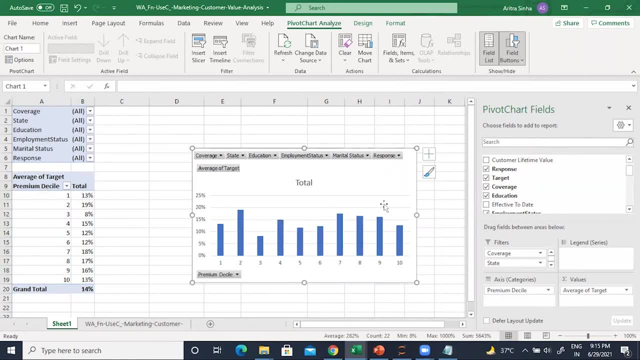 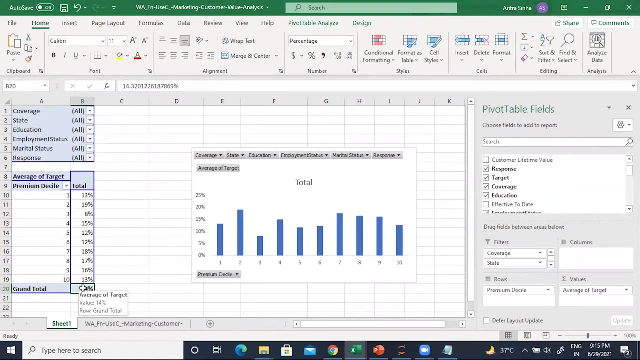 how does this graph look? does it look good for a finger predictive purpose? not that good, no, yeah. no, i mean like, look it is. there is no discrimination because ultimately, 14 is the rate of success, right? so there is no premium bucket where you are superbly higher than 14. 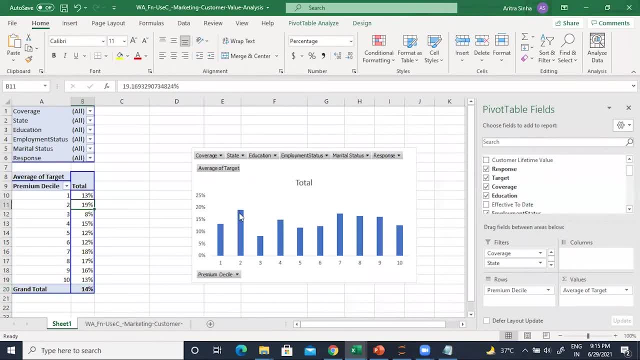 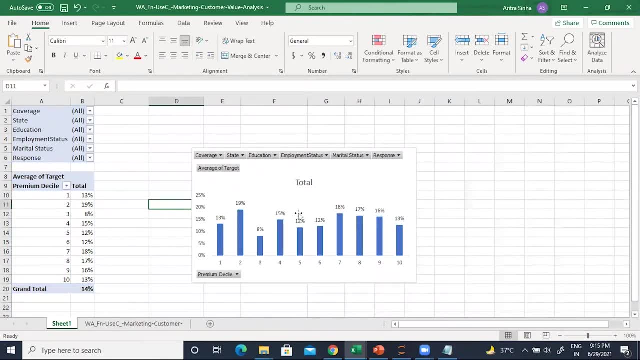 except for this part somewhat higher, this one- if you do data labels, the add data, you can clearly see 14 is the average event rate. so in no, no such case where it is much higher and there is also no uh slope or discrimination that is shown by this variable. 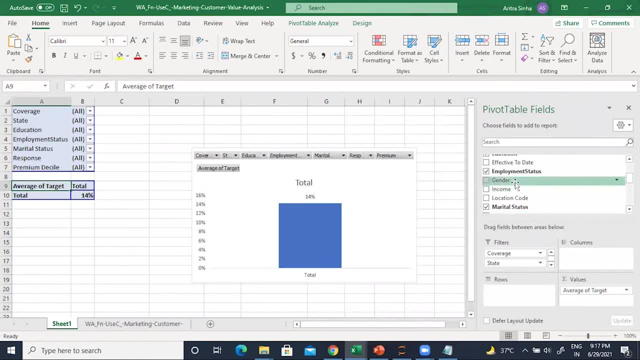 okay, we now have the target variable as well. let's bring in gender again. gender seems like a again gender. not good predictor. you can see we're bringing gender here. see 14, not not very different from each other. um, this is, these are two. uh, you can see that gap here is 14.17 versus 14.48. 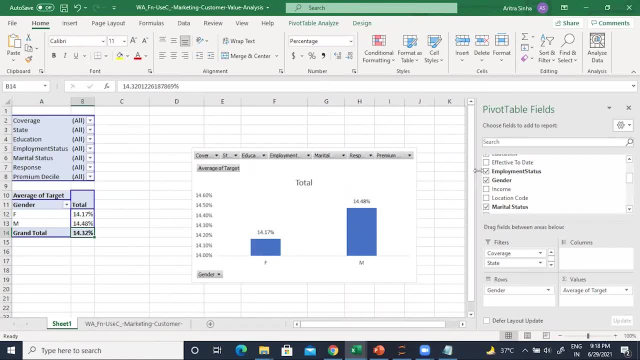 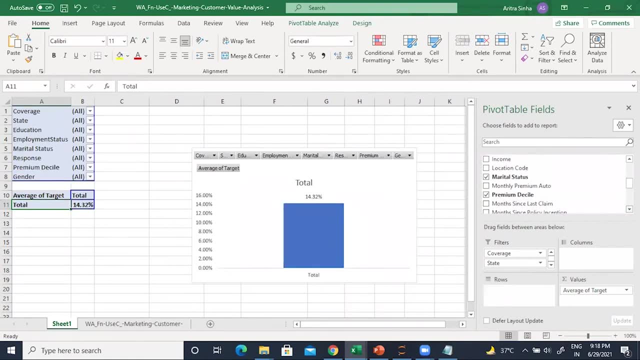 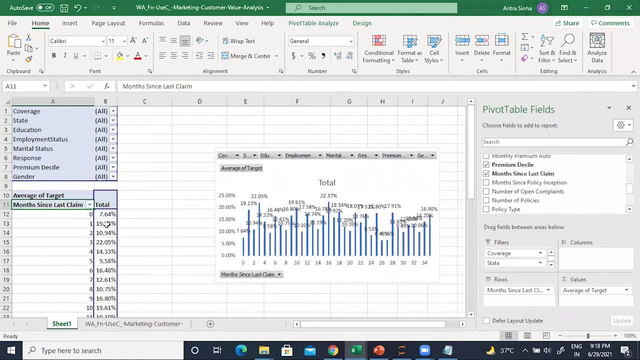 that's why is a little bit of gap, but overall there is not a lot of cap, right, so gender is again not very promising for now. then what is it that we are looking at? months since last claim? okay, months since last claim, because it's a continuous variable. we can't actually use this as a categorical 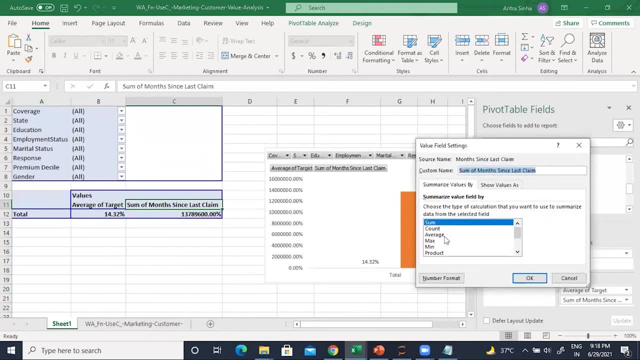 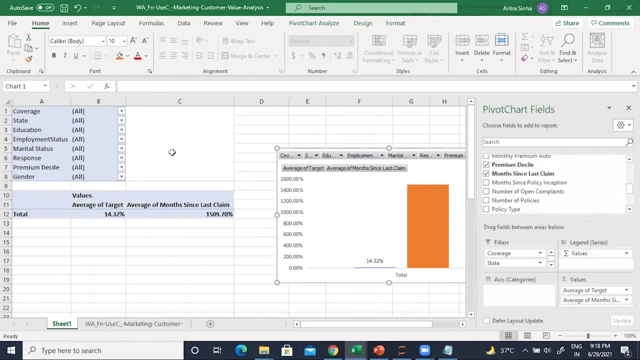 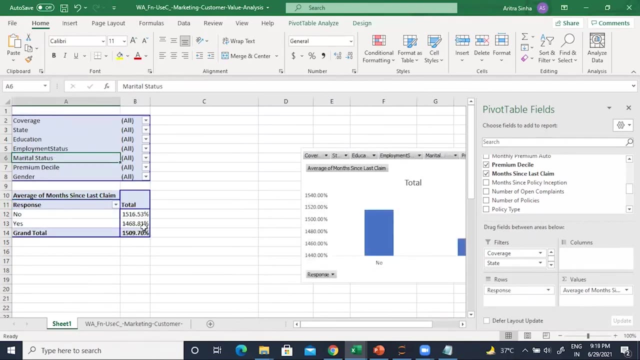 what we're going to do is we are going to have looks like this, like this: we are going to have have average month since last name. okay, we can get rid of the graph if required, or maybe remove the target here. bring in response yes or no. so here we can see that month since last. 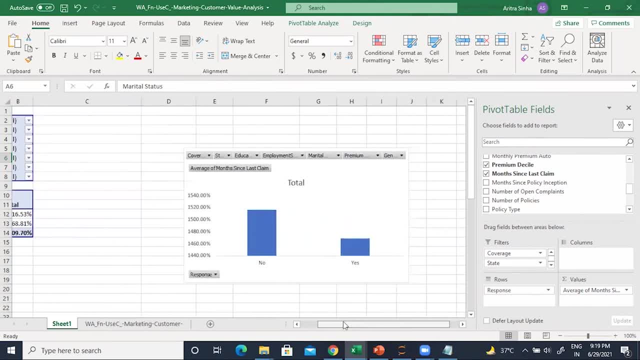 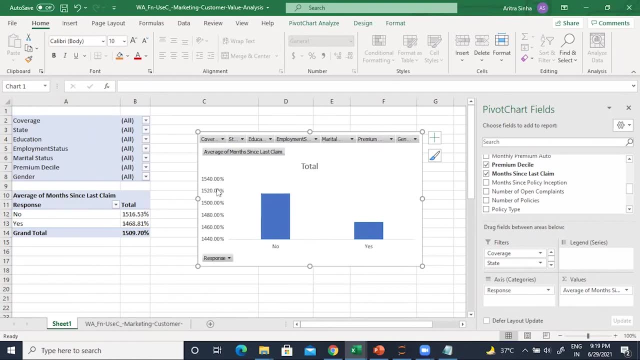 name, um, but the more i mean the if, if the time has, if, if, if it has been a long time since the claim has been made by the customer, then chances are higher that the individual, uh, might actually respond. okay, so how? how many months since last name? so some some changes here. so 14 months. 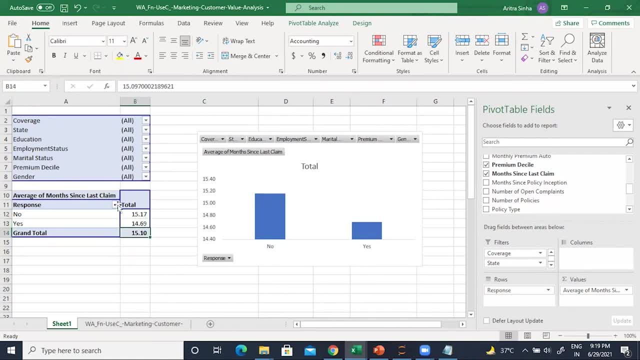 on an average, 15 months is the uh month since last claim made. but people have responded. they've you know, they've also claimed recently. so it's good, it goes, it is logical and it is very intuitive because it means that the customer is happy. when the claim was made, the money was given out and the 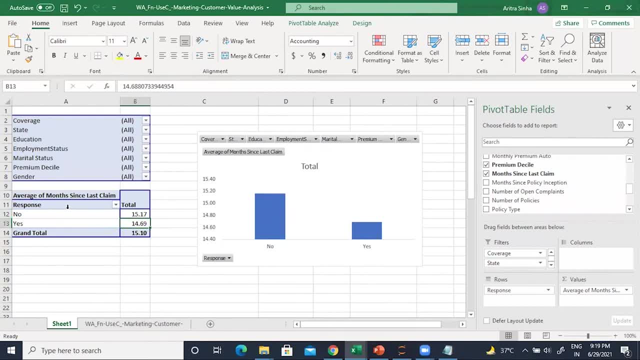 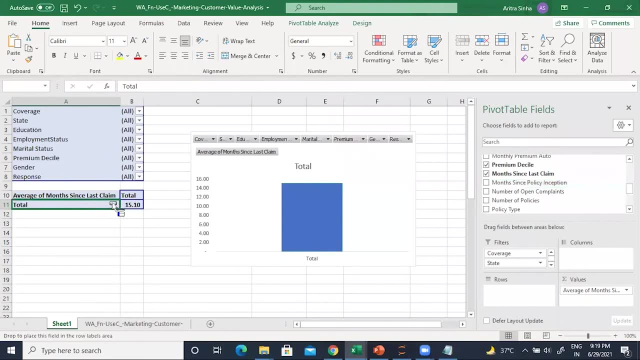 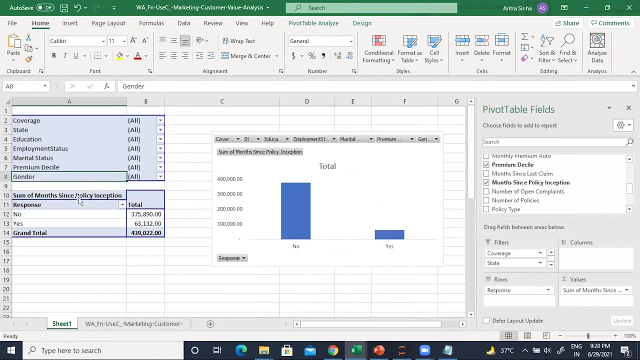 customer was pretty happy, so they actually are more likely to renew their portfolio, renew their. you know the policy now, month since policy inception, how much time has it been since you are a customer? so that is the metric here. so let's see, month since policy inception it will. 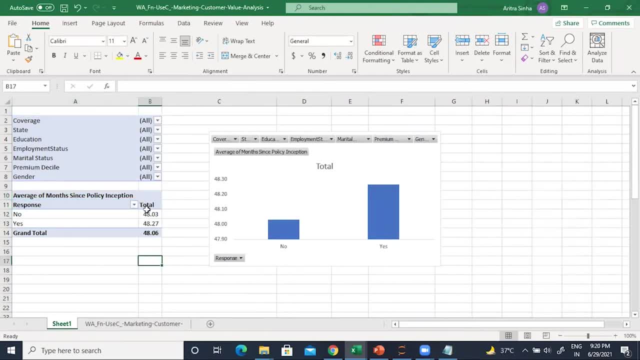 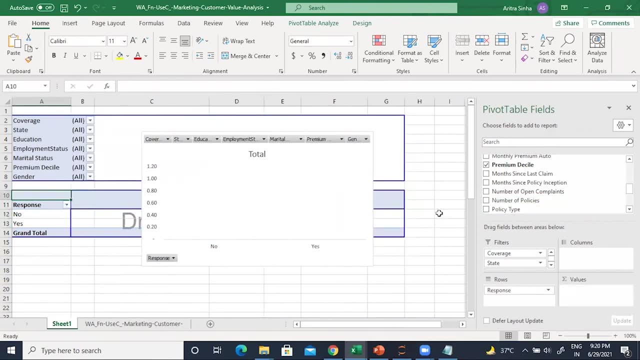 again, we have to take the average. it is not very different, right? 48, 40, uh, 10 year is not playing that much of a role. number of, let us get rid of the number of open complaints. this should be. yep, see, you can see it here, right? 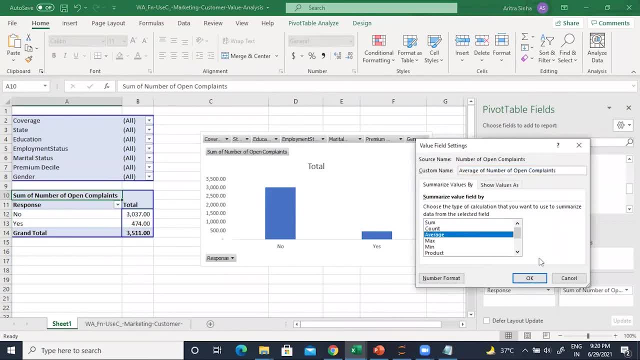 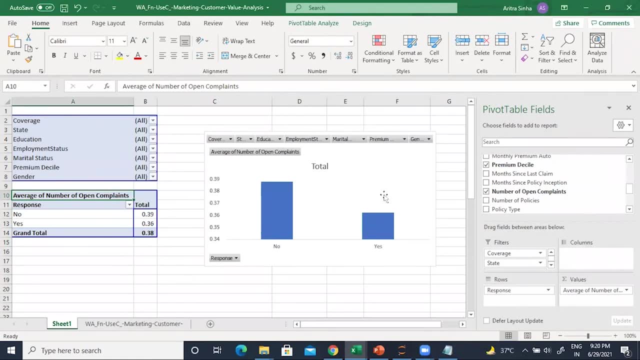 uh, number of open complaints. this actually should make a difference. the number of open complaints, uh, i mean, is lower in case of people who are people who have responded, versus people who have not responded. if you take a sum of number of open complaints, you see the 474 complaints are coming. 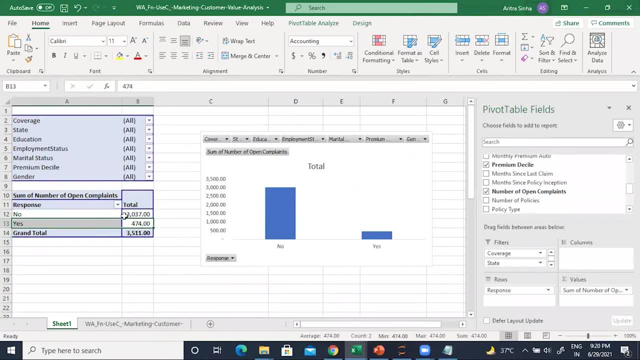 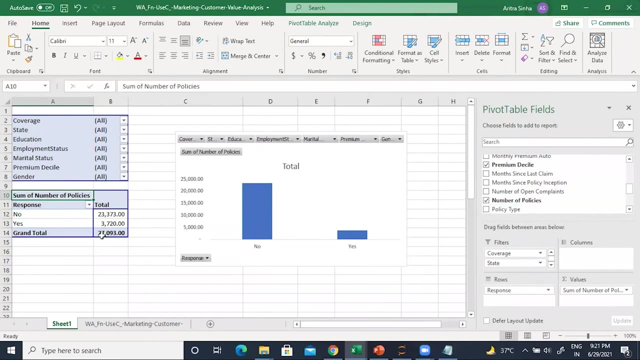 from people who have responded. i mean only 474 versus. if there are a lot of complaints, of course, this- this is again intuitive, because if customer is happy, then they will come back and take your services again. okay, number of policies. uh, oh, it shows the total number of policies here, which is again lower number of policies. 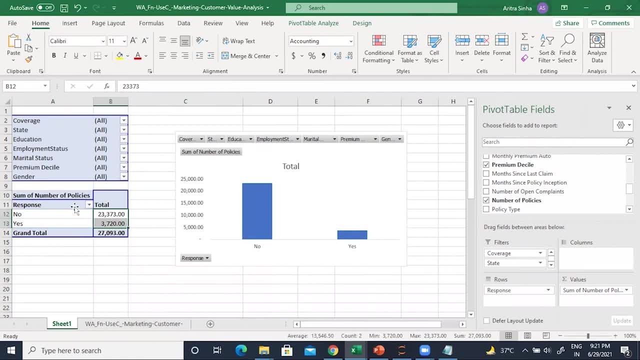 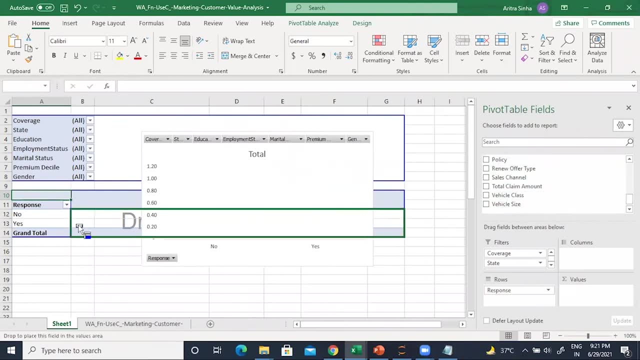 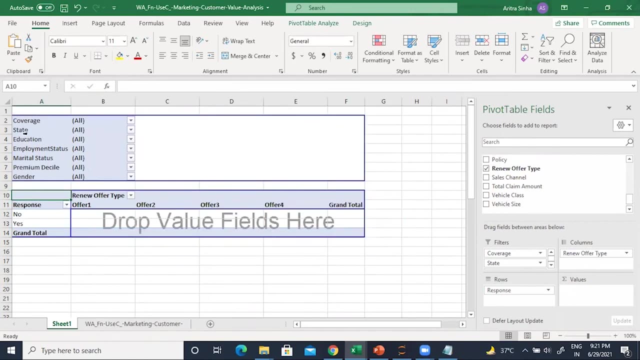 this can actually. this can also be good in terms of predicting chance of responses. what else does it have? renewal offer type? yeah, this can be interesting. let's have a look. um, let's get rid of the graph, let's bring in the number of customers, okay. so what do we see? we see that out of time, one, three, four. 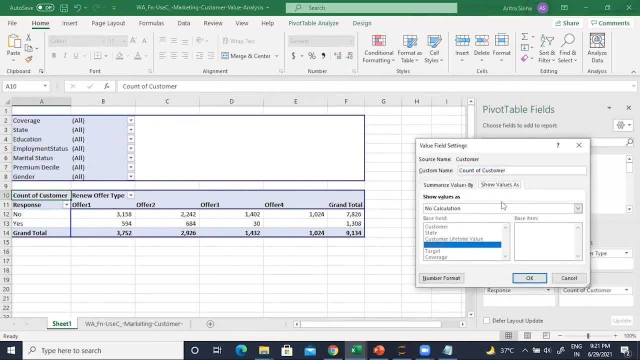 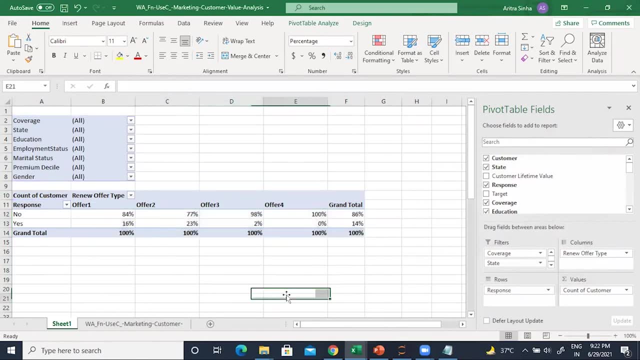 chance of. let's have a look. let's express these as percentages of columns. can you see how i'm using excel for deriving insights? uh, is something, is this something that you guys normally do, or is this completely new for a lot of people? you would want, uh. 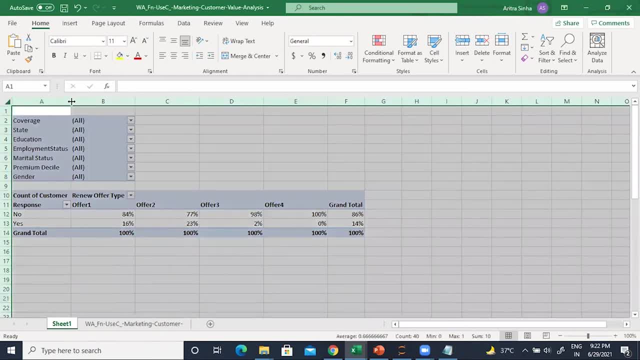 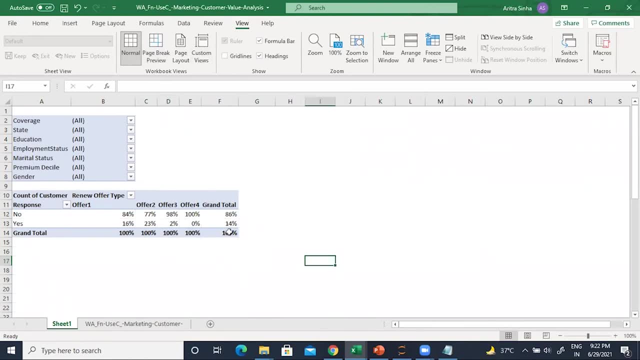 training and guidance on this. can i know, uh, what is this scenario? this is something, something new. i hope you're enjoying what is happening like it's it's. it's not, uh, using any program per se or any programming language, but um, merely using excel. but can you? 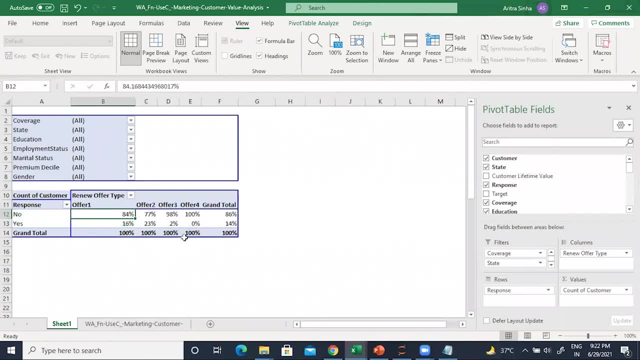 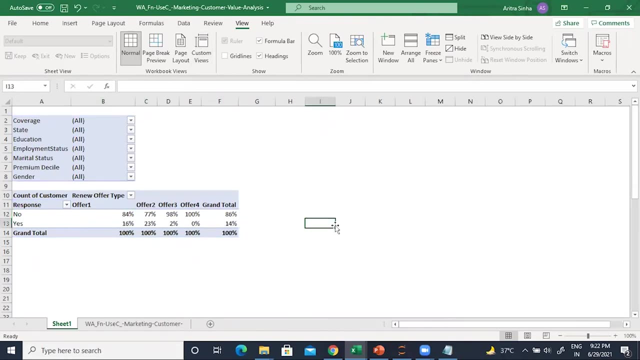 see the power of excel right in a very short amount of time. you're getting an overall good sense of the data. um, so would you like me to put together a project in which i use excel and solve a classification problem? um, there's a separate kind of modeling, called heuristic modeling, that can be done on excel. 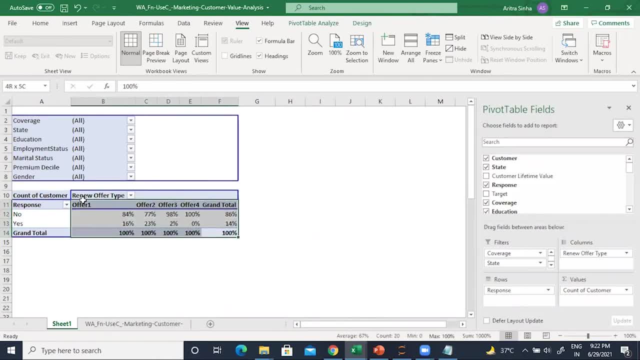 um, but it involves bivariate analysis and it involves finding out variable cutoffs and applying those variable cutoffs. if you would like to let apurva know and i can take that to you, okay, uh, offer two. there's something about offer two. people like more of offer two you make. 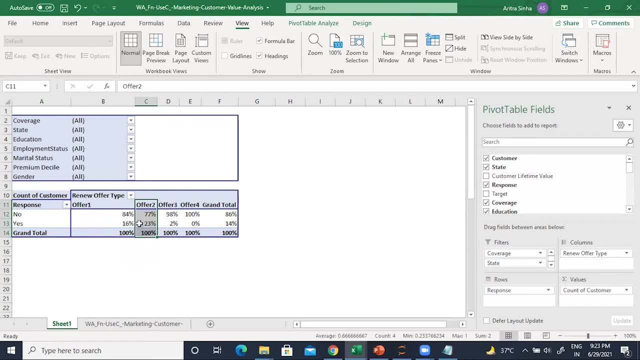 offer two, people like um, almost like double the chance of responses. uh offer one is also not bad percent, but offer three and four are not liked by customers pretty much because majority of people who have been offered uh offered three and four out of 100, 98 never responded in offer three. 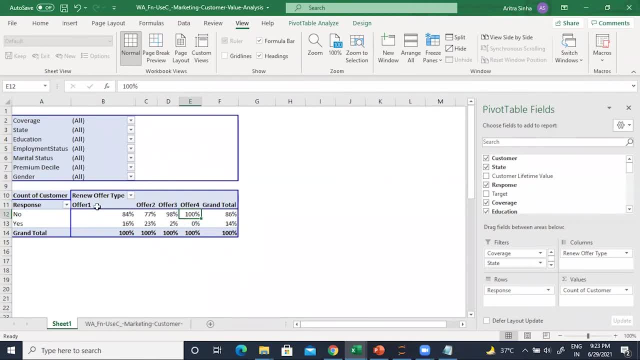 and nobody liked offer four. so three and four are clearly not working. one and two are working. two is the best, followed by one, then three and then four. three and four are equally bad, but uh, two is the best, followed by one, make sense. so, yes, similarly, let's look at which sales channel is good sales channel. 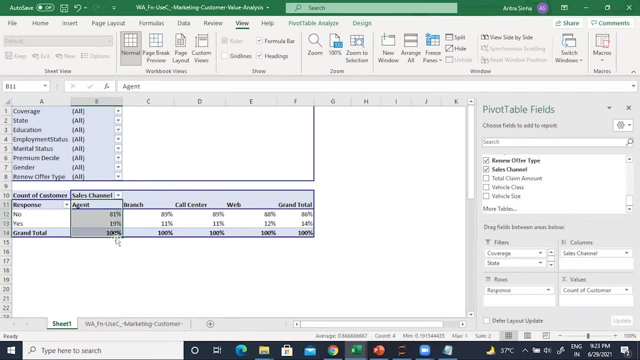 agency agents are always going to be good. human to human touch makes makes a lot of sense. call center: you know how many times do i like it when policy, because i called me, i don't like it too much. call center: uh web or all the advertisements. unless and until i'm really looking for something, it might not actually help me renew the uh. 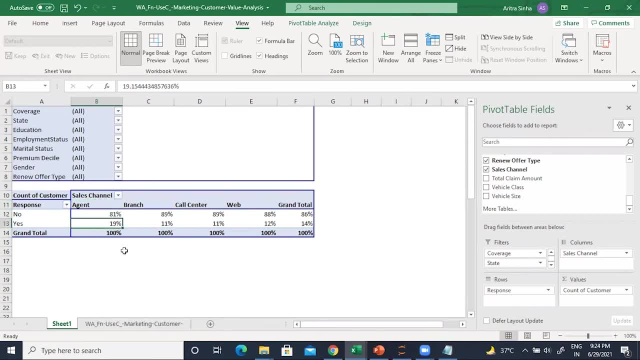 policy. so agents are slightly more effective in terms of nineteen percent probability. overall you have fourteen percent right. other than other than agent, pretty much all of them. they bring down the probability of success even from fourteen percent right. it's all eleven at two and so agent is uh standing out. so if you have a one hot one hot encoding for agent, that can. 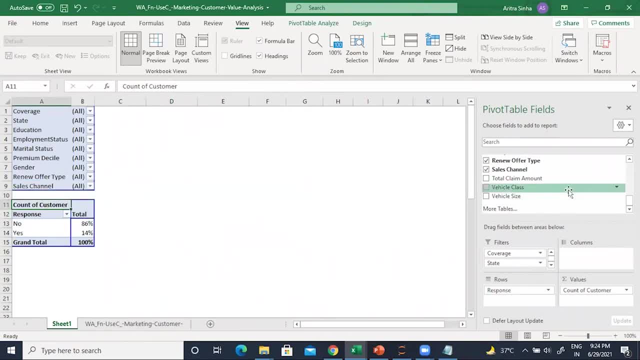 be a good uh predictor, but not a very powerful predictor, but still a good predictor. uh, wicked class. let's see what kind of things are. so here's the thing. right, if your car is super expensive, you would ideally want uh it to be insured as much as possible. so i mean, you would kind of stick to the same insurance. 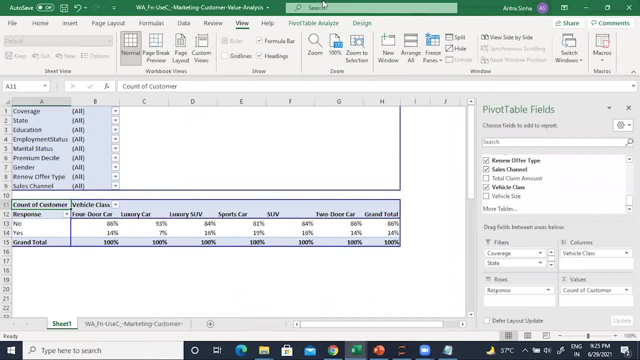 because i, if you, especially if you've got good service, so we've got luxury cars. so these are- yeah, it's a little counterintuitive with luxury cars, but in case of sports car it looks like chance of renewal is higher. uh, let's bring in something like: 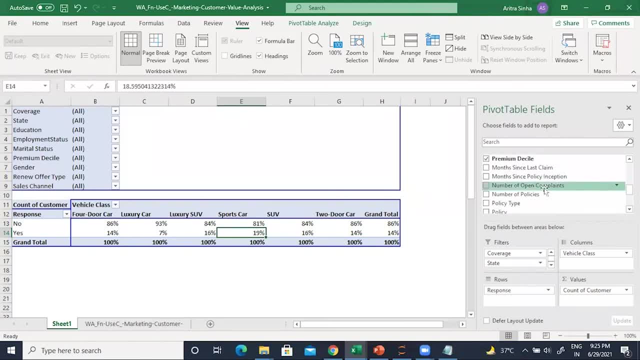 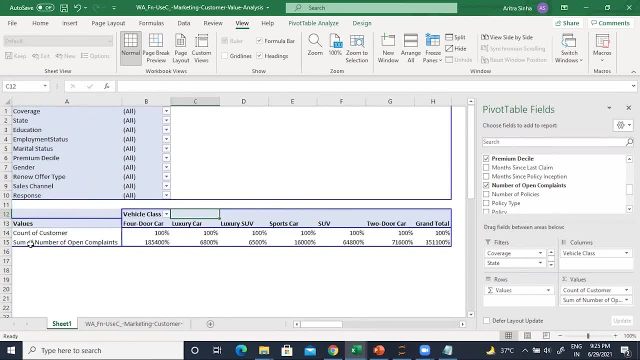 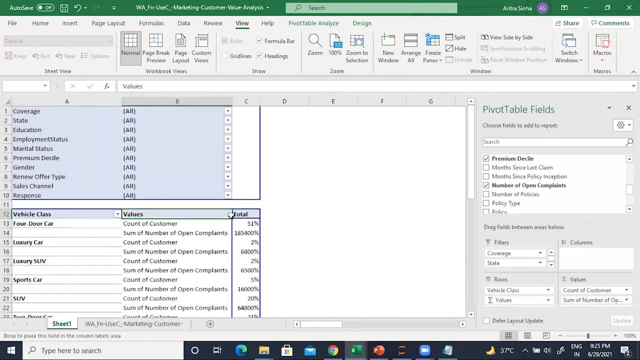 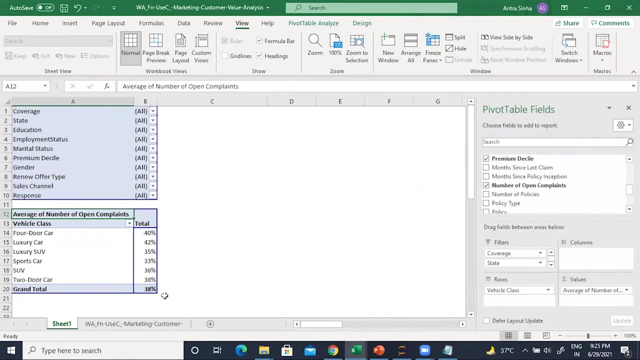 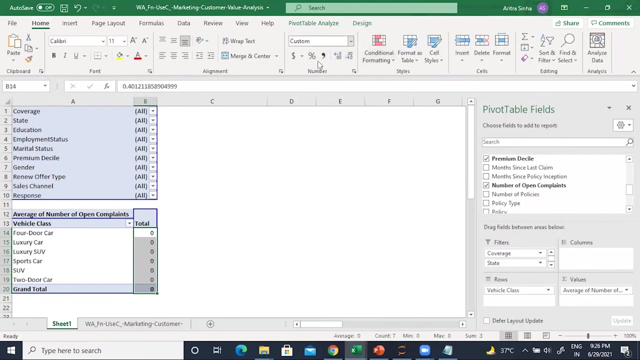 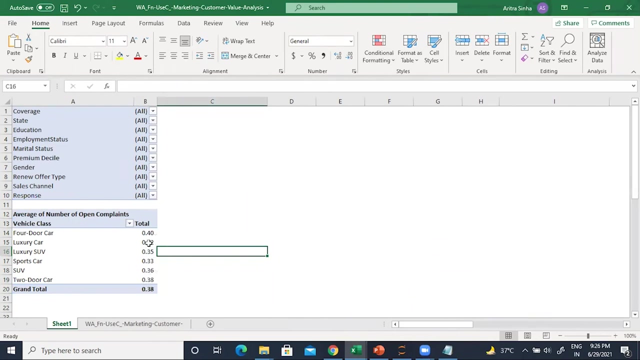 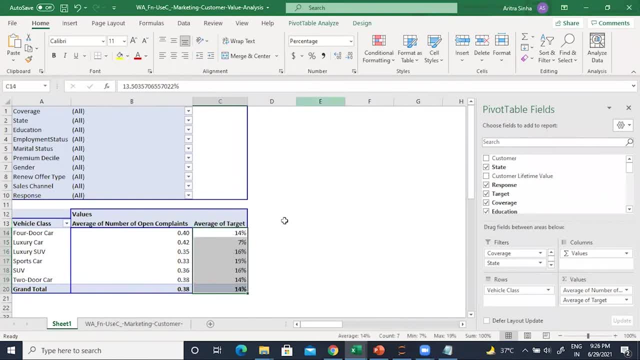 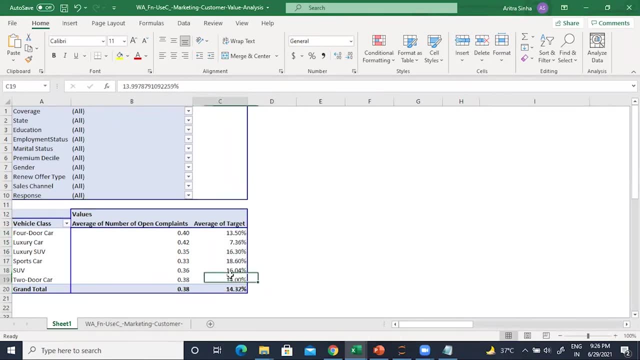 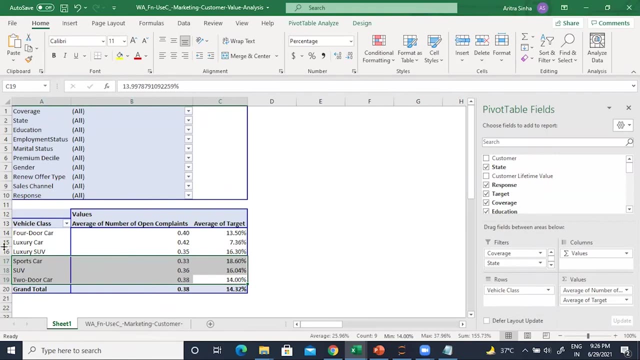 let's see the chance of success. chance of success marginally improves when complaints go down again. it is tying back to the same story that we saw that again. it is tying back to the same story that we saw that again. it is tying back to the same story that we saw, that if you're kind of happy as a customer, it. if you're kind of happy as a customer, it, if you're kind of happy as a customer, it makes sense what you do makes sense what you do makes sense what you do. so always try to make sure that your data, so always try to make sure that your data. 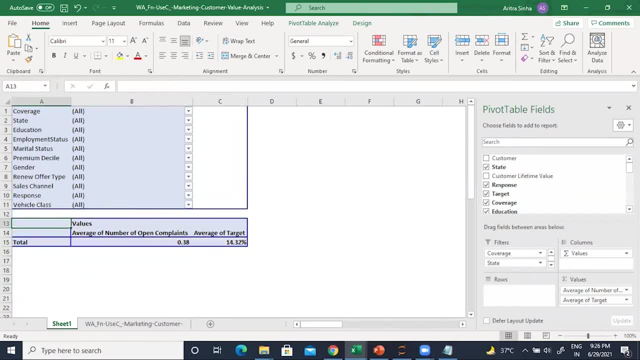 so always try to make sure that your data makes intuitive sense. okay, makes intuitive sense. okay, makes intuitive sense. okay, um, because in interviews or in any kind um because in interviews or in any kind um because in interviews or in any kind of project presentation, of project presentation. 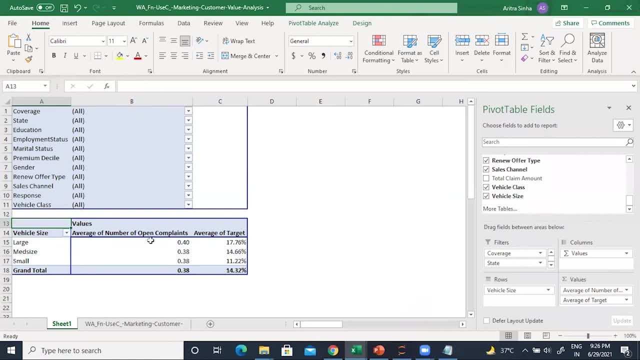 of project presentation. this actually helps to show that, yeah, i. this actually helps to show that, yeah, i. this actually helps to show that, yeah, i have checked on intuitive size as well, have checked on intuitive size as well, and in case of large class, more likely smaller cars- they are going to shopper insurance whoever. gives them the lowest premium, they will go with them, okay. total claim amount. is it going to change on an average? on an average, total claim amount is highest in case of smaller cars, and this is the most unprofitable part of the business where smaller cars are being insured. 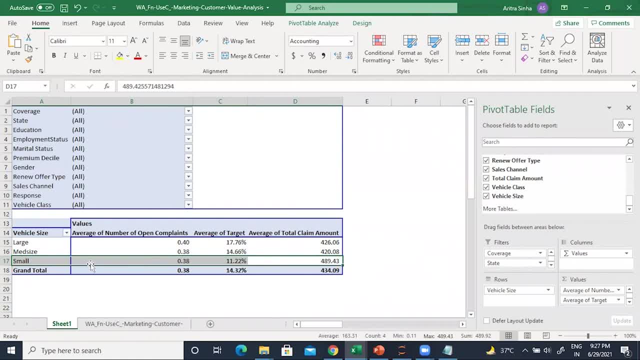 claim amounts are on an average or higher as compared to larger and mid-sized cars, but they are also not coming with good renewal rates. renewal rates is 11 as compared to the average of 14, so this is the most unprofitable part. however, this is the most profitable part, so larger cars. 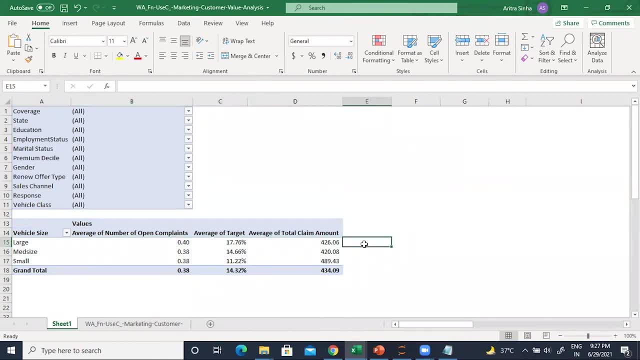 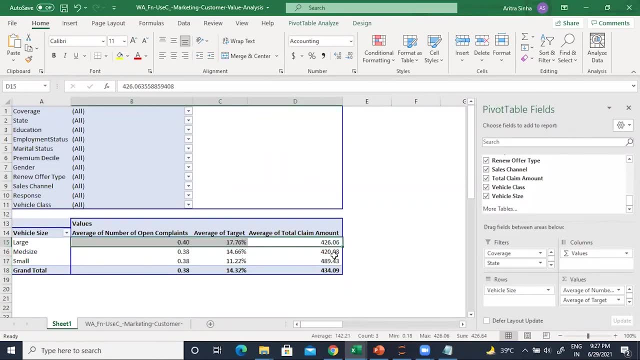 makes a lot of sense. you ask the insurance company to pay less money to you and also give them repeat business by doing renewal. so this is good for them, this is good and this one is not good. so again, if you are trying to create a strategy in python, we'll try to do it using um, i mean vehicle. 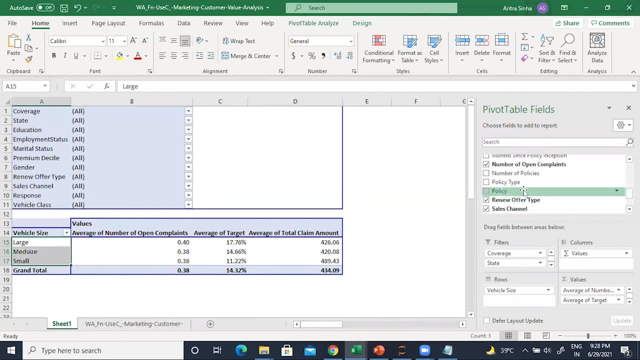 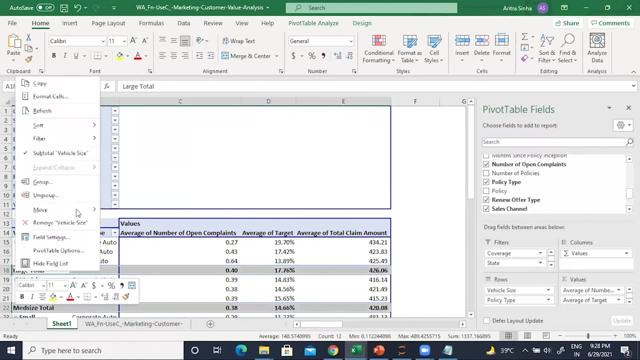 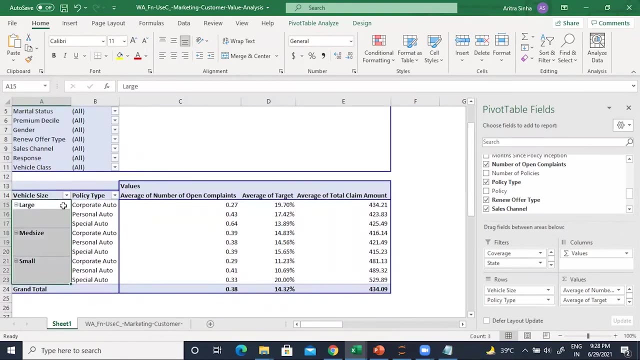 size can be a consideration for that. okay, what else did we miss? type of policies: all right, let's have a look. so in pivot table you can also drag uh variables like this and you could do an interaction analysis. see, in large cars we can see what kind of policies you have. the corporate auto is a policy type. 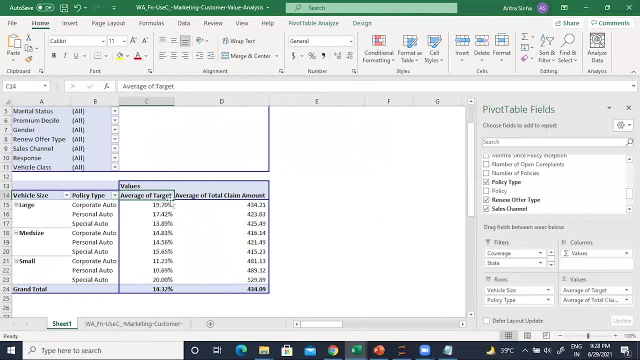 and, uh, let's get this. so 19 is the overall renewal rate with 434, so that is standing out as the most important. uh, this is the most profitable part of the business where you've got large vehicles under the policy type of corporate where renewal rate is quite high in case of small, small. 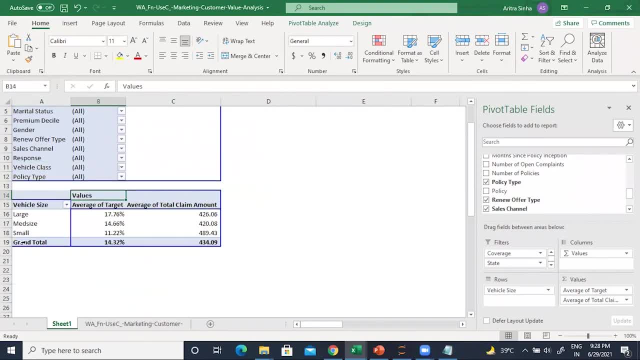 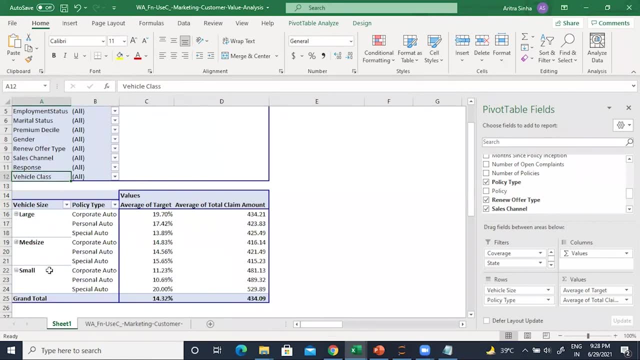 is overall bad if you look at. if i just take it away, right, small overall is bad, correct. but if i take a policy type, then within small special auto, whoever has taken special auto becomes good. i mean from a renewal perspective. renewal, at least terms of renewal, is quite high- 20, but also it's 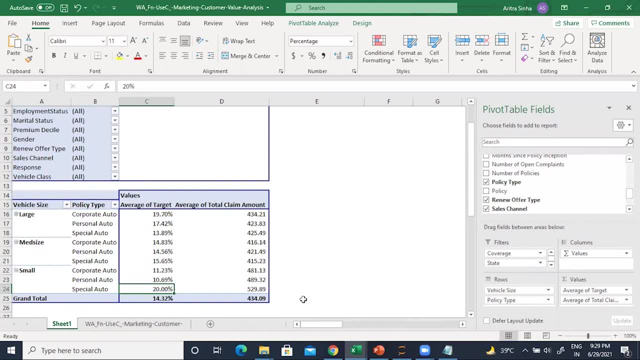 costly because they are going to charge, you know, and they are causing the majority of losses: 529 per customer. okay, so this is what we call as interaction: interaction between vehicle size and policy type. now, why would we want to use machine learning? because machine learning models can automatically identify these interactions, especially decision.